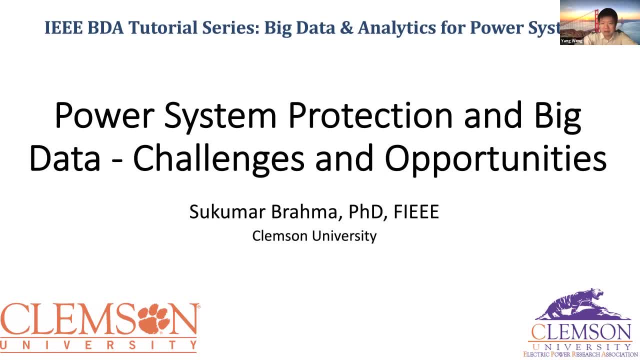 especially the ones who are connecting technology to data, to protection. We are very lucky today to have Professor Char, graphics director, and I grind John Brown to talk about his vision and his idea. Dr Charles Brahma received a Bachelor's in Advanced Media Science development at the University ofburn Zürich in the United States. at the University of 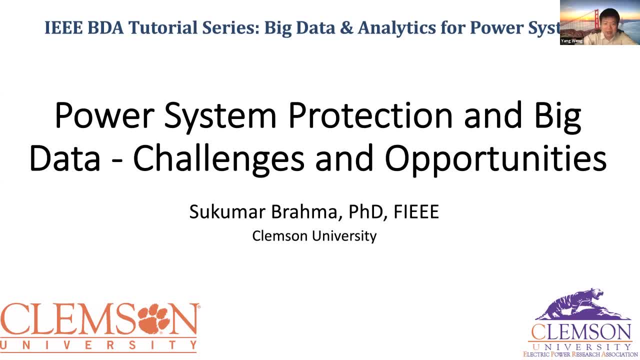 Beijing. For those who wish to learn more about who isその professor dares to spend the time in the talk. Professor Brahma University and a master degree from IIT Bombay. The PhD is from Clemson University. They are all from electrical engineering. So yeah, he also is with a title in Clemson University. 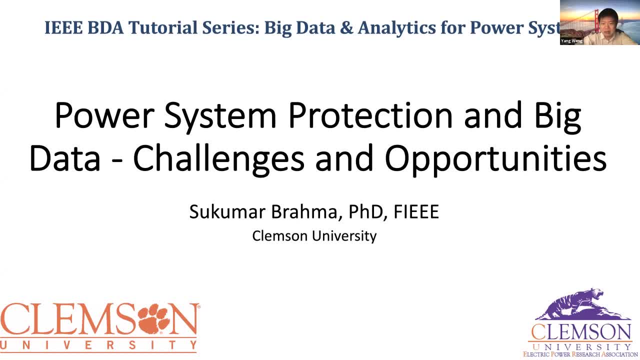 Media and Energy, Distinguished Professor in the Power Engineering and the Director of Clemson University Electrical Power Research Association. So yeah, if I pronounce correctly, this is Before joining Clemson. he was William Christine Indow's Chair Professor at New Mexico State University. He has chaired the HBPS Educational Committee, which has a great impact over here. 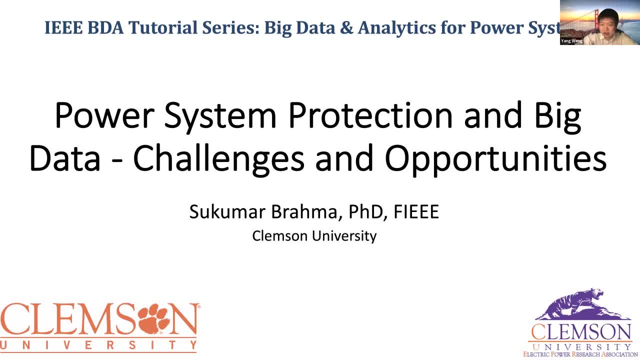 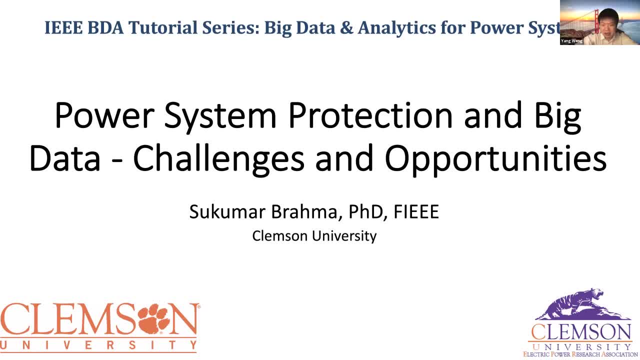 So, yeah, he's been a very good friend of mine. So, yeah, he's been a very good friend of mine. Yeah, we are formulated. He's a member of the PSRCC. He has been an editor and guest editor in. 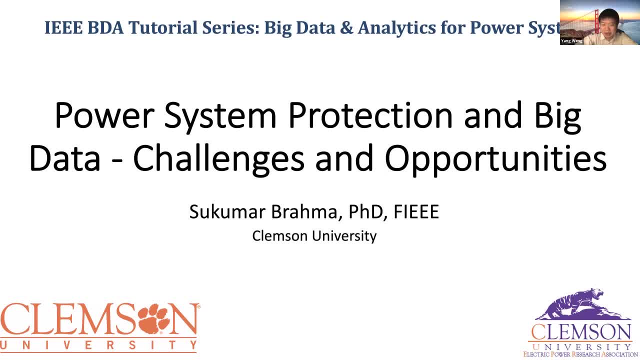 chief for IEEE transactions on power delivery. His research interests span across diversified areas of electrical engineering and computer science and to have cutting edge approaches to emerging problems like what we are talking in this webinar series. Finally, Dr Brahma is a distinguished lecturer and a fellow faculty and I look forward to this great talk today. 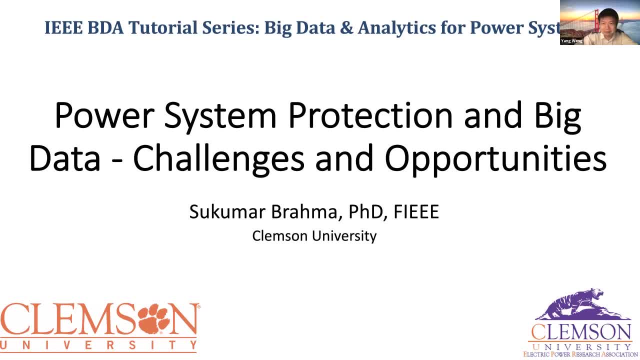 Professor Ibrahima, thank you, Thank you. Thank you, Yang, and welcome everyone to this talk. Well, hopefully we will have a good discussion. I think that's probably what is needed, because there is a lot of questions on both sides. The protection people are looking for, what they can. 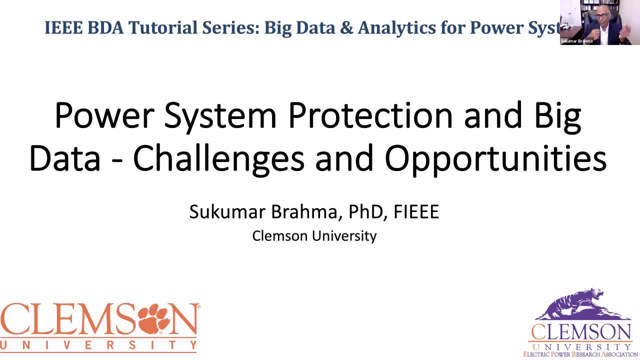 do to improve their system and the data analysis. people are always trying to get into other domains where they can make an impact. So if you want to start this, I will tell you a quick story. where about? I think it was about 2003 when I was I just graduated- done my work in protection. 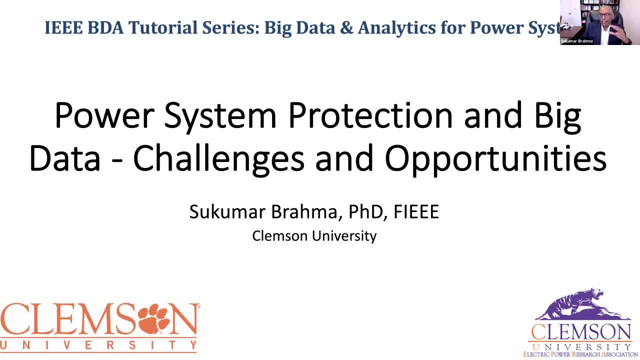 and started doing protection. A colleague of mine who works in data science and AI- even then he worked in that area- said: you know what, all these things that you're doing in the next 10, 15 years, that will be done by machine learning. And I said: well, we'll see. 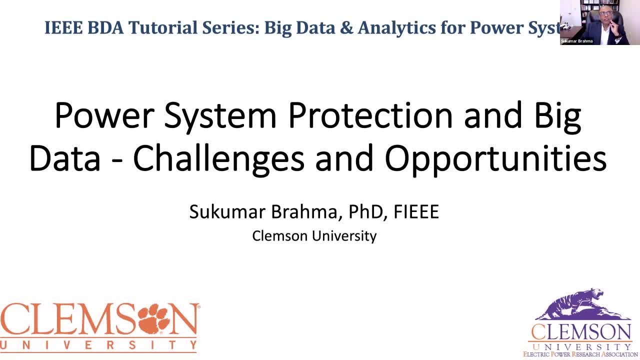 So now it's been what? almost 17, 18 years and there has not been a single relay that has a machine learning feature in it. And talking to quite a few industry people that I regularly interact with, they are not thinking a lot about that as of now At the same time. so that is the 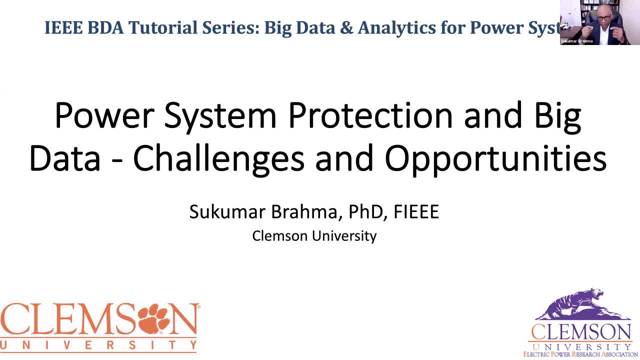 one side of the story. The second side of the story is that, as Yang mentioned, I go to the power system relaying committee meetings a lot and almost every meeting I attend, And recently there has been a working group on applications of AI in protection, So that is being chaired by. 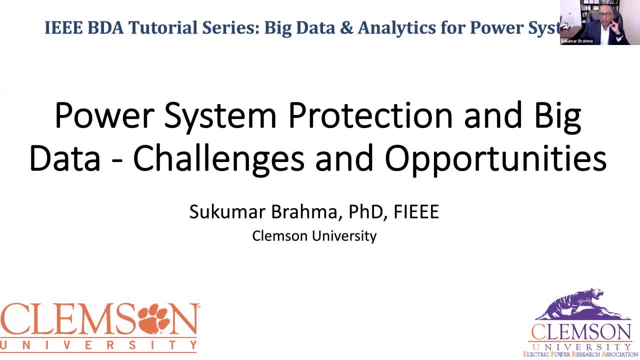 Dr Yi Hu and I'm a part of that, So it's not all bad People, as I said, have started looking at how we can use AI to do that. One of the projects that I'm working on from DOE with Sandia National Lab. 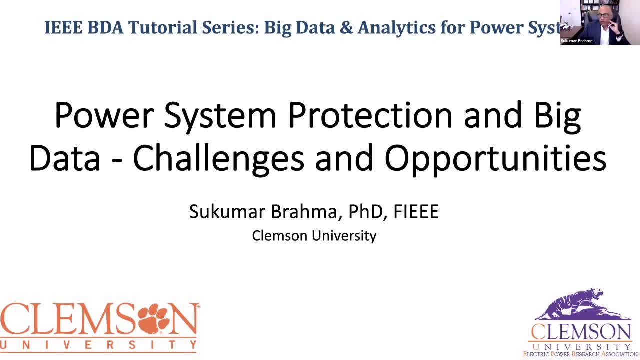 the Sandia National Lab folks are doing a lot of extensive application So they're trying to use machine learning for the protection applications where the legacy protection is. SANDEEP GURUVARAKRISHNANI is failing in the distribution systems and micro grids. 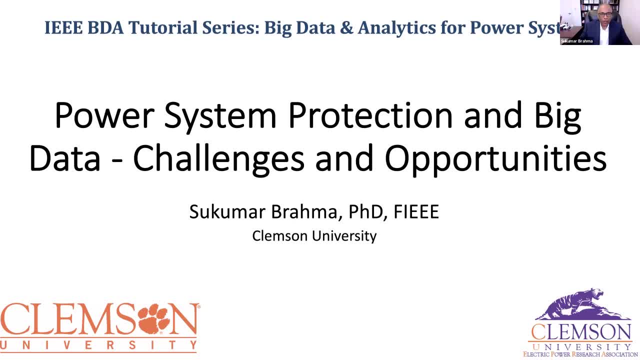 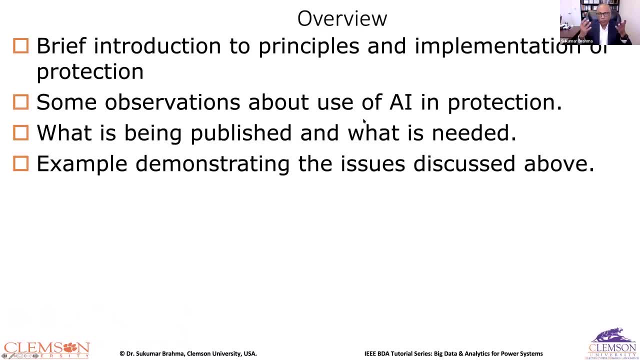 So this is. you know that. that's why this is. This is important that we look at. you know we basically need to look at what the protection is right. What protection is? It's been there for decades and decades. It's been fine tuned And, as it was mentioned, we graduated from. 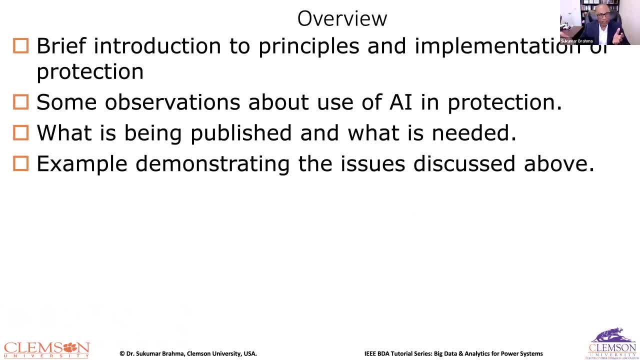 electromechanical relays to solid state relays, and now we all have numerical relays and we are. So what we'll do is, first we'll have an overview of protection. you know how it is done and what takes. what are the metrics for reliability, and so on and so forth. 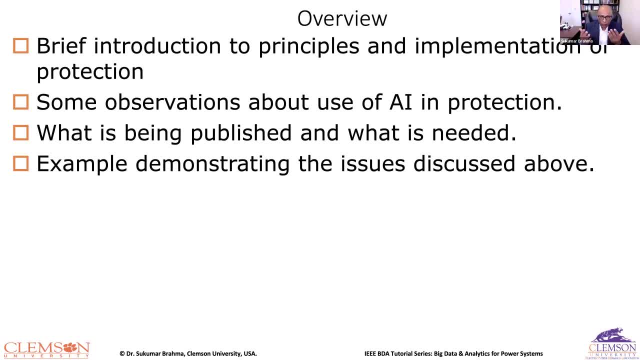 And then use of AI in protection, so where it can. so, basically, first I'll probably talk more about pitfalls, because I'm basing my observations on the papers that have been published until now on, you know, use of AI in protection. 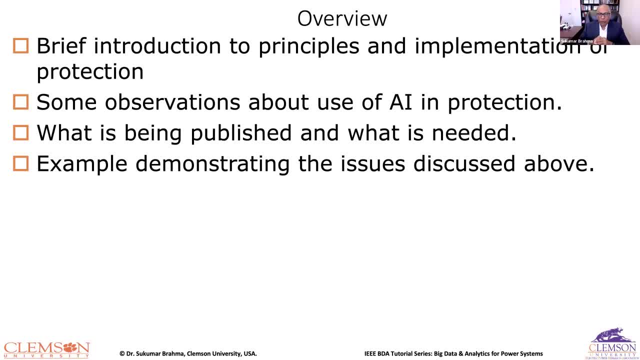 I've reviewed a few, So I'll talk about that. Based on that, I'll talk, I'll make some observations and then we'll see what actually should be the way to go forward, And then I'll so while I was at New Mexico State. 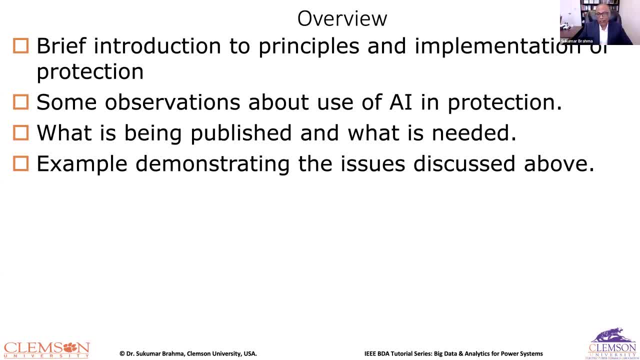 we discussed, we did actually end up using machine learning for about five years on an NSF project, And I'll talk about basically that project will display everything that I mentioned before. What are the challenges? How to you know how to get around that? 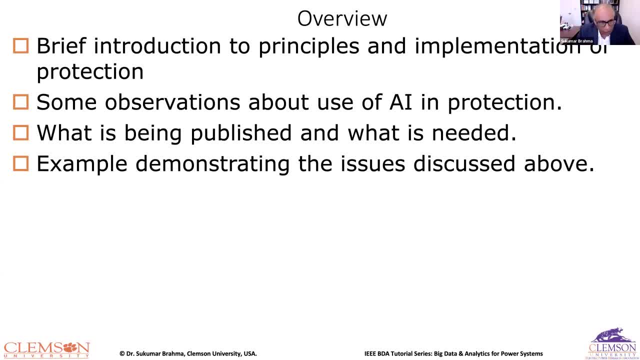 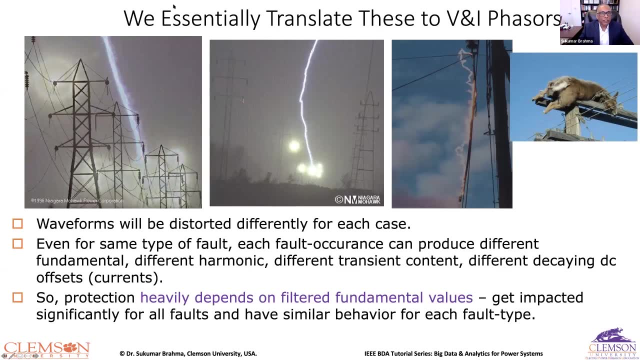 So that is the plan, And then, as I said, you know, questions and answers would probably be great at the end. So here is essentially what we do. okay, These are the events that you see. Let me. I think this will help me if I have a laser pointer. 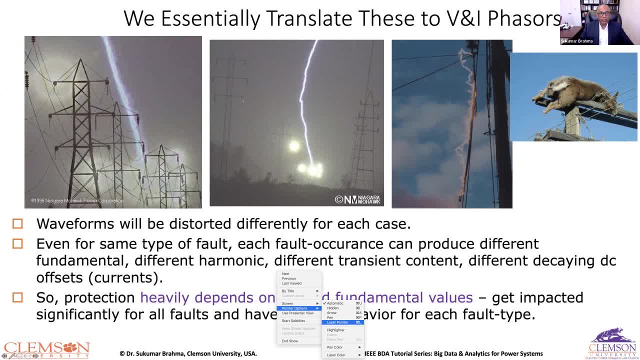 So these are the events: lightnings, flashovers, you know, woods, I mean the trees touching the water, Wires, some pretty, you know brave animals trying to rest on the wires. All these things we want to capture as a fault, right? 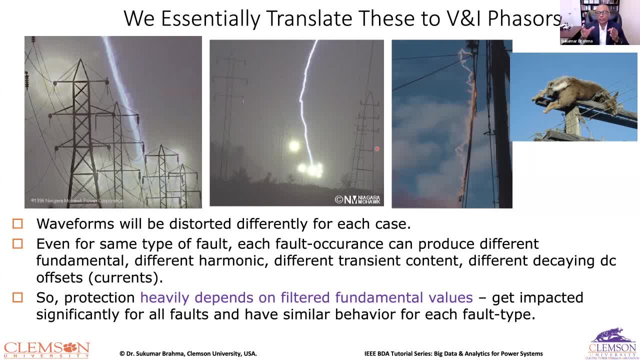 So, as you can imagine, all these events are so different than each other that they will give you different signatures. They're not giving you know, they're not going to look alike, So that is why. What are those? so what are the different things that we'll see? 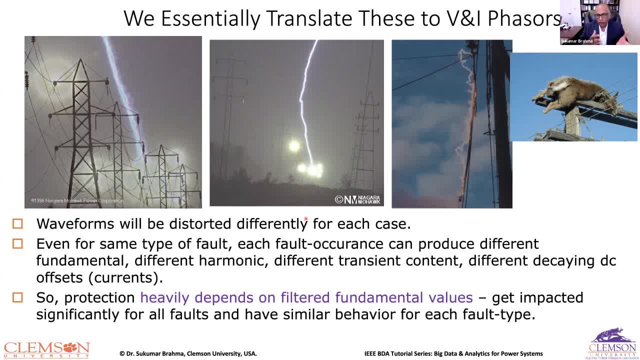 We'll see. you know the different forms of you. know the different forms of you. know these things, Um, when we're looking atwords or quedings. you know the two states. you know fingerprints like pictures. 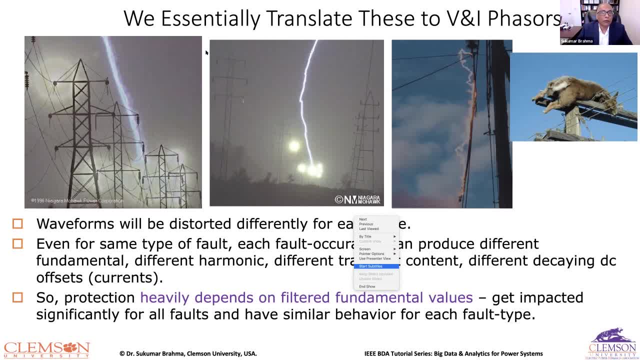 I think that is something that we're going to discover if we are returning to this only with the wherewithal, because it means it is something that is going toarse forever, And then this is very, very lucrative. We have a lot of technology that the local government, uh, also has to. emocòn VíASE. 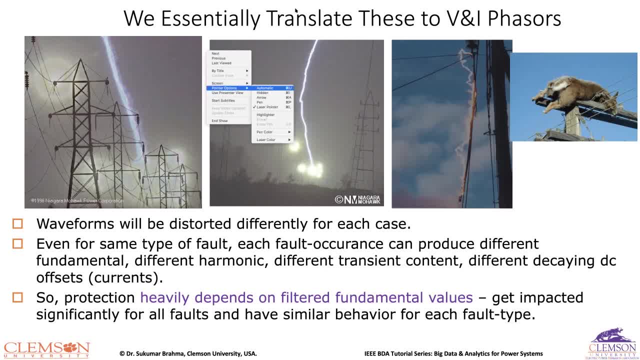 going to server. So if we have to deal directly Or meeting with the local government, It's very complicated, um brahama. so what i see is: i cannot hear you, chosa. can you hear? yeah, now, now. so i don't know. 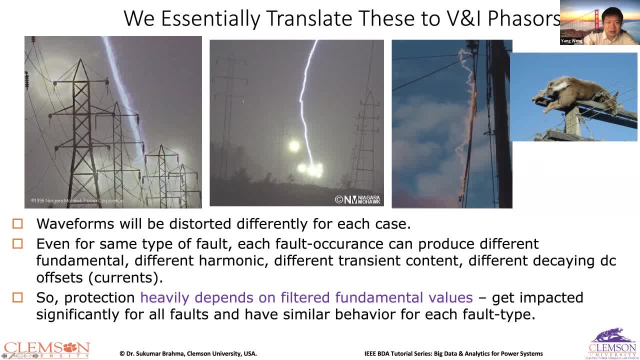 how i got muted? uh, okay, yeah. how long have i been muted? uh, no problem, 10, 10 minutes, not 10 minutes. okay, all right, so so i've not been talking to the ether for a long time, right, and the pictures are very meaningful, so we enjoy them, okay, cool. so, yeah, this is. i use these to get the students 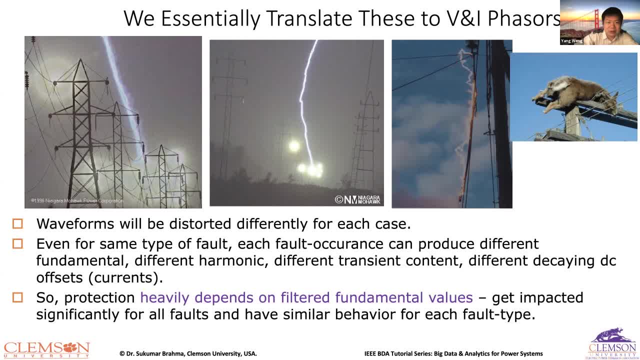 interested. uh, so these are some of my uh slides in the bosses of analysis course and when i do fault analysis. so just basically, you know, letting them know that there'll be very different signatures for different types of fall. but why we heavily depend on the phasers here are because 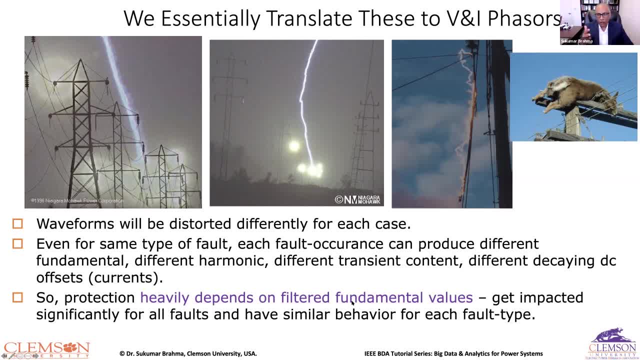 the phasers have some kind of consistency across all these different types of falls, not only the reason for the fall but the type of fall, line to line, line to line to line, line to ground. all these falls, the other, all these other elements that you see here, the harmonics, the transient, the decaying dc offset, all these vary. 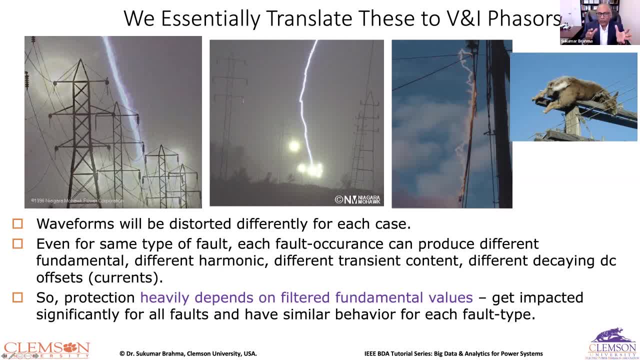 a lot and it is very hard to to use those signatures consistently for for detecting uh an isolating fault. but the, the fundamental values, the phasers of v and i have a more or less consistent uh behavior across all reasons of faults or types of faults. so this is basically. 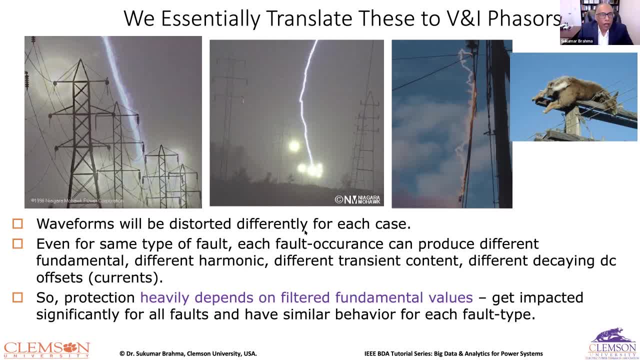 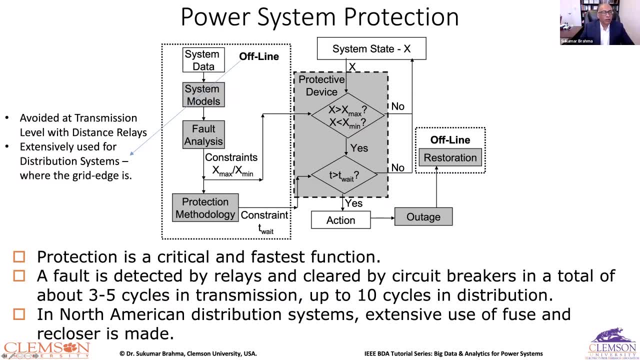 what we do now. uh, coming to the distribution system, because, as you know, you guys are all working on a lot on distribution systems and and grid edge in distribution system. this is what happens. so this is a protective device, okay, which constantly senses the state of the system. 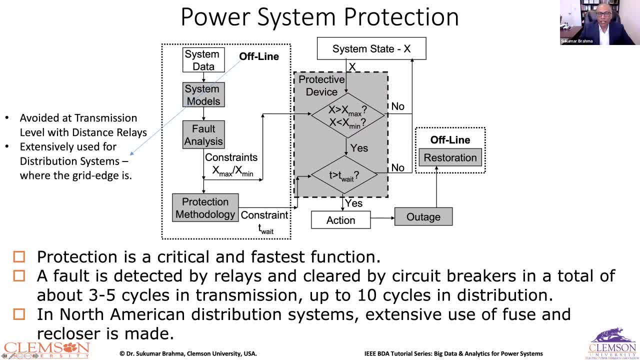 which is, in this case, is just voltage and current. okay, uh, they, it is converted to phasers. now we talk about numerical relay, so it's converted to phasers, and these are. it could be frequency as well. okay, so, and these are then compared with threshold values. uh, and if, uh, it is greater than a. 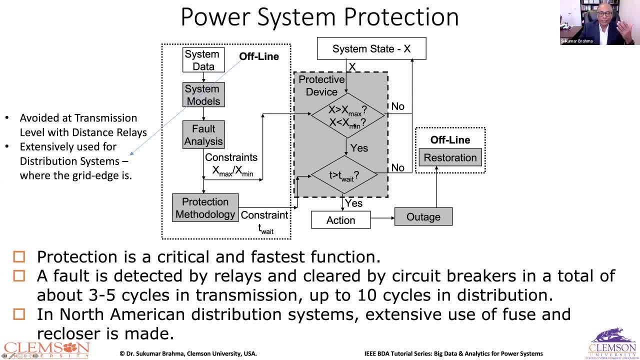 certain. so if current is greater than a certain value, voltage is less than a certain value, then it is declared that that's a fault. Now that x max or x min, these are the thresholds that we set, and we'll talk about that If there is. if it's not detected, it just goes on. 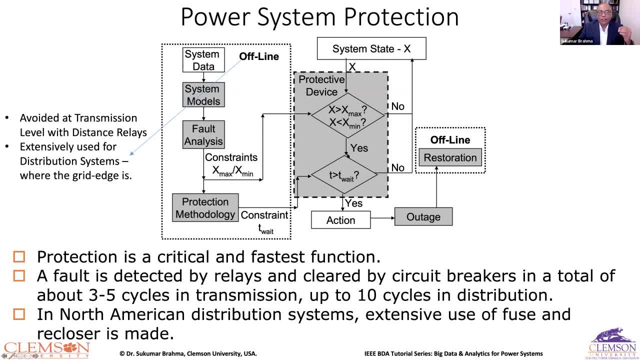 in the loop. Now, if it is detected, it needs sometimes to wait. depends whether that is a primary zone- that means this protection is in charge of its own zone, or is it backing up something else, right? So, based on that, there's a wait time, right? And then the action is taken. 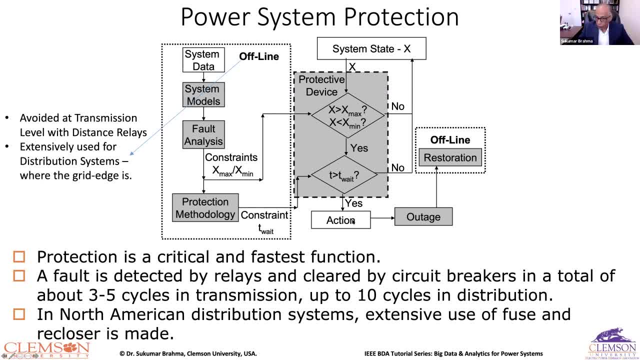 which means the relay operates, the breaker opens, so the fuse blows, and then there's an outage and a restoration. So this is all real online process. but these, how do you decide these thresholds? Well, the thresholds are decided for distribution systems. they're decided by 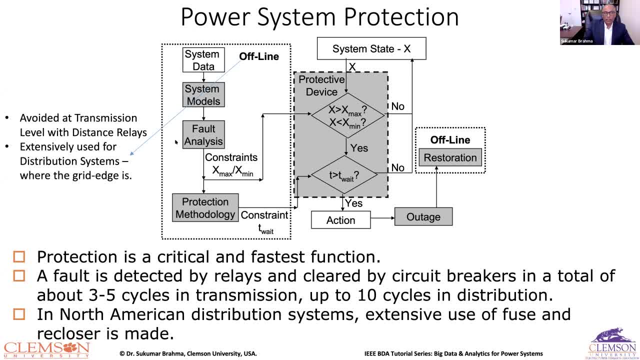 offline short circuit analysis, or fault analysis as we call it. where we have system data, we create models out of that many of you are familiar with. the most common model we use is a bus impedance matrix right And then you do fault analysis. that means you figure out. 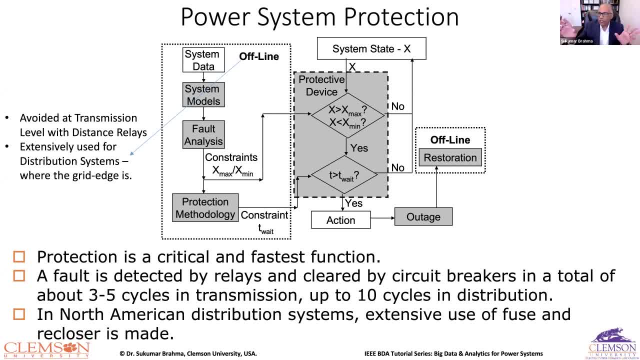 you know every type of fault at every bus in the distribution system. what is the fault current going to be? Based on that, you get an estimate of what constitutes fault and what doesn't constitute fault. So overload, for example, is not fault, but anything more than two times the rated current is a fault. something 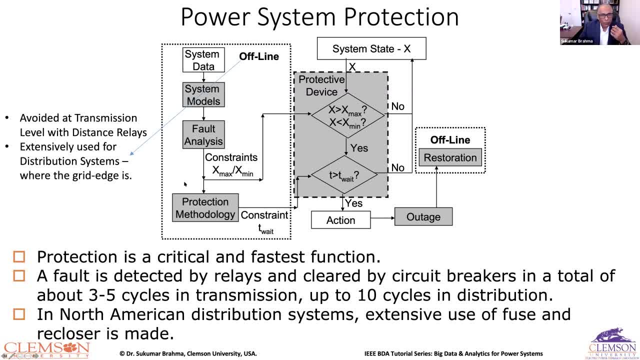 like that, And then the protection methodology, which is over current, under voltage frequency, depending on where you are implementing the protection. these are decided And then those are the. so also the wait time is decided from here and the thresholds are decided from here. 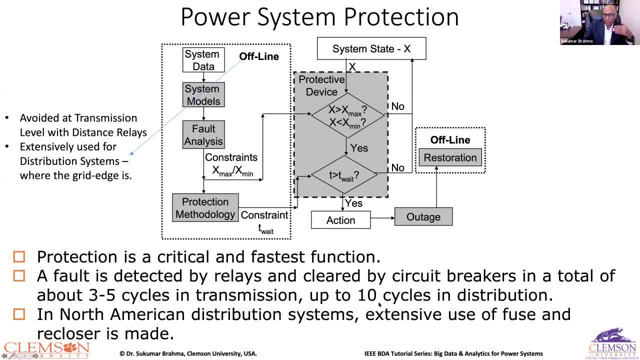 For distribution systems you have some more time because it's, you know, low voltage, but still about 10 cycles. up to 10 cycles- usually quicker- is okay. For transmission it's three to five cycles, because so here it is decided based on. 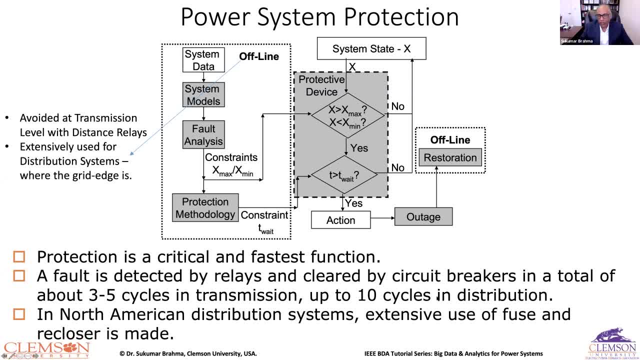 the stability of the system. here it is decided based on the actual damage to the equipment. Those are the criterias to select the time, allowable time for the fault to clear. okay, Now here's the thing: North American distribution systems we use extensively fuses and reclosers. 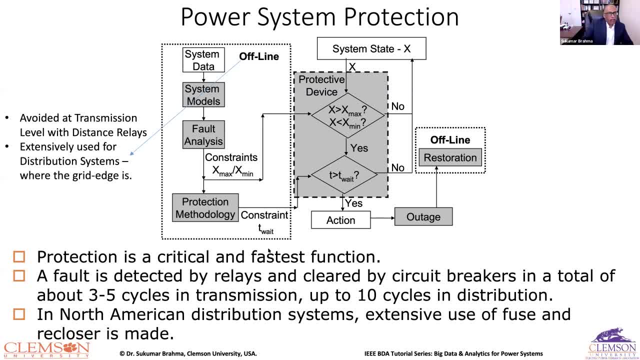 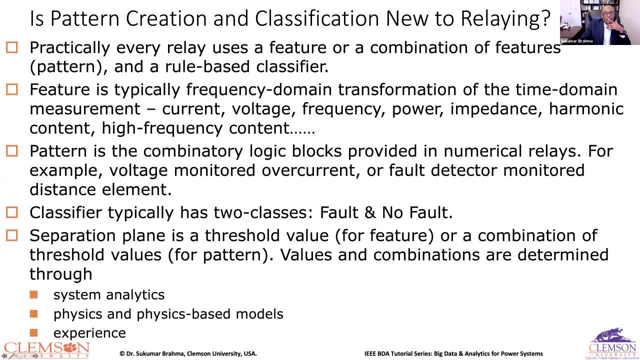 so, and we'll talk about that later. So I, just since we're talking pattern creation and you know classification, is it really new to us? Well, as we saw, the relay uses a feature or a combination of feature. 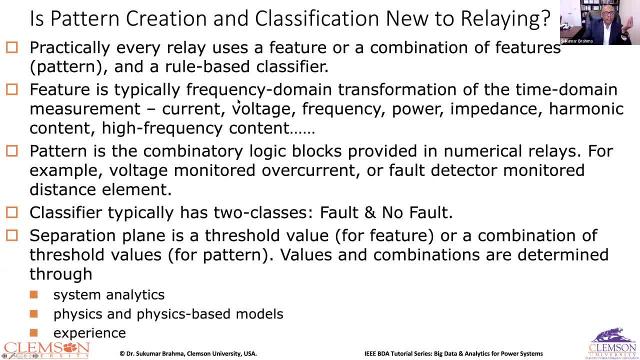 and a rule-based classifier. What are the features? It's typically a frequency domain transformation. okay, Because you measure time, domain, data, voltage and current, and then you get current voltage, frequency, power, impedence, harmonic content, you know, high frequency content. All this comes as a frequency transform. 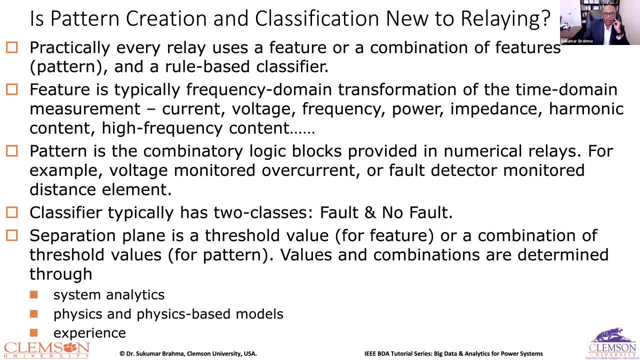 of the time domain data. So these are our features, and then our protection logic is based on a combination of features, which is a pattern, basically right, For example, voltage monitored over current or fault detector monitored over current For the bulk of connection and SLR data. 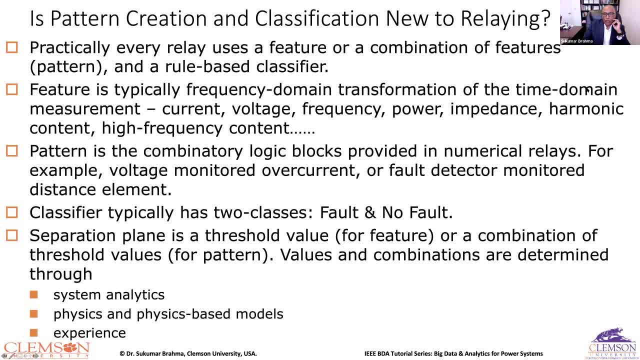 monitored distance. So that's a pattern, right. What is our classified? It has two classes: fault and no fault. right, And what is the separation plane? That is the threshold value that we talked about, right, And the threshold value based on system analytics, physics and 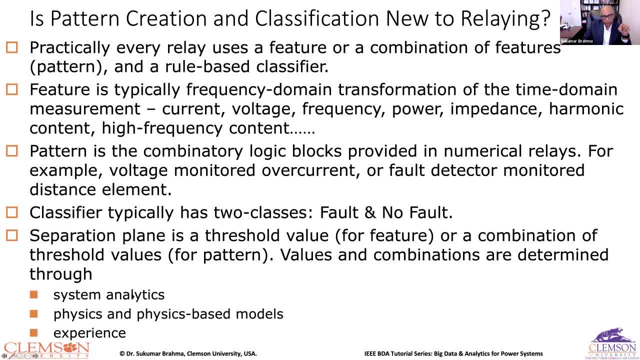 physics-based models, because those are the models that are used for system analytics and, most importantly, experience. So the protection engineers- one of the first books on protection is titled Art and Science of Protection. So the protection engineers, they're a little cocky. 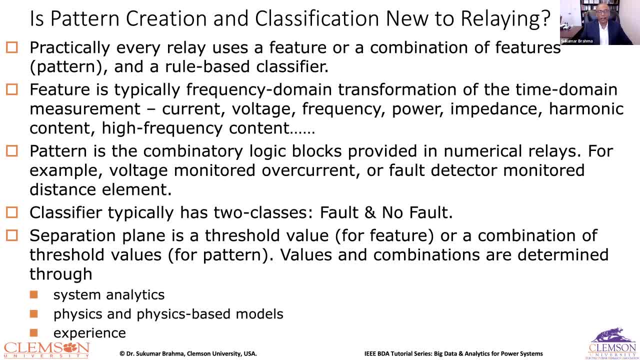 about it that they're just not scientists or engineers, They are artists also, because there's this experience that tunes everything they do. They don't apply the same method in the same way Across different circuits or different systems. So that's what it is. So it's there just to. 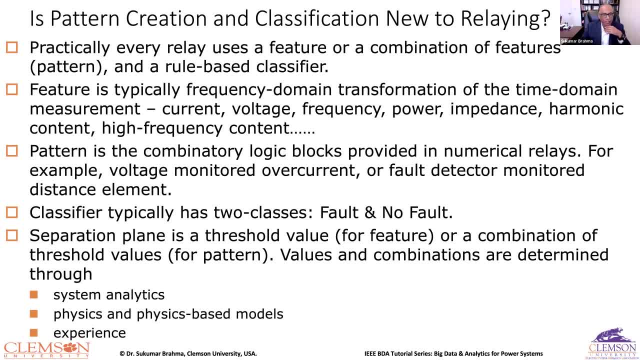 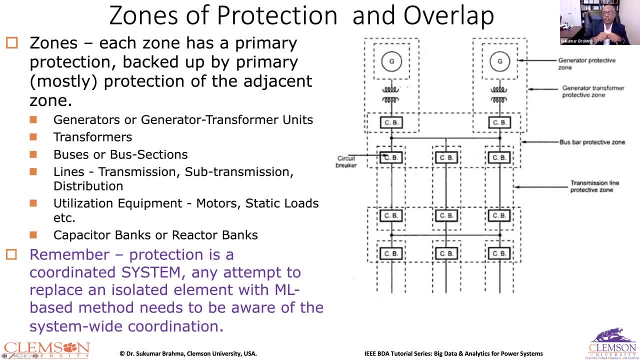 you know. so it's not new, It's just not learning based. And then you have zones. This is a humongous system, right? Every point in the system, every location, needs to be covered by some protection. So we have generators- we have you know. we have you know, we have you know, we. 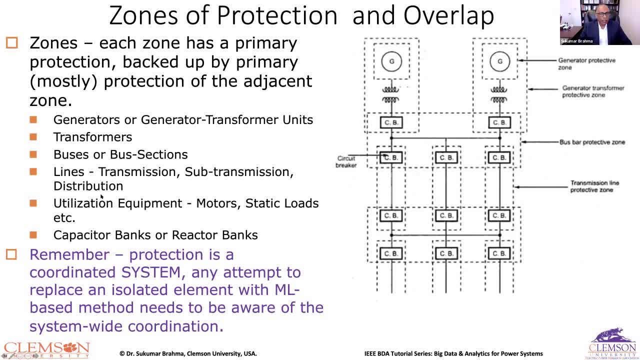 have bus bars, we have lines and then all other equipment: motors, loads, capacitor banks, reactor banks. they all have their own protection, which is considered the primary protection And, as you can see, the zones are actually overlapping. So that means that there is no. 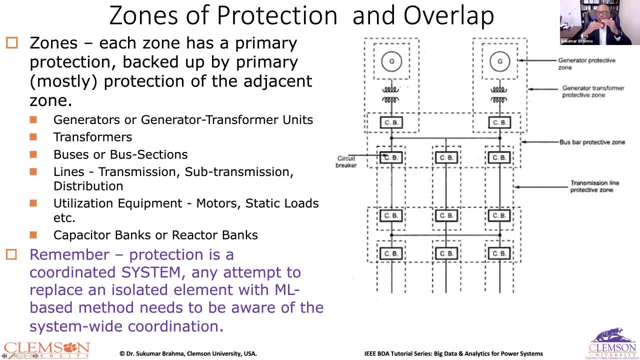 place in the system that is not protected. Yeah, In this, if there's a fault here, two protections will operate. but that's okay, Compared to nothing operating. So that's how it's done. Now, in each zone, each zone is protected. 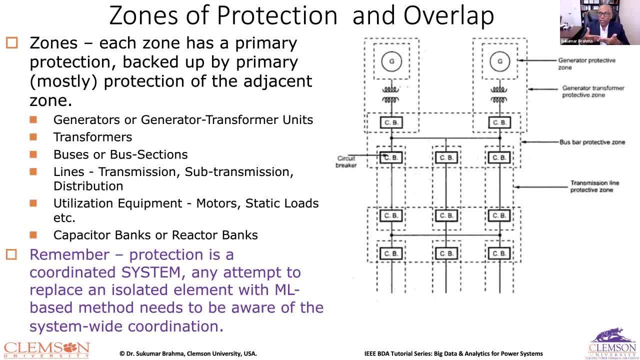 by its own protection primary and has always has a backup in case it doesn't operate. So this is what we need to understand. is that it's a coordinated system. Okay, If you and most of the papers start to do that, if you try to replace any 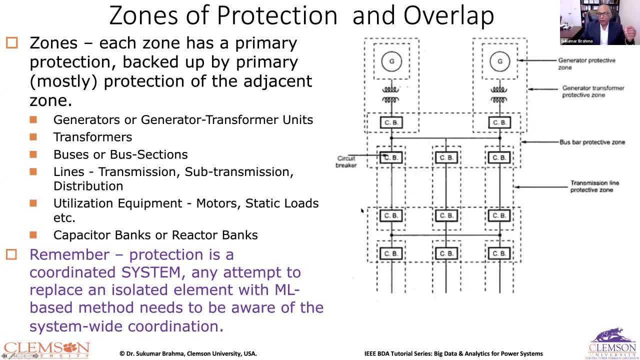 one isolated element or one zone with with AI based or machine learning based methods, you are not taking into consideration this whole coordinated protection system, And that's where you can run into problems. Okay, quickly, what is? what are the metrics for protection reliability? 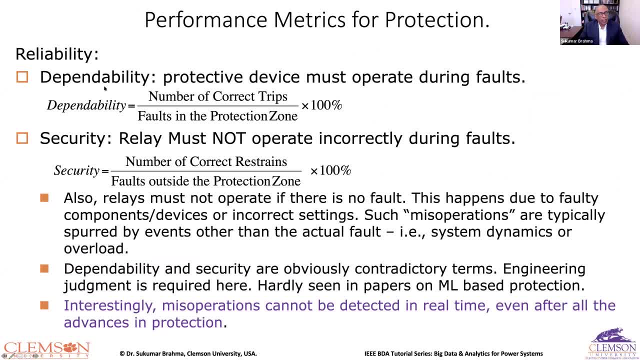 Well, reliability has two aspects. dependability, which means if there is a fault the device must operate, So number of correct trips divided by the faults in the system. Security, so there's another part of it. Okay, It should not operate incorrectly for fault. So if the fault is in the other zone. 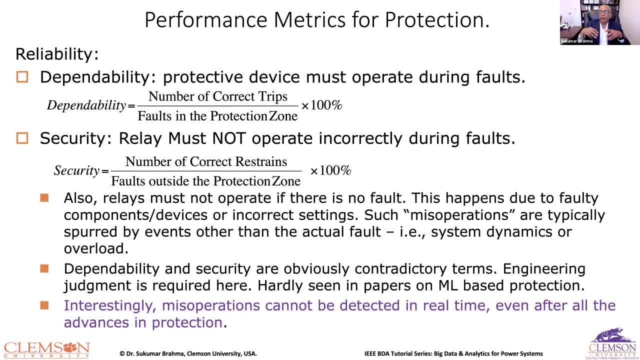 it should not operate. it should operate only for the faults in its own zone. Plus, if there is no fault, it should obviously not operate. Right, That's the security part of it, And if this happens, then it is called a misoperation. 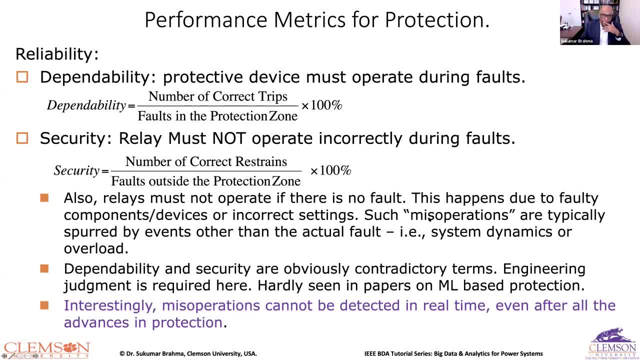 Okay, the misoperations are, and we'll talk more about misoperations, because these are, misoperations, are the only thing. after all these years of protection, Misoperations are the only events which still cannot be detected in real time. So if there is a fault, yeah, the system is going to. something is going to operate if it doesn't. 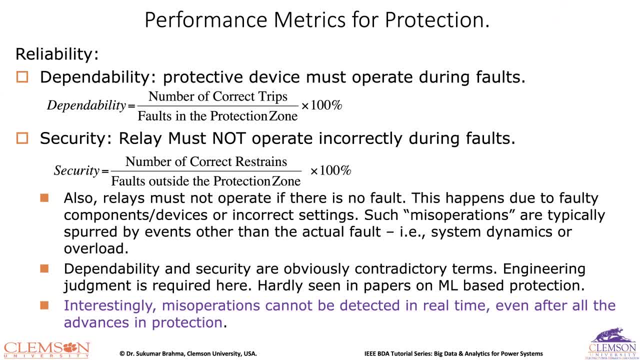 operate. something else is going to operate, that is really very, very well taken care of. But if it operates without any reason for incorrect settings, for example some problem with the relay itself, Virginia Tech guys in the 90s came up with something called a hidden form. 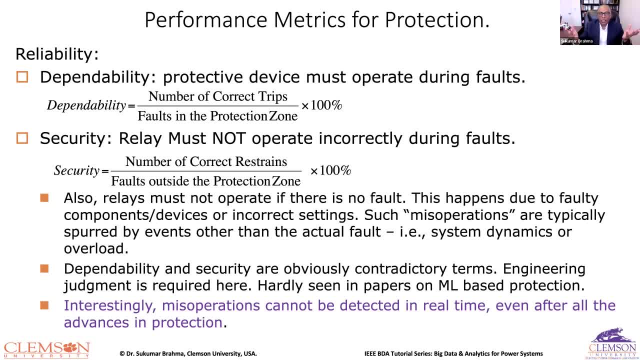 which you don't know, but suddenly it manifests itself. That is still. remember this. okay, this has still no protection. protecting system is able to detect misoperations. Okay, selectivity. So now look at how much redundancy is built in. So, for example, this is: 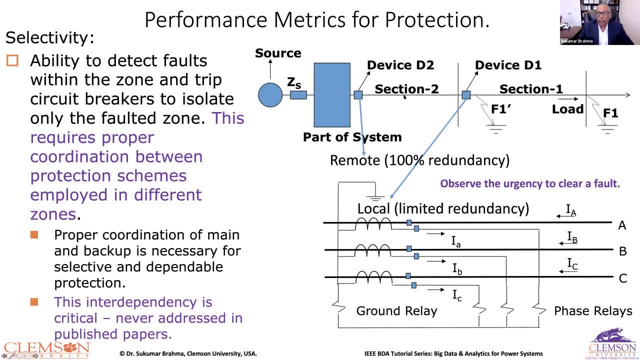 if you take a simplified distribution feeder, which is section 1 in section 2 here, right, and if there is a relay system, if it's fused, then it's just a fuse, but if it's a relay system you have phase A, phase B and phase C. 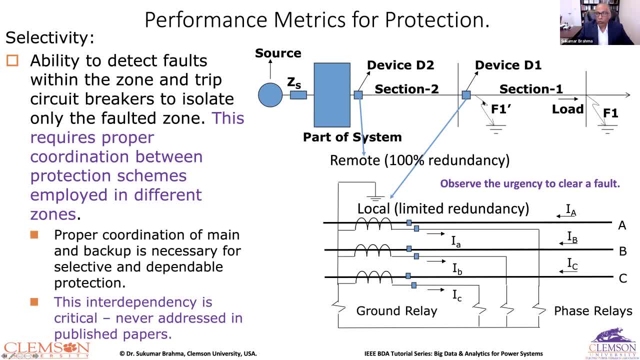 phase C relays and you have a ground relay, which is right here. So for any type of fault, say for example, take A to B fault- If it's A to B fault, there are at least two relays that will. 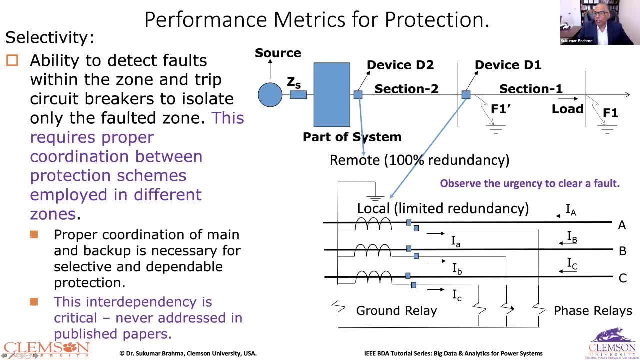 see and operate for that fault. So if one relay has a problem, the second still operates right. If it's a phase to ground, then phase relay and ground relay are the two relays that will operate. So there is a redundancy built in right here at the local level. Now suppose 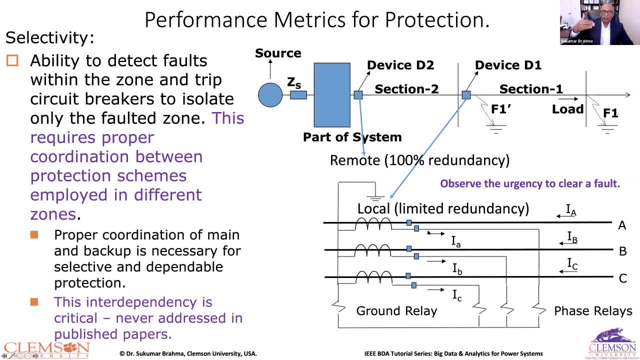 in this case the relay would trip the breaker. Suppose the breaker doesn't, or suppose the current transfer and the voltage transfer or something wrong with them and this scheme fails, then this fault is also seen by this relay here. okay, And that's why the waiting time, if it. 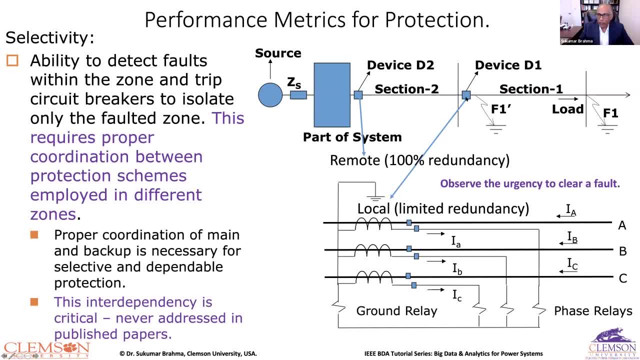 waits for this device to operate. if it doesn't operate, this will operate. Now, here is a 100% redundancy right: Different relays, different CTs, different VTs, different breakers. So that is why. so just observe the urgency to clear the fault. This is how it has been set And that is. 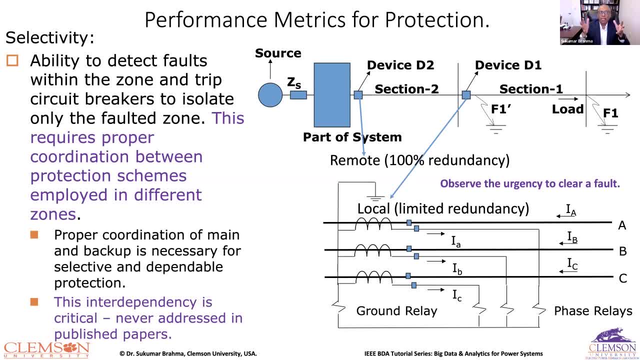 why. you know, it's very, very unlikely that a fault will just go on and on and something is going to happen. So this interdependency again is critical. okay, And if most of the papers that I see will do something here but then say, okay, I am doing better than the legacy scheme for here, but what? 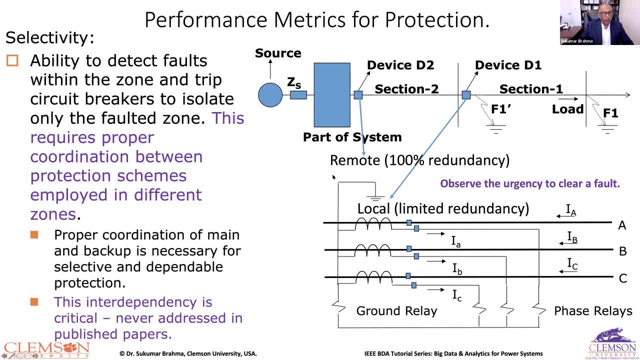 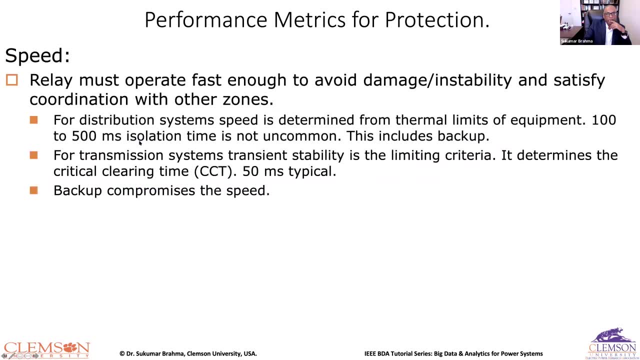 about backup. There's no backup there, So that is something that I consistently see in the papers that are published on this topic. Speed: of course speed is important And, as I said, 100 to 500 millisecond for distribution system is not uncommon. 50 millisecond is. 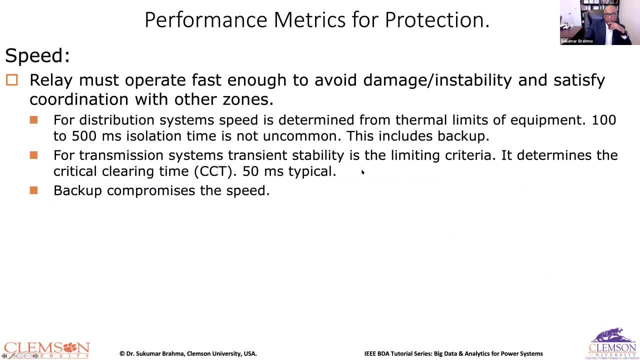 typical for transmission, because transmission is. it's based on critical clearing time, which is stability, dictated Here, it's dictated by the damage curve of the equipment, And then backup obviously compromises the speed. So these are the metrics for evaluating how good or bad your protection scheme is. This is our distribution system: Most parts of the US. 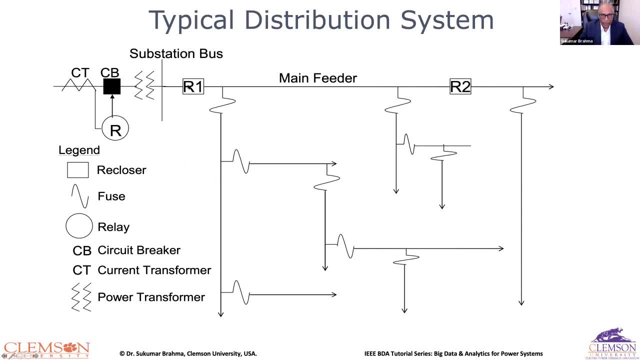 has fuses and reclosers. okay, The fuses coordinate with each other and then the fuse coordinates with the recloser. So this is because it's cheap and simple to implement and because of that, all distribution systems until now were fed by just one source, which is substation. 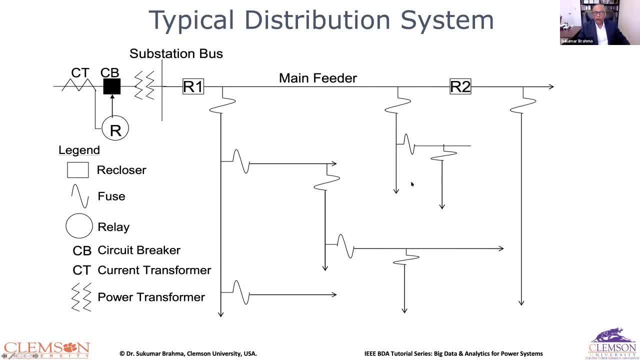 source. So any fault that happens here, right anywhere in the system, is going to have a fault, current flowing only in one direction. So that is the whole the assumption. and the system is radial. There are no loops involved. So these are the assumption on which all protection systems 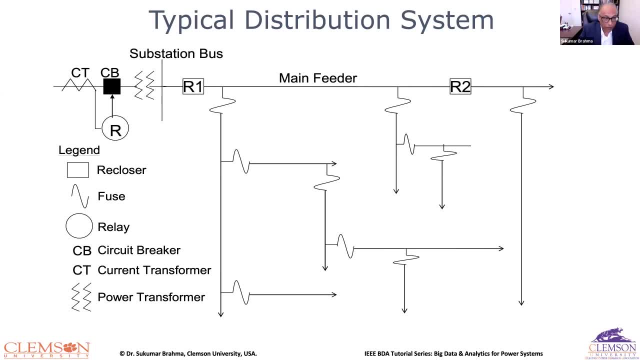 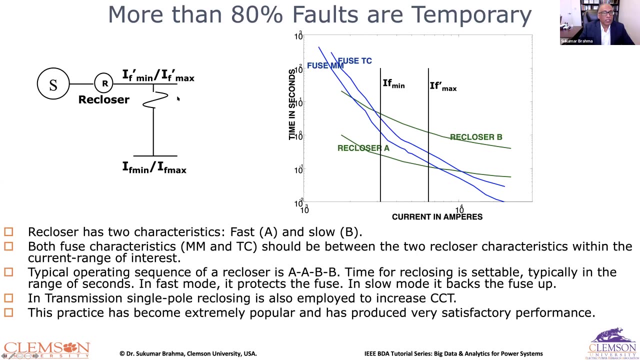 were built in the US and still are built, And that, of course, as you know, is changing, And we'll talk a little bit about that. And then again, what is the fuse and the recloser? Well, what happens is about 80%, or 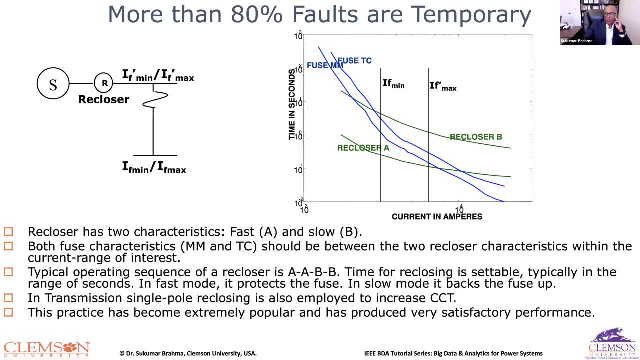 more faults are temporary. This is one another aspect that I've never seen the machine learning based methods address that. what happens if the fault is temporary? So if more than 80% of the faults are temporary, do you want to really blow the fuse or operate? 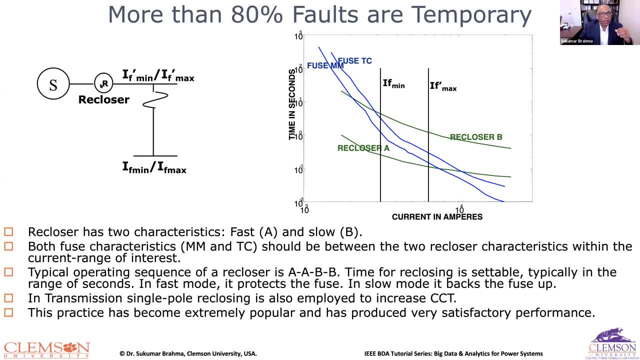 a relay? Obviously not, And that is why it is overseen by a recloser, right If there is a fault here, the recloser. if you look at this curve here, this is the time and this is the operating curve. The recloser has two operating curves, A and B, and the fuse has two curves minimum. 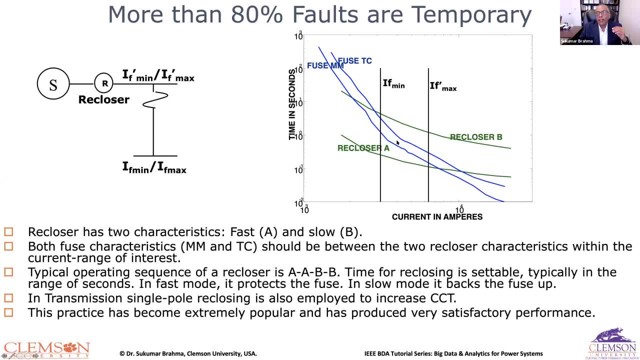 melting and total clearing. Let's not get into a lot of that. That's the fuse and those are the green ones are the recloser. So if you look at this curve here, this is the time and this is the recloser. So any fault that happens which would be between these two values, we know that because 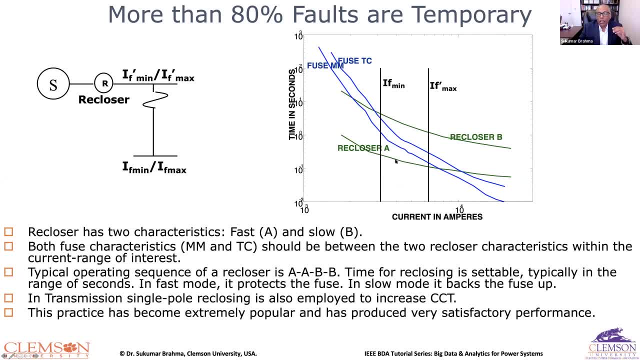 we've done short circuit analysis. recloser operates first, So recloser operates, So the fault here is isolated. then it waits and then it comes back and closes back again. If it closes back again, the fault is gone, You're good. If not, then depending sometimes on two fast operation. 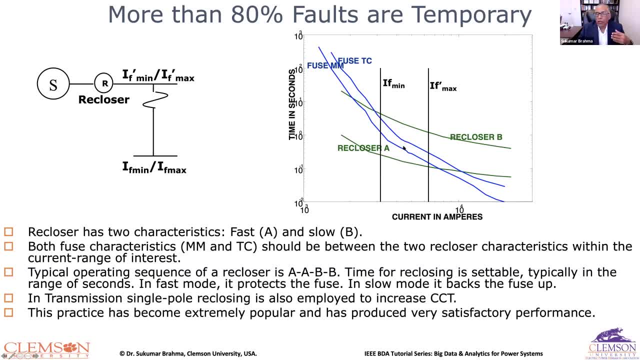 where it allows the fuse to blow. That means this scheme makes sure that the fault is permanent before the fuse is allowed to blow. This aspect, so recognizing whether the fault is permanent or temporary- is an important function. So if you can do that with some machine learning mechanism, 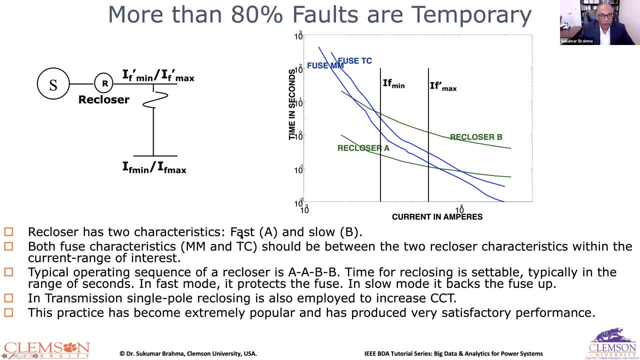 that'd be a great contribution, Because in this case, what happens is we still we're waiting. So that is something that and again, no, I have not seen papers that actually address this. There is also in transmission line, there is single pole reclosing which is employed, And there 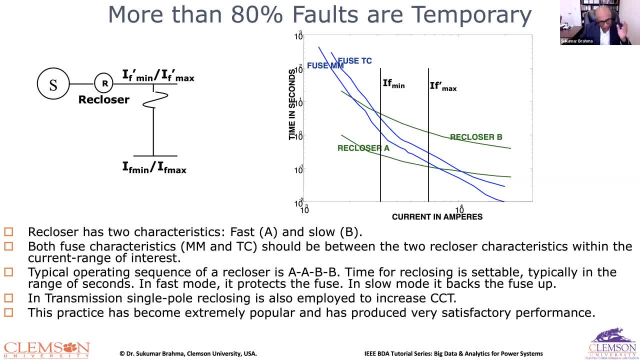 there is a, So I'm. I probably shouldn't go into that due to the time constraints, but there is a. there's a problem of secondary arc And before you close, reclose, you need to figure out whether the secondary arc. 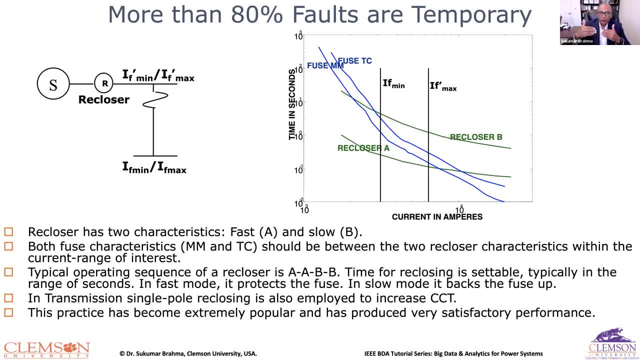 is extinguished or not, The secondary arc is created because of the capacities between the lines. Even when the recloser is open, there is a secondary arc going on. So, and then again, detection of secondary arc is a great application for for machine learning-based. 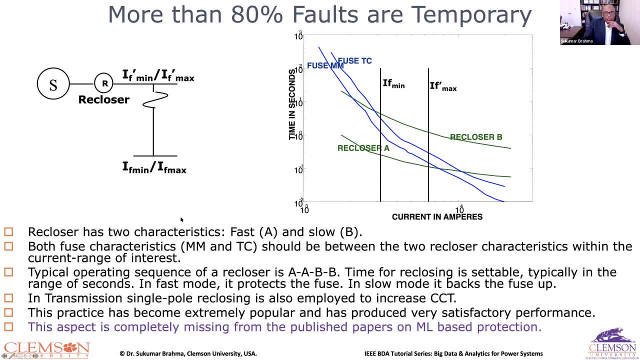 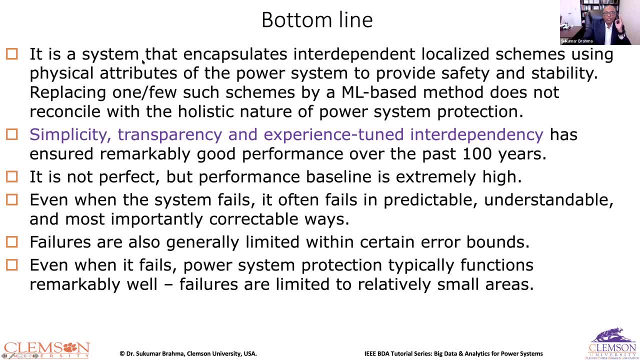 methods. Okay. So what's the bottom line? Bottom line is this: okay, It is. it's a system, it's not one device. It's a system of devices which encapsulates the interdependent localized schemes, uses physical attributes of the power system to provide safety. 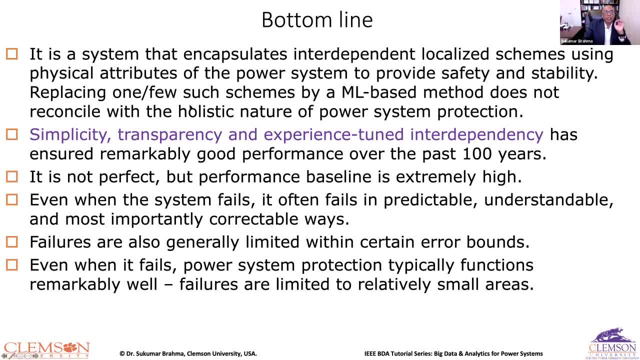 and stability right. Replacing one or few elements ah will not reconcile with this holistic nature of the system. protection Most every protection engineer- looks for transparency. He or she has to know what's going on. If you give them a black box, they will be very uncomfortable because you're talking. 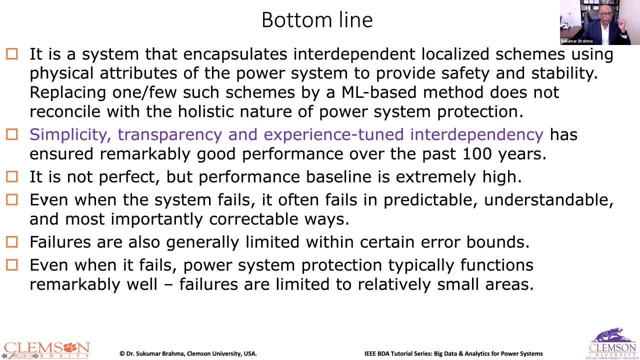 of protecting very expensive equipment. Also, it's not perfect. obviously we know that it's not perfect, but its performance baseline is really high. As I said before, even if system fails, it fails in predictable and understandable and, most importantly, correctable ways. 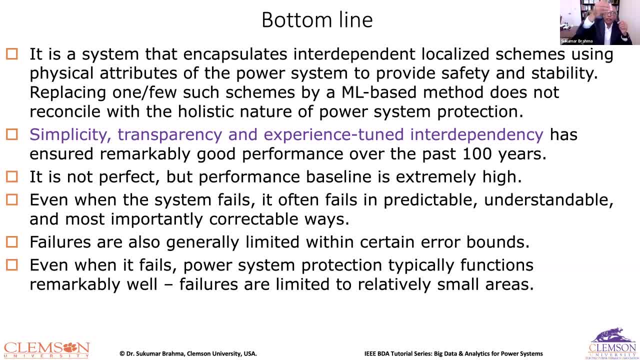 You can predict if this doesn't happen. this has to happen, and if a series of operations happen, you know why they happen the way they happen. You can, in postmortem, you can figure out. okay, this didn't operate. there was a problem. 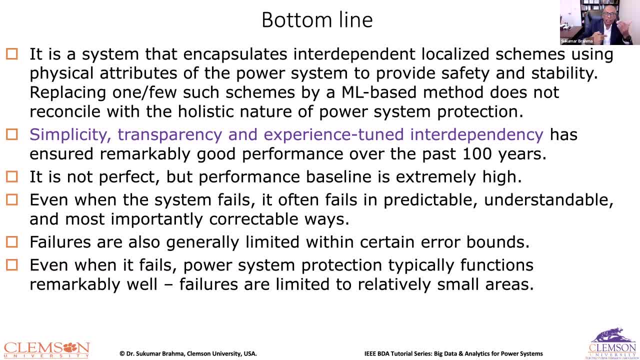 here. that is why we had this. That means you can correct it. That's why transparency is essential for protection. people right And again, failures are generally limited within certain error bounds. If you have say, you guys are in Tempe, so you will never have a fault on a distribution. 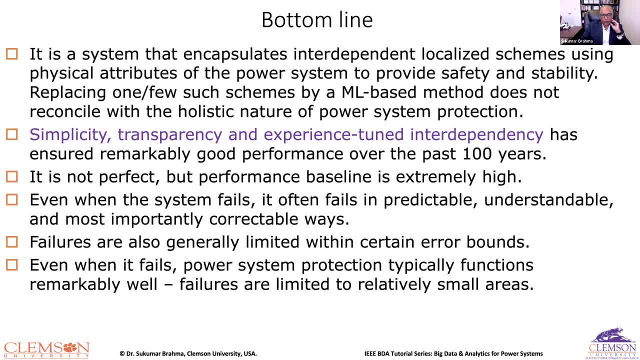 feeder That would take out, you know, the entire substation, is very, very, very unlikely. So the damage or the outage is usually, in almost all cases, limited to relatively smaller areas. So this is where we are. so, and you know, we live here, we've lived here for years. 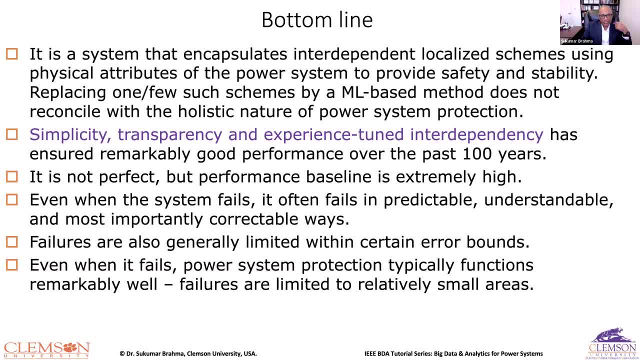 Just imagine how many times we've lost power, considering that all of our lines are overhead And exposed to weather, exposed to storms. right, Considering that, I think they're doing pretty well. Okay, so now let's look at what the papers do. 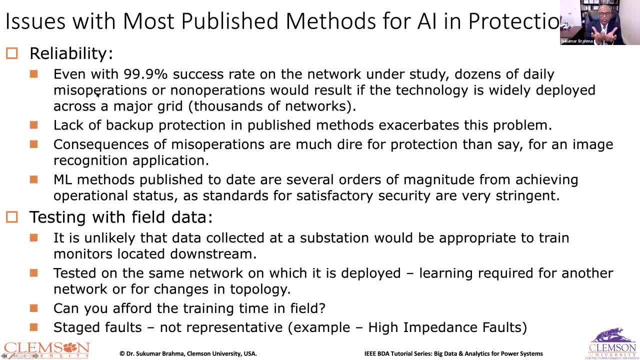 So I've seen papers that said that again, that takes just one scheme and then take their, you know, do their testing, do their training, do their testing. It says 99.9%, Okay, 99.9%- success rate of that one experiment that they perform. 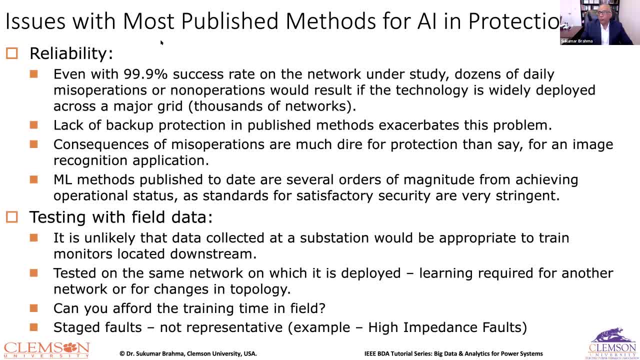 What you don't realize is if this scheme, suppose the utilities adopt this scheme and they use that scheme in thousands of networks, what is going to happen is there'll be daily dozens of non-operations in that system, even with 99.9%. 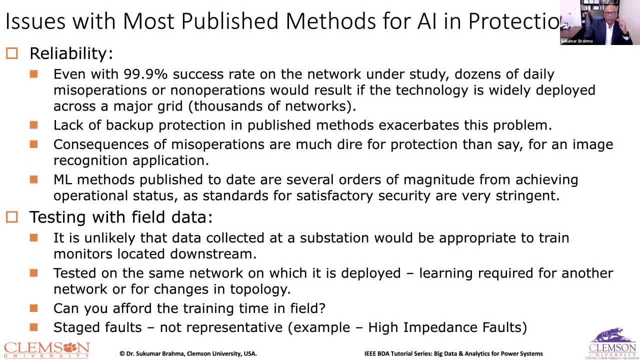 Okay, Whoa So, but is deceptive If it is employed in a very large scale, right? And of course, the lack of back up protection I already mentioned. the consequences are dire. So you know, because if it doesn't operate, it's non-operation means something is going. 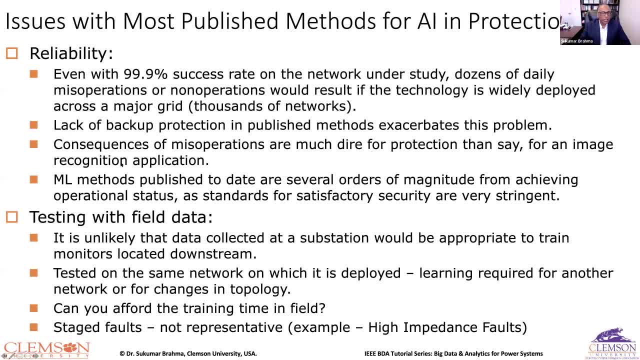 to blow up right, As opposed to say: image recognition- Well, Yeah, taking place. if you catch the wrong guy, you can, you know, finally say okay, my bad, and release that person, But in this case so. but of course, if image recognition is going on in drone, when 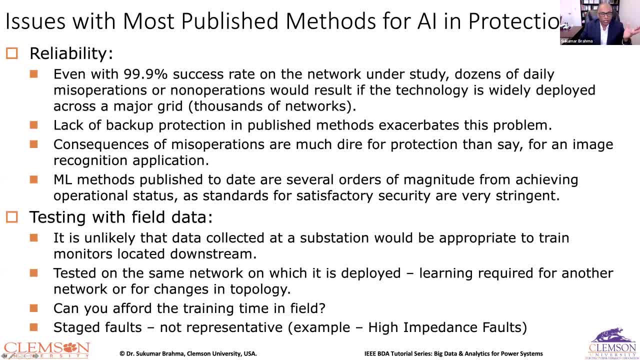 it's attacking some enemy territory, then it's, it becomes very important. But in protection there is no such case as okay, we can deal, we can live with that. It's always going to create, you know, either fire and then damage, and a lot of outage cost everything. So that is why 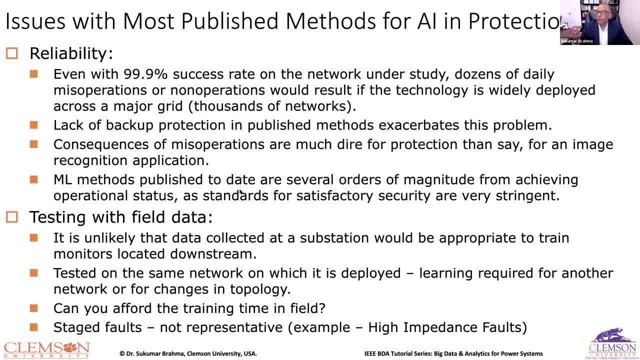 understand that, because I've seen this. when I talk to people, they say that the protection people are very conservative. They are. they are, you know, not ready to work with us, but understand where they are coming from. This is why they are conservative, Okay. 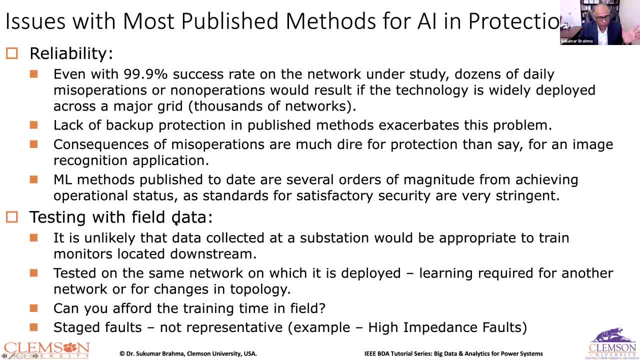 Okay, So testing of course. suppose you have field data, we'll see if you have field data on. suppose you have field data, If you have field data that you collect at a substation, would it be the? would it be useful if you are trying to train some monitor? 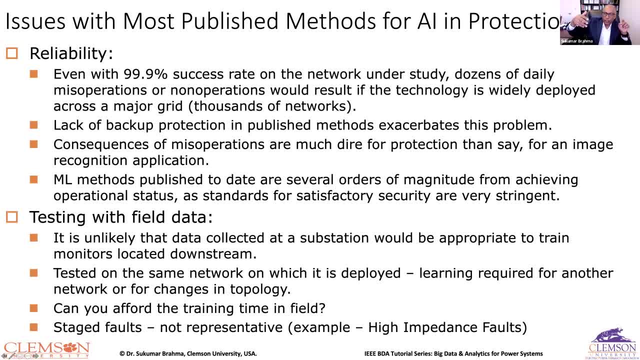 some device downstream, In other words, the data that you gather there downstream, the data that you gather at the substation. are they interchangeable? Can one data be used to train everything in the system? Think about that. Okay, It is usually trained for that particular network, So if you use it in, 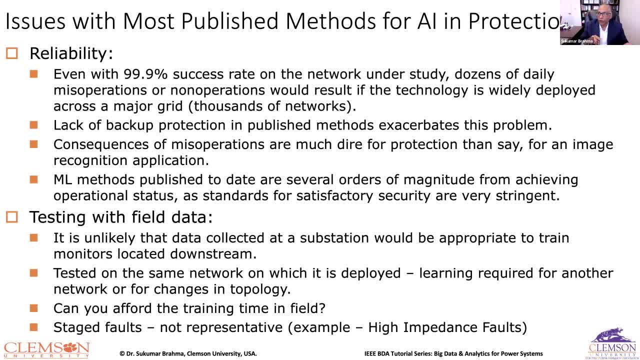 another network or the network changes topology- right, It needs to relearn. The fault patterns are changed now, right, So is that okay? Can you afford that? training time in the field? Can you do that? Can you wait? Also, people have done staged faults. 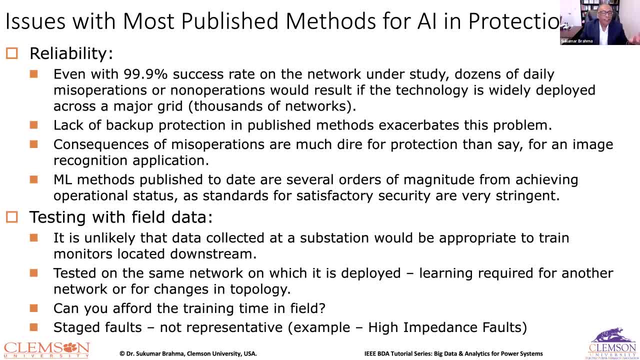 To gather the test data. but staged faults are few and they are not really representative of all the faults that take place. An example is a high impedance fault, for example, of a lot of people have used AI and it's a worthy method to use for this, But look at this high impedance fault. 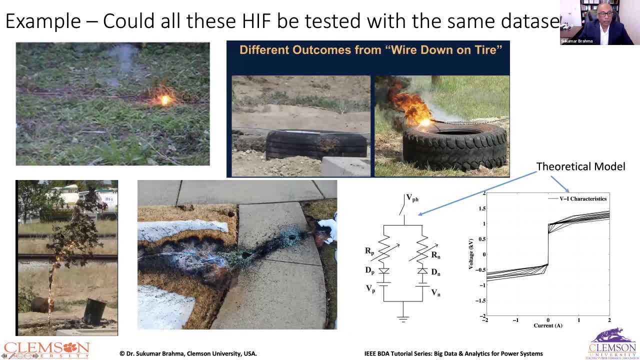 this high impedance fault, this high impedance fault. There's a tree burning here and this is a concrete- this is basically just you know, destroyed because of probably a 34 kV line or something like that- that has fallen the conductor, live conductor, falling The fault. 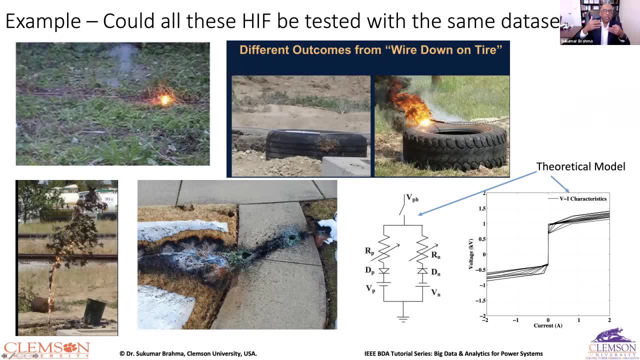 signatures of both voltage and current. High impedance fault is where the current is so low that your usual methods fail. There's no overcut, But it's very dangerous because it's a live fault and if you don't do that you're going to fail. So it's a very dangerous fault and if you don't, 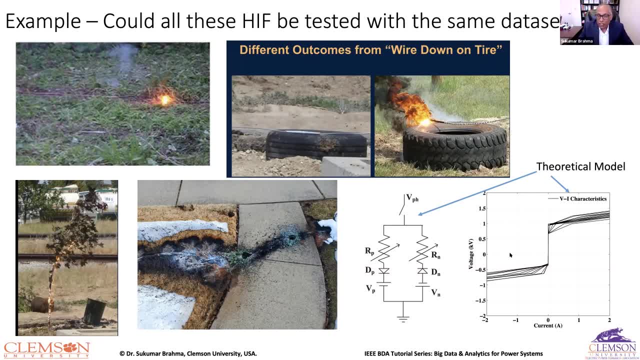 do that, you're going to fail. So if you don't do that, you're going to fail. So if you don't detect it, you're in trouble, right? So we have created theoretical models, you know, and we use. 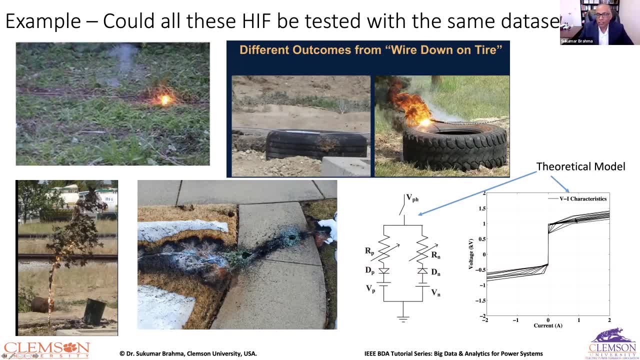 that, but people are saying, oh no, that's not, you know, doesn't, is not representative. But can you, if you create staged faults, would it represent all this? Again, a question that needs to be examined. Data Data is- and I think you all of you know who use, who have. 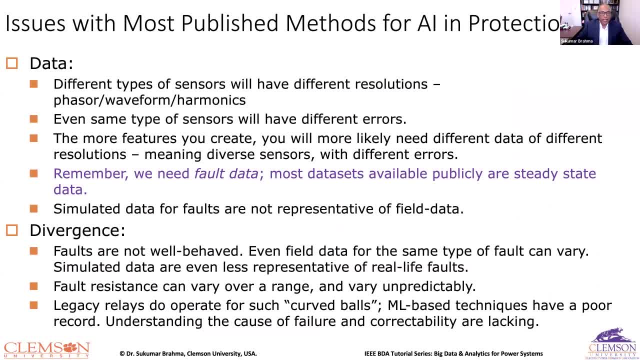 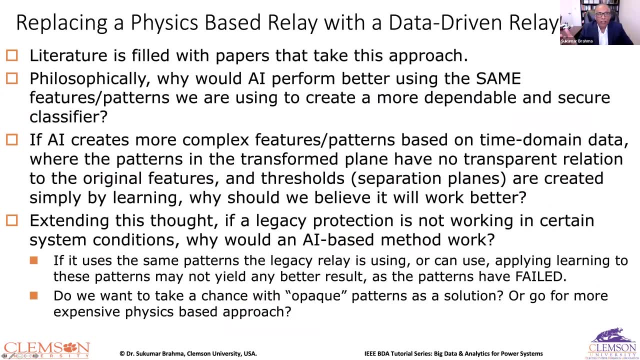 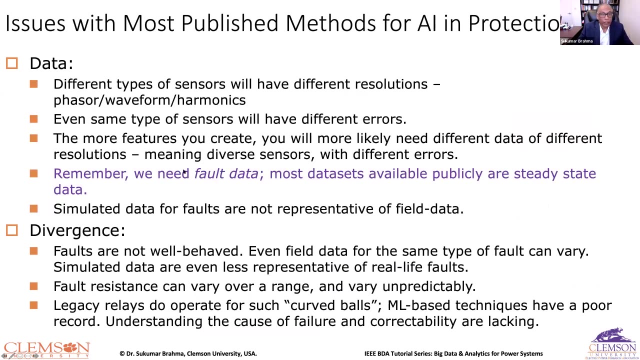 who have power, who work in power systems. that data is a problem. First of all, look at this bullet. Now there are public domain PMU data, public domain system data, But we don't. we want actually faulting right What happens in the steady state. we 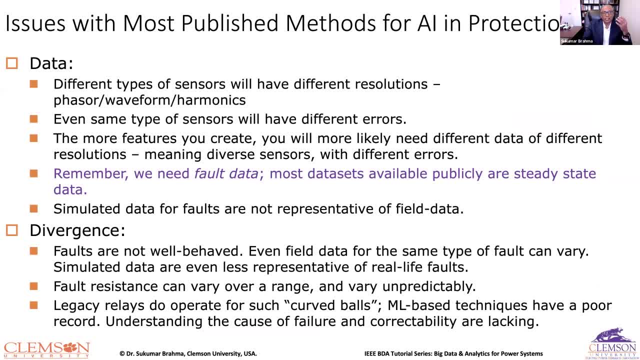 it's not of any use to us because the relays are operated during fault. How many false data sets for false do you have? That is important. So again, if you use different sensors, they'll have different resolutions. There'll be phasor, there could be time domain. 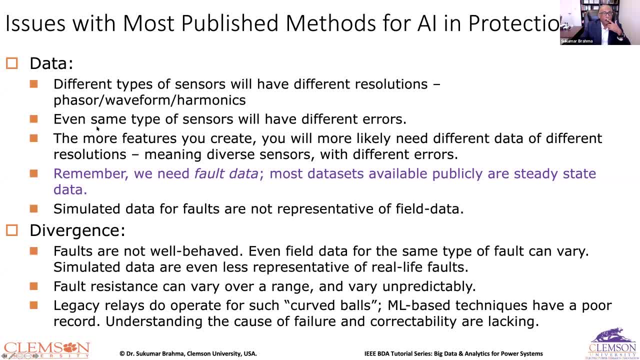 waveforms, there'll be harmonics. Even the same type of sensors will have different errors. A CT could have variable error between plus and minus 10%, So understand that The more features you create, the more likely you need data of different resolutions. 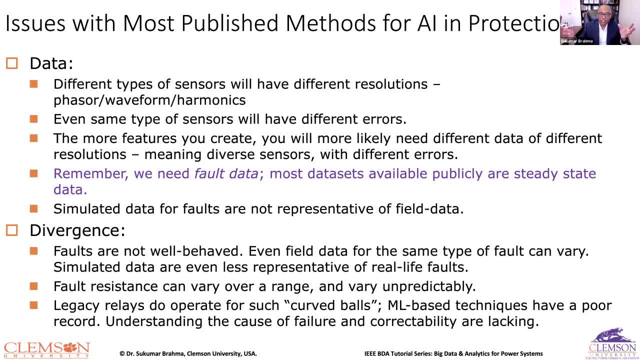 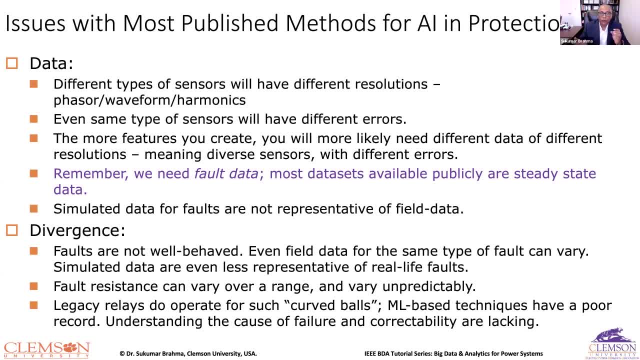 and they have been able to work around that. But when you do a machine learning-based approach, remember that there are errors and you cannot assume very, very accurate measurements, So that's another thing that you need to take care of. And then divergence After. 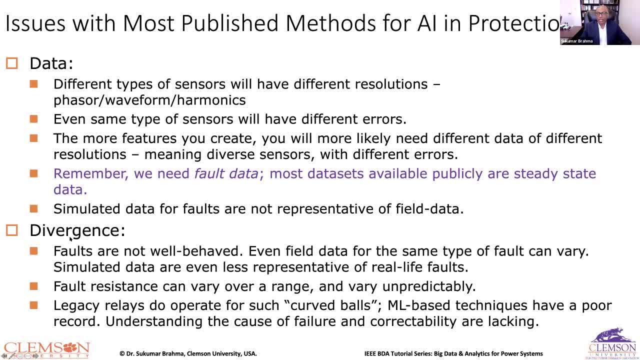 all this, the faults are not well behaved. Each type of fault, even the same type of fault, can vary from fault to fault And again, if you simulated data is usually very sanitized data and a lot of faults happening out there will not exactly or even very closely. 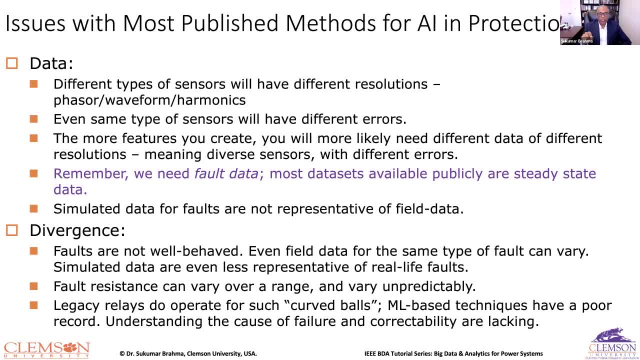 match your simulated data, you can only actually do a more accurate measurement. So again, if you your simulated data okay, And fault resistance is another unknown- that will change everything. So again, all these what we call covered balls, the protection systems, today legacy schemes. 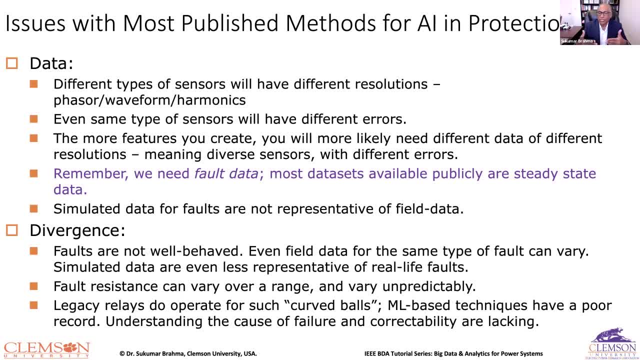 can deal with this. They have incorporated these aspects in the design, whereas for machine learning-based systems it's not yet shown. And this is something you might relate to. for example, a self-driving car after all those 100,000 miles of whatever they did, and then they. 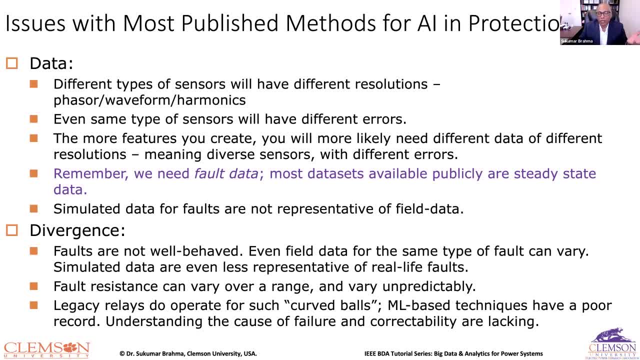 put it on the road and it killed somebody. So if there is something unexpected, the ML- the machine learning-based techniques- are very suspect to deal with it. So these are some of the things I thought that you should know, okay, So that when you design the schemes, you're aware of these pitfalls. 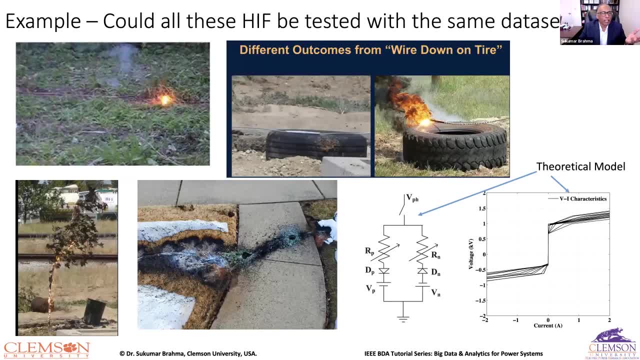 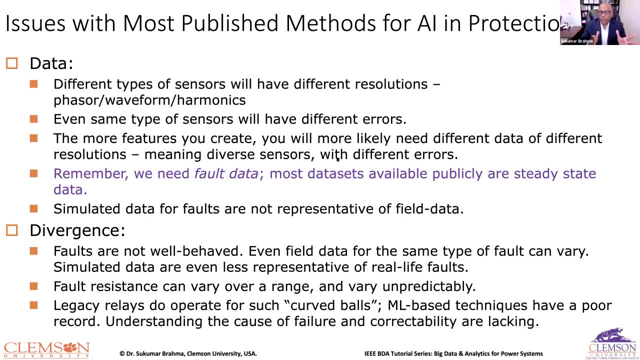 So don't think that I'm kind of, you know, pessimistic about it. I'm just being realistic about these. Now, if you replace a physics-based relay with a data-driven- okay, which is what most papers do- They're saying: okay, here's my 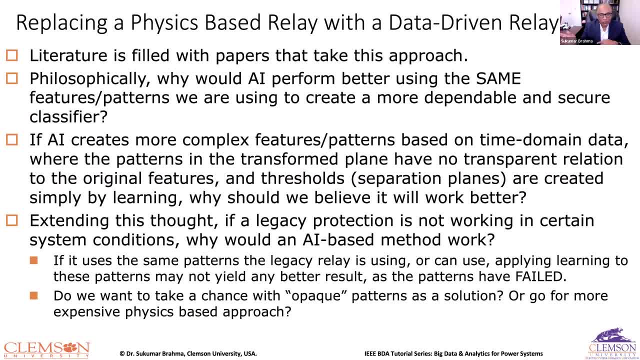 data-driven relay testing, rather training testing. we're done. Well, they are still using the same features. They're using current voltage, frequency, rate of change of frequency. All these features or patterns, you know combination of features, are already. 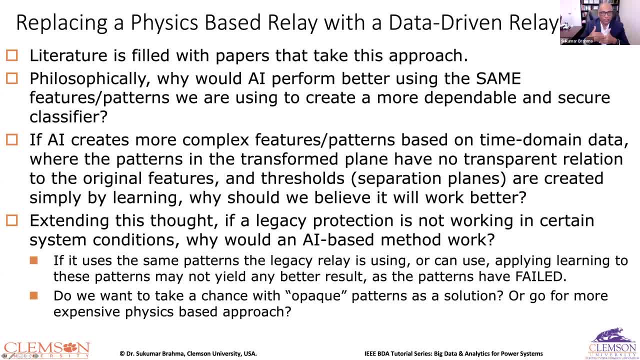 used by the relays based on the physics. So what is the guarantee that if you use the same patterns in a machine learning-based or a data-driven relay, you will provide better performance? And I'm not saying you won't, I'm just saying you need to address this question. 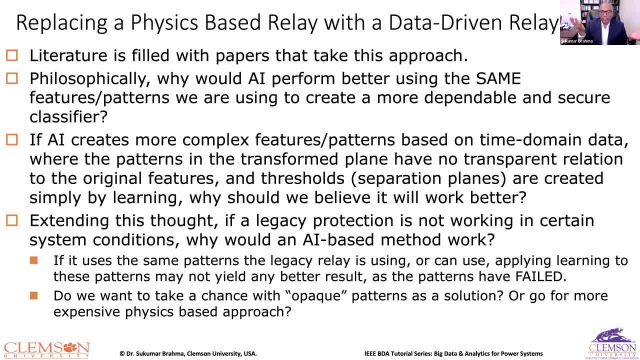 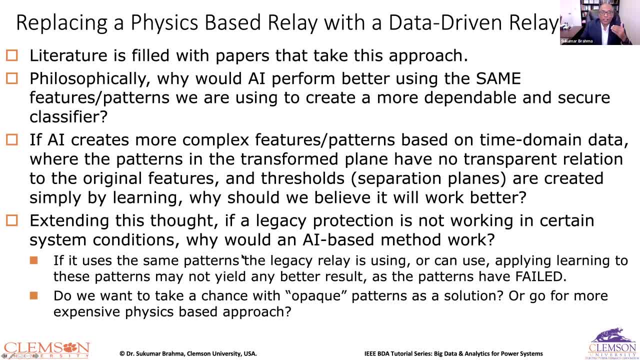 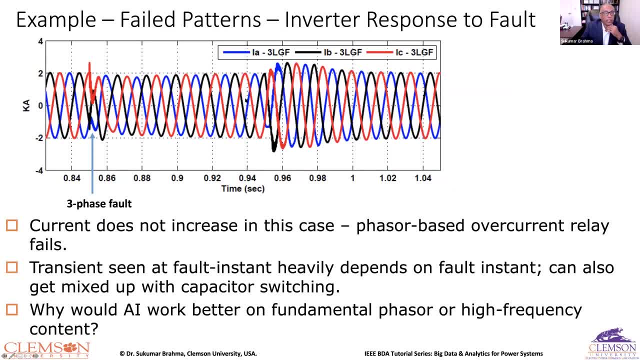 industry today, in the power system, distribution system today, with inverter-based relays or inverter-based resources, the overcurrent principle is failing. Why? Because, look at this, This is where so there is an inverter. Inverter typically limits its current and the fault is taking place. 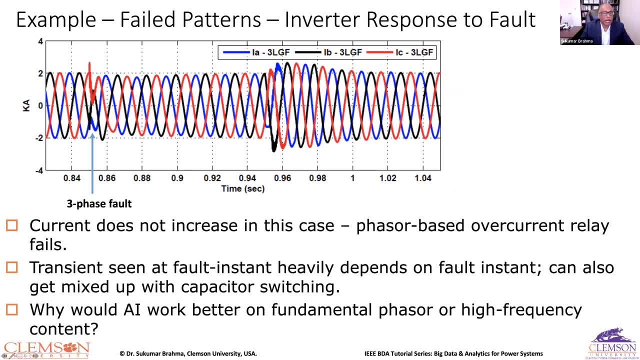 here and after the fault the currents are hardly increasing. So in this case I've limited the currents to the same as load current- Typically it's 1.1 or 1.2 per unit, which is not a fault level current. So that means that the overcurrent principle 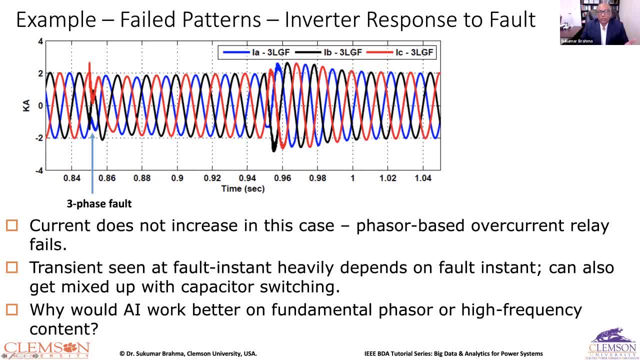 has failed So well, don't use. if you use the overcurrent principle in data-driven relay, it is not likely to succeed. So that's the point I'm trying to make is: what is it that you're using in the data-driven approach? 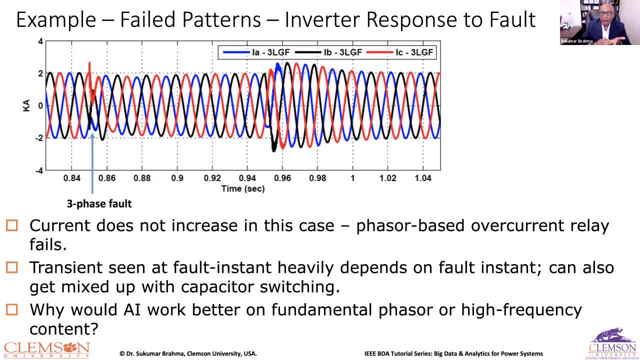 that is superior to this. What features will you create? What inputs will you take? And the features that you create? you have to show that those features are performing better than just the interpretation of those features based on physics. I'm hoping I'm making myself clear here. 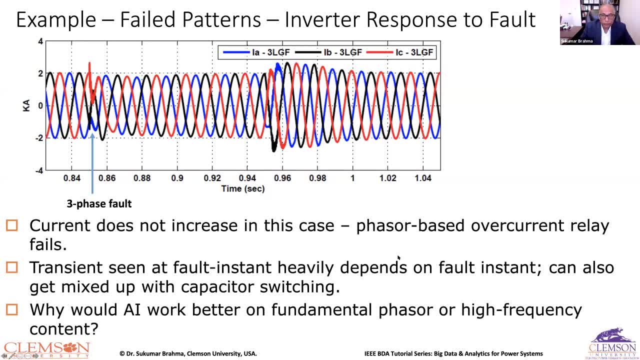 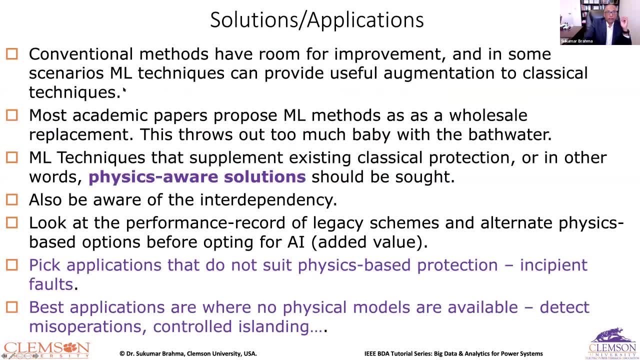 So solution? So yes, we agree that there is always need for a room for improvement And in some scenarios the machine learning techniques can provide better performance, augmented performance. but don't throw the baby with the bath water. Okay, keep the baby there. 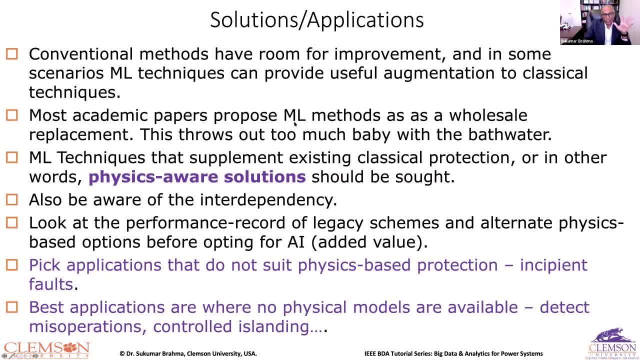 So don't replace, in my opinion, okay, don't just replace- a machine learning, a physics-based method, with a data-driven method. okay, There's something that is going on in the and you know, you guys know this more than I do. 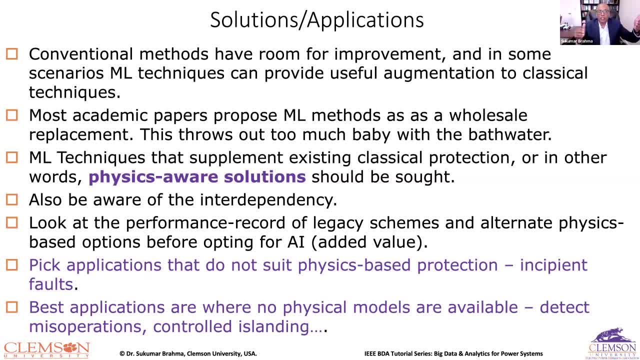 that's called a physics-aware solutions. That means you use the physics in your solutions, because I think the argument for this I've seen that you know, if it's just computation-based, it becomes extremely expensive, But if we use physics in it, 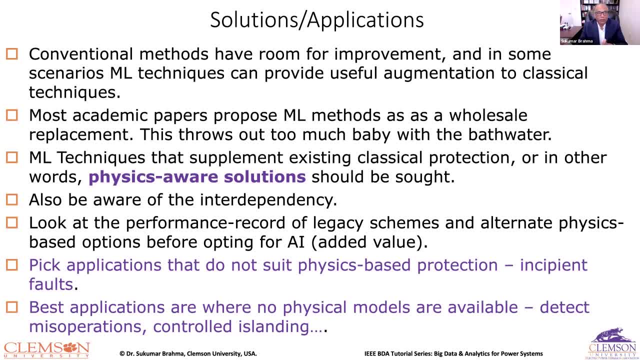 then it becomes more reasonable to compute, The computing part becomes easier. But in this case actually the performance will get better if physics is you know, if you take physics as a friend and use it in your solutions. Also, the other thing is obviously there are applications. 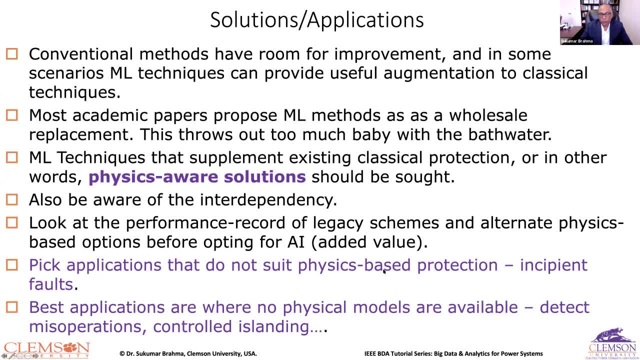 that are not suitable to physics-based protection, For example incipient fault. The fault has not happened, but it is about to. You know, the insulator is getting worse, It's deteriorating. It's not failed yet, but it's deteriorating. 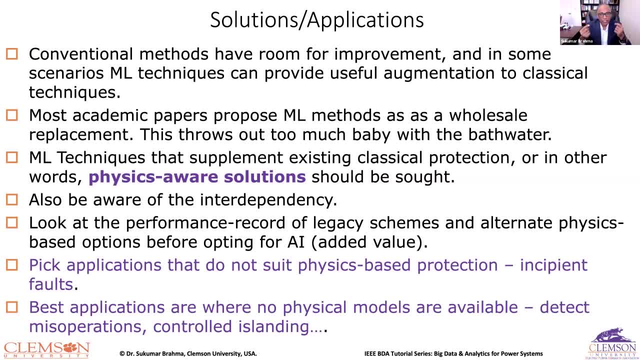 Something like that. the machine learning-based methods would work wonderfully there, because there is no physical model there, right? The other is, you know, detect misoperations. As I said, misoperations are still not detectable in real time, which is very surprising and very frustrating. 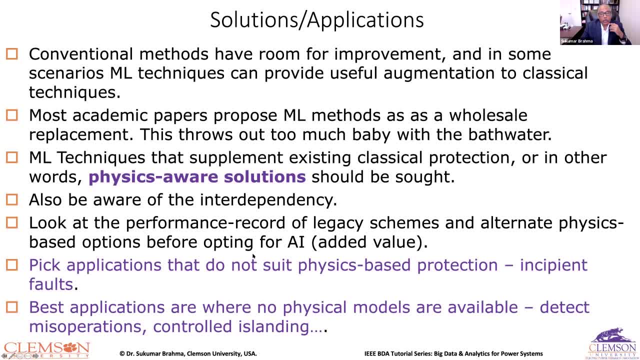 but that is the case, okay. Controlled islanding, for example, When there's a power swing going on, you don't want to just strip the relay that sees the power swing. You want to make sure that if there is an instability going on, a swing is getting unstable. 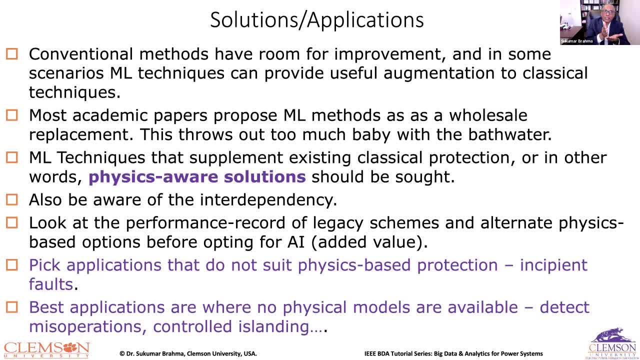 the system should be separated, separated at certain boundary so that the resulting separation, the two islands that are created by the separations, remain stable. All this is usually done offline, through offline studies, and this is also called part of system-integrated protection schemes. 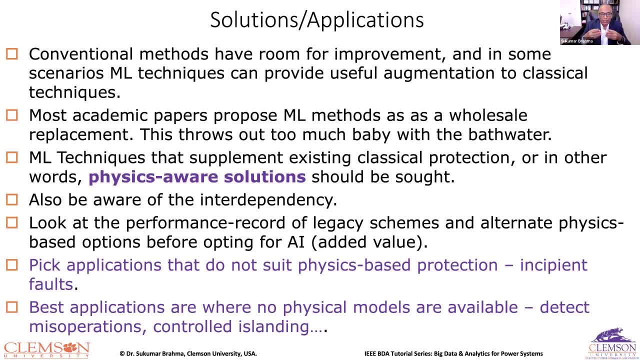 which are system-based, not local, And there it is always set based on offline analysis And if you can do it using real-time data and inform that system-integrated protection schemes to operate in a certain way, if you adaptively change their settings. 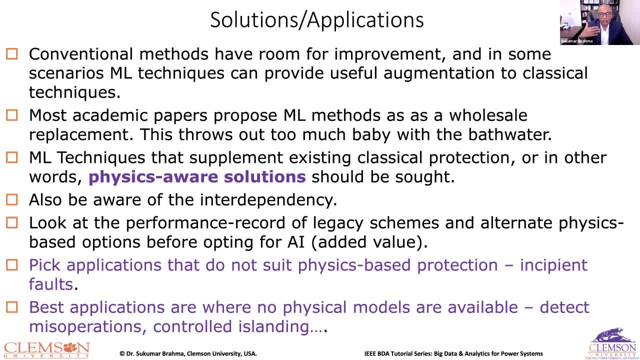 based on the system condition. that'd be great. That's probably the holy grail, and I'm sure so. you know Vijay Vittal, right? He was saying the other day that we still got to come up with a killer algorithm, right? 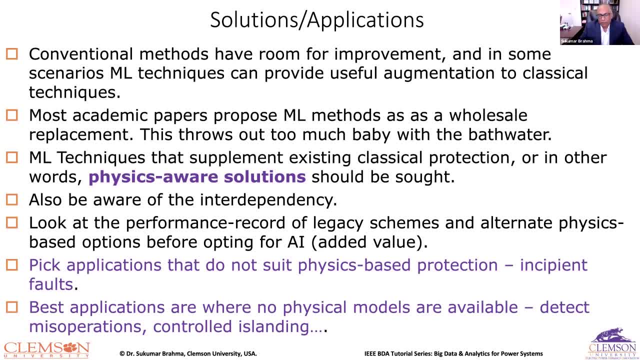 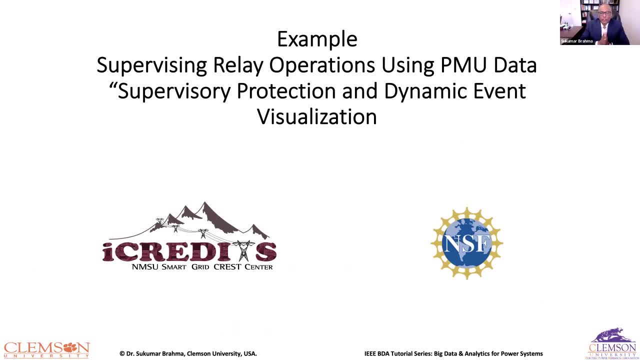 A killer app using PMU data, And this is one of the killer apps. If you can do this, that would be great. Okay, so we got some time. Let me give you an example. So this is what we did. 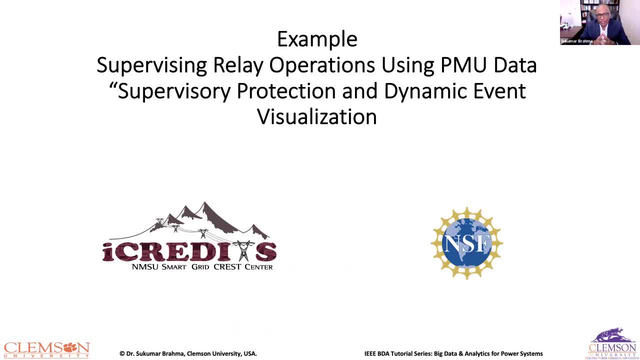 when I was at New Mexico State University, we had an NSF-funded center there which we called iCredits, and after five years working there I still don't remember the whole full form of iCredits, but there is a full form there. 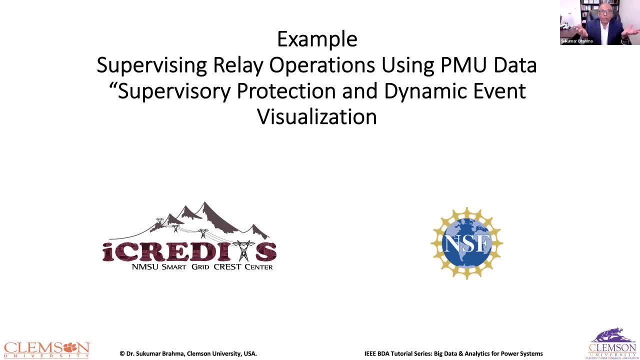 And it essentially was given between computer science and electrical engineering department. The electrical engineering department mostly power systems people, and the computer scientists were, you know, data scientists, communication experts, you name it. So this is something we did there and I want to give that as an example. because it'll kind of show you, you know what's going on. So this is something we did there and I want to give that as an example because it'll kind of show you you know what's going on. So this is something we did there and I want to give that as an example. 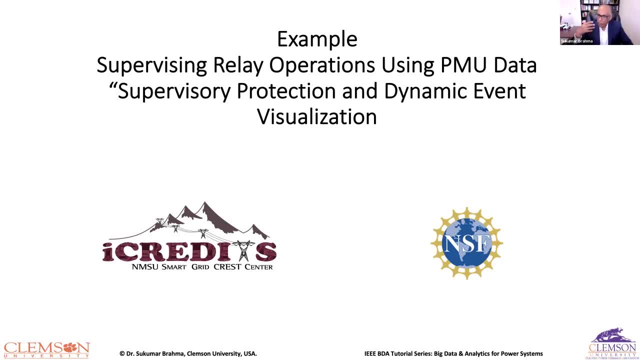 because it'll kind of show you- you know what's going on- That even with an application that is worthy of machine learning, how many obstacles are you likely to get into? how many obstacles are you likely to get into? Okay, So let's dive into this. 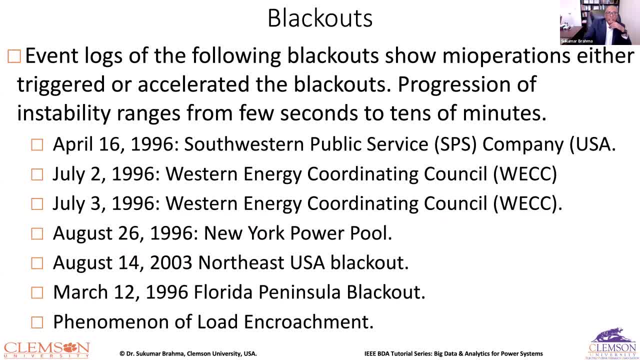 So, first of all, again coming out to misoperations, if you look at blackout logs, right, So these are only selected logs of blackout logs. So these are only selected logs of blackout logs that happened in 96, 96.. 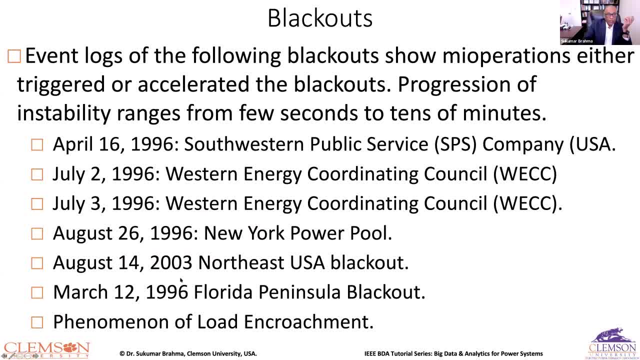 2003 was the biggest one. right, All these blackouts. if you look at the log, All these blackouts, if you look at the log, you will see that something misoperated, some relay misoperated, The settings were not proper. 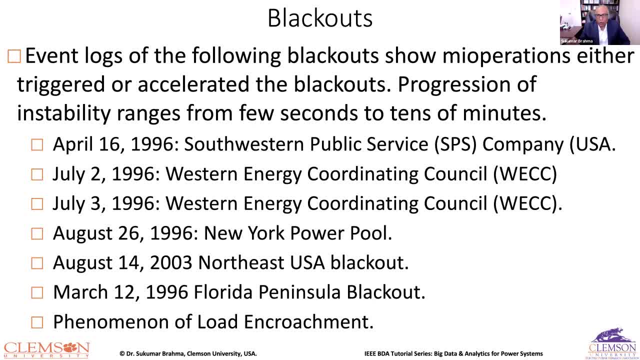 the relay had a problem that you know hidden problem that just surfaced at that time, But it misoperated And what happens is, And what happens is, it's just so, It's just so, Just quickly going to the next slide. 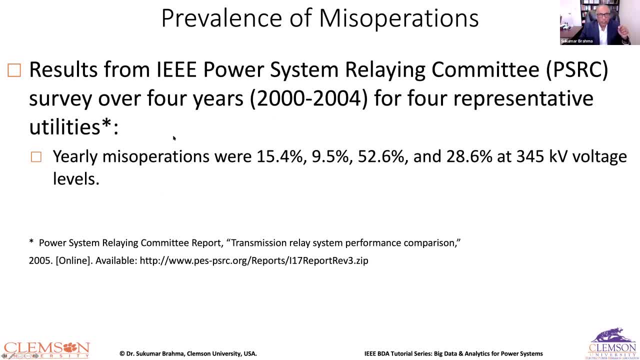 The Power Systems Relaying Committee actually made you know, performed a survey some time ago. Here is the report. The yearly misoperations were 15%, 9%, 52%, 28%. The yearly misoperations were 15%, 9%, 52%, 28%. 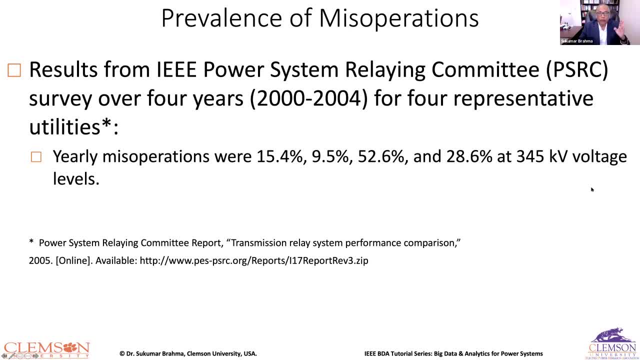 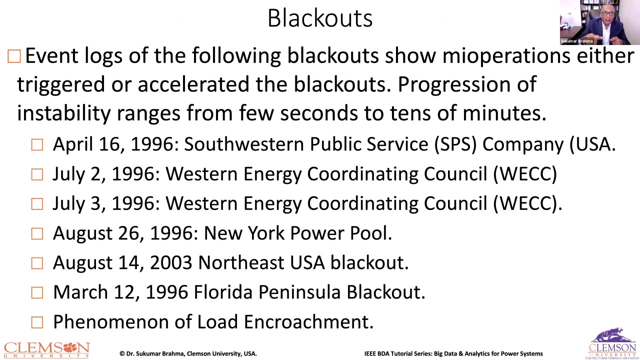 at 345 kV voltage levels for four different utilities that were surveyed. These are the. So these are not small right? But now every misoperation doesn't really result in a blackout, but these did okay. There you can actually see that some misoperation is responsible for either accelerating it. 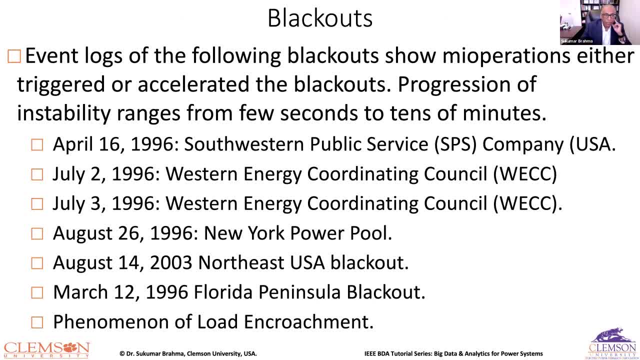 or, you know, triggering it. So it's a serious business, right. And there is a phenomenon called load encroachment, which is common with all distance relay. So if you look at blackout logs of- I guarantee every blackout- you will see load encroachment. 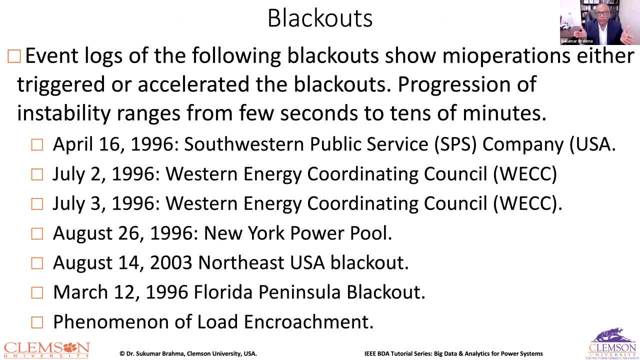 relay tripped on load encroachment. Essentially, what happens is quickly to give you an idea- if there are two parallel power lines, right, They are fully loaded, it's peak time they're fully loaded and one of them trips right. 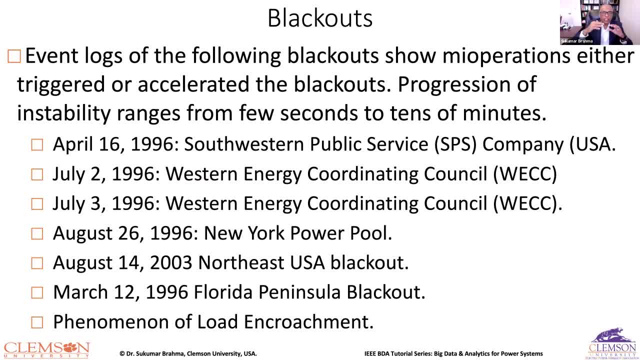 So, first of all, why would that trip? They are so much loaded that they become hot, they expand And they typically sag into a tree. That happens, the line trips And then the whole power is shifted on the other line, which for a distance relay that 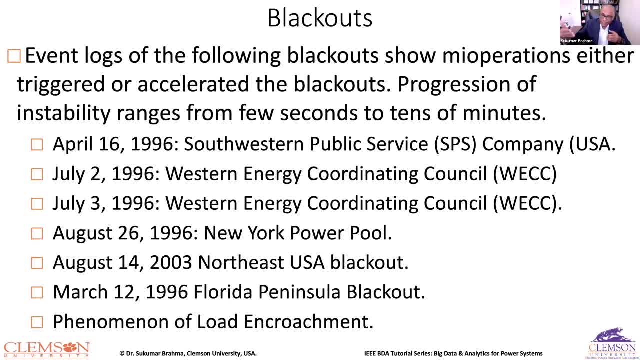 looks like a fault And the distance relay of that second line, which has no fault, trips, which means that it has, when you needed that line the most, it got tripped And that is how the blackout progresses. So the load encroachment. 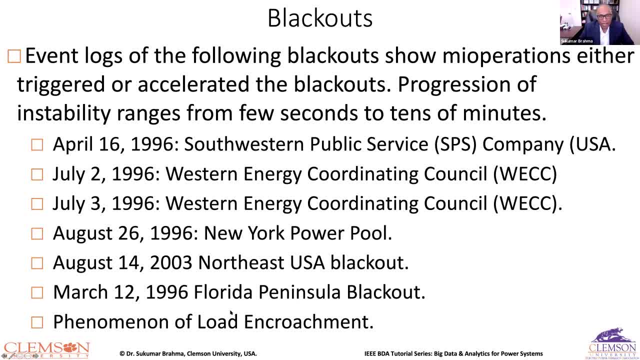 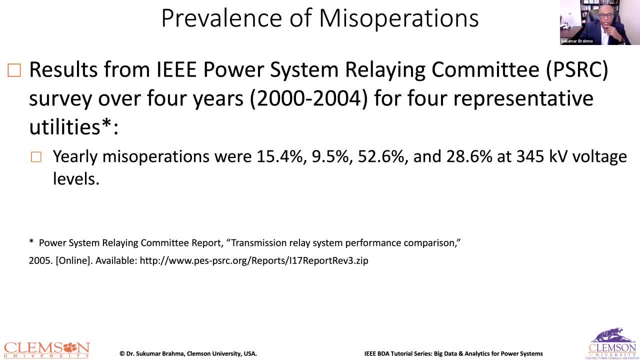 The load encroachment is very common for every blackout that happens, So that's why we So. when I started working with PMU data, this is the first thing I realized that, okay, how about we track this? Because now we have PMU data, can we use that to detect misoperations? 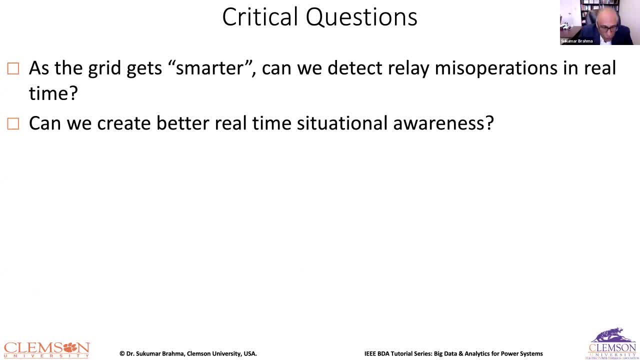 So that's what we were trying to do, And this is something you guys know. Professor Meliopoulos at Georgia Tech. he's also trying to do that in a different way. He's not using AI, he's using dynamic state estimation. 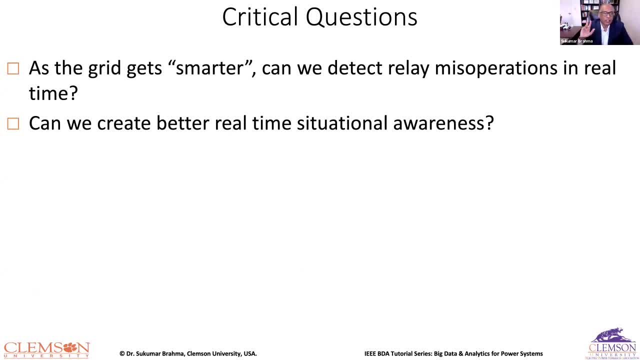 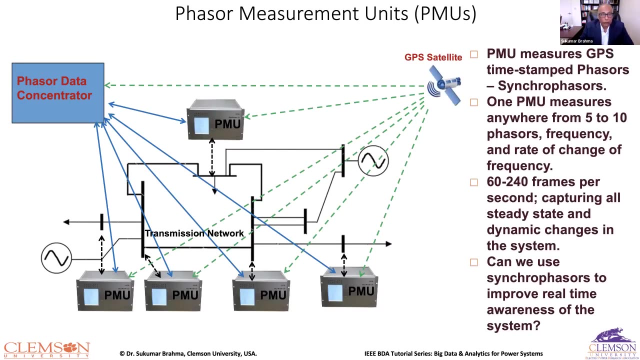 But it was interesting that two protection guys thought of the same thing about misoperations and started working on using PMU data for detecting misoperations. So of course, you guys are all aware how this works. There are PMUs And they feed to things like this. 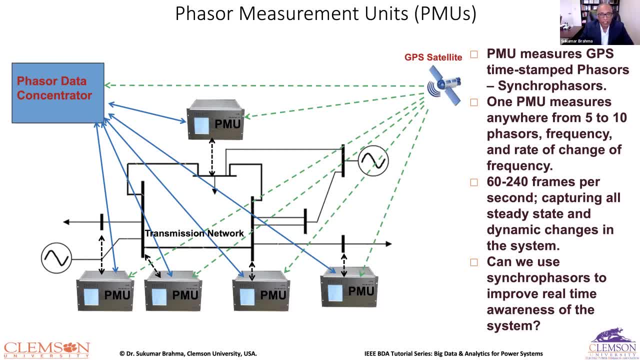 So that's what we were trying to do: Phaser data concentrator, and they're all synchronized because of the GPS right. The older PMUs had 30, even 10 frames per second. 60 is common now, 120 is pretty common. 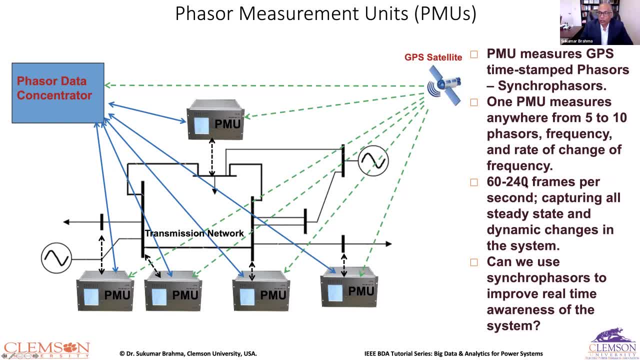 240,. if they're not there, they will be there. So 240 frames per second, that is a lot of data for our systems. Remember the SCADA data is much less than this, first of all in quantity, And it comes once every two to four seconds. 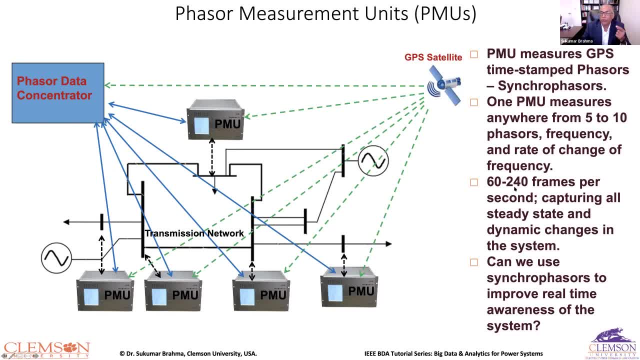 Once every two to four seconds. Now we are talking of 240 frames per second. That is why can you hear me? Can you hear me? Yes, I can hear you. Okay, good, I got a message saying your internet is unstable. 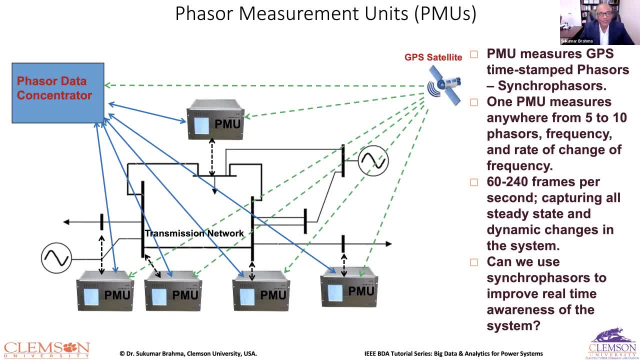 I don't know. I'm in my Oh, okay, Yeah, so I just wanted to make sure. So now, US has, at this point, I think, 1700. until what? was it? October 2014.. I don't know if I have the data before that, but after that. 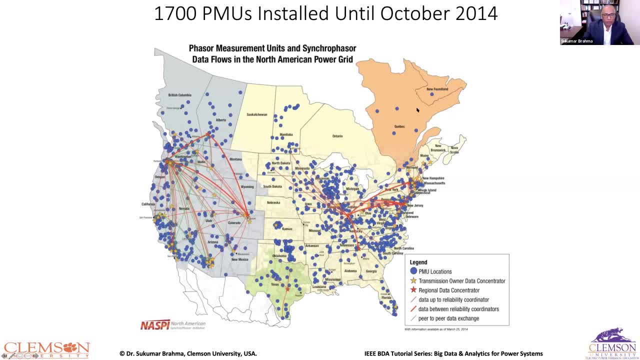 But it is a good data. It has slowed down, but there are quite a few PMUs here In developing countries, for example in India. it's a lot more aggressively. This is a lot more aggressively done. Okay, They are installing PMUs like crazy. 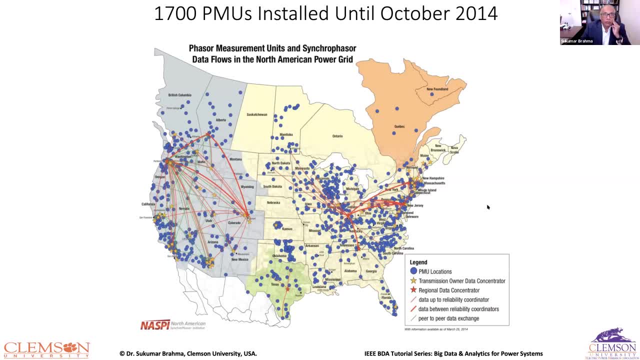 But this is what we have right, And so how can we use this to detect misoperations? So here is the concept that we came up. Okay, So the data are coming from PMUs And, as you probably know, the data needs pre-processing. 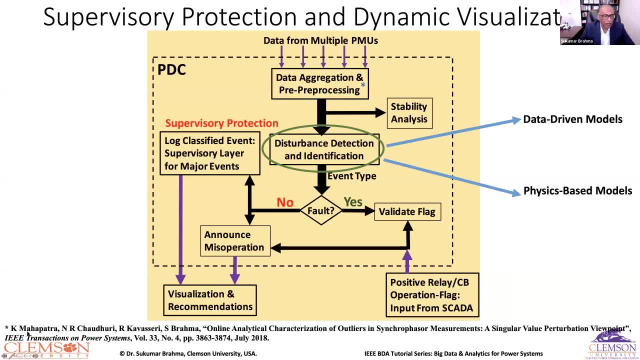 And we are not talking about pre-processing here. I'll just put a paper here, cited a paper here that we did based on. That was a part of another project, but that's So suppose we did that right. And now the pre-processed data comes in. 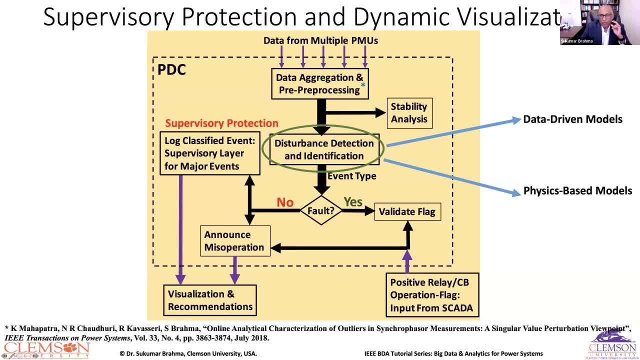 And I think a lot of you who are working on PMU data have probably worked with disturbance detection and identification. What type of disturbance is this right? That's a very popular application of PMU data And we actually did it both using data-driven model. 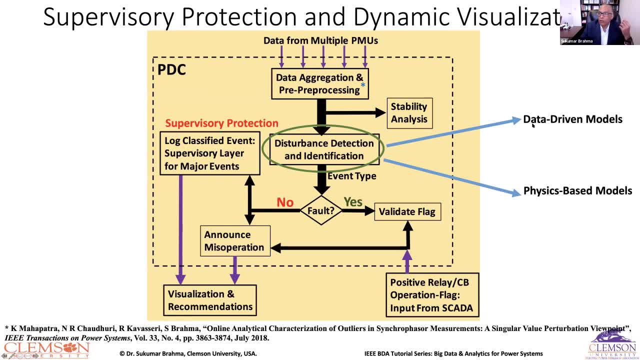 and then we used some physics-based model to inform our data-driven models, And we'll talk about that in the coming slides. Now, actually, what I'm interested in right now for my application is this: whether that's a fault or not, 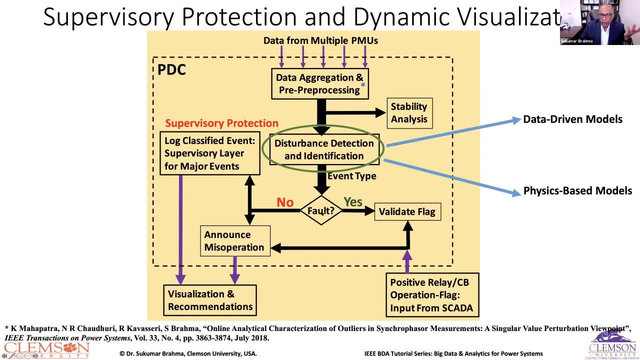 If it's a fault and if the relay has also operated. so what it does is it sees if there is a relay that has operated- because when the relay operates it provides a flag- And if the PMUs detect that there is a fault. 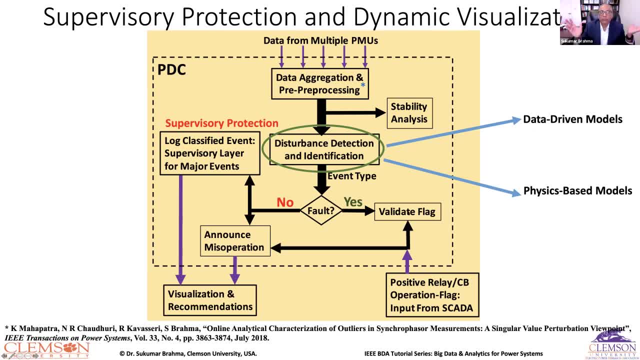 and the relay has already operated. we're good It operated for the right reason. But if the PMUs don't detect a fault and and you see a flag, then that's a misoperation, Right, And then that misoper. 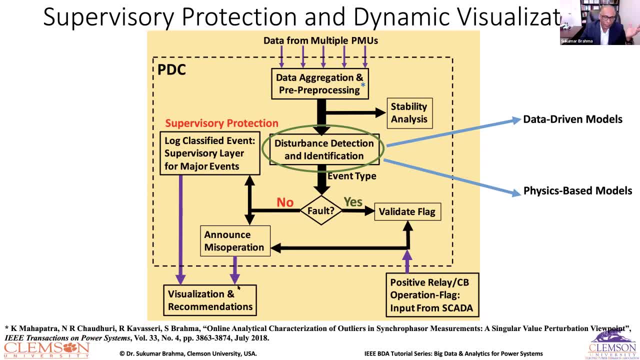 How do you handle misoperation? Well, it depends Typically you, the operator knows, and then they take, you know, they close the line back or something like that, or take care of the you know, disable the relay or replace the relay whenever possible. 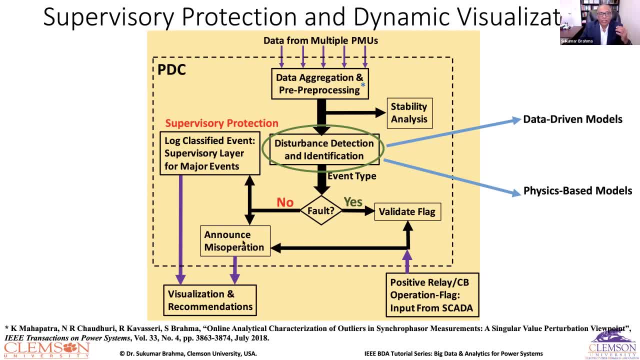 But at least there is a misoperation detection in real time. So that's what we were interested in. But since we were identifying fault, we also said we'll identify other disturbances as much as possible so that we have a a supervisory layer for major events. 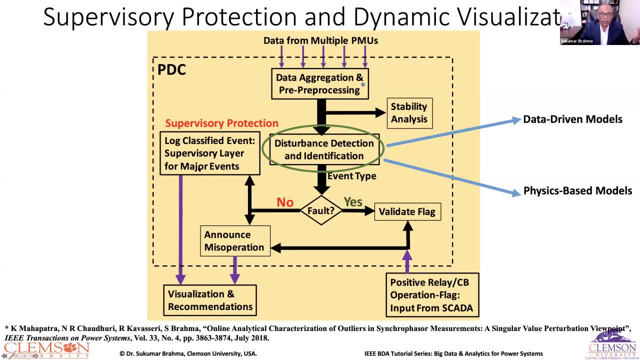 if there is a, you know, dynamic event going on: generation loss, load loss, capacitor switching. So it's better. you know it's basically we did that as well. So that's a visualization screen. What So now? first of all, 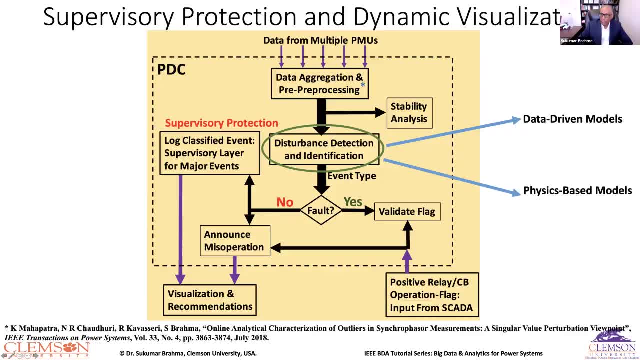 I don't know how many of you have actually got PMU data for disturbances. Again, remember I said that I don't care if you have loads and loads of PMU data for for steady state or normal system. I want PMU data for disturbances. 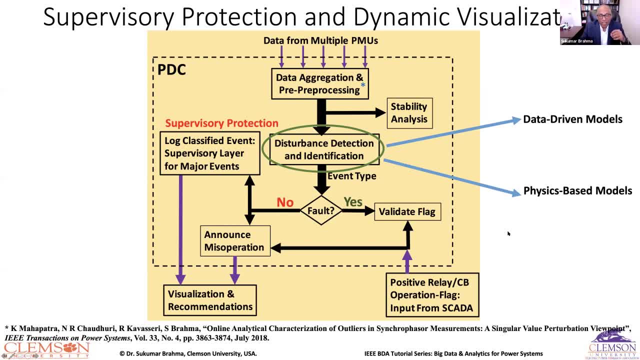 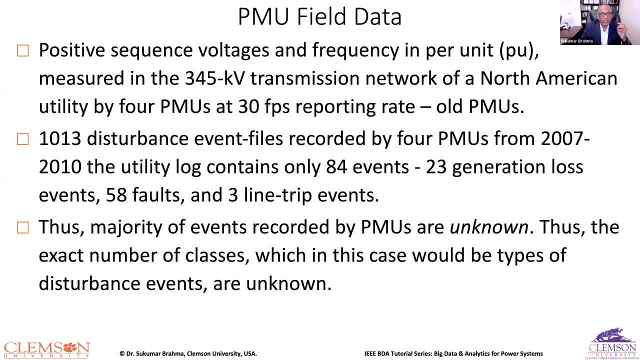 Right, It is very, very hard to find, But we had a utility, who were kind to us and they said here, So they had old PMUs, okay, 30 frames per second. They only had positive sequence. Now you have phase A, phase B, phase C. 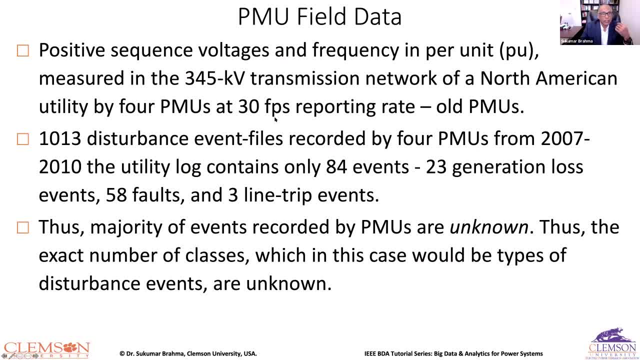 But they said, okay, you know what? what we do is we store all the PMUs. basically, when they see there is a disturbance, They recognize it because it you know rate of change, of frequency or something like that will trigger that. 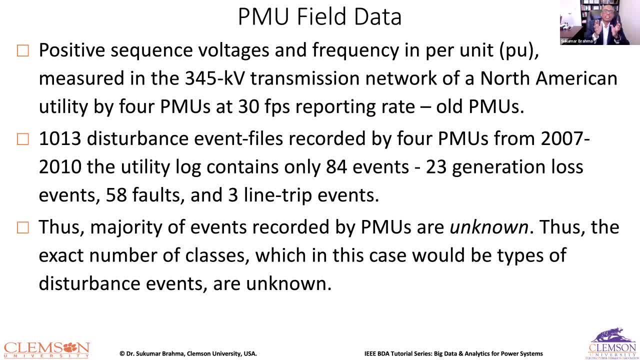 And it stores that disturbance files separately. So they said: okay, you have for four PMU for four years. we have all the disturbances that happened. We have them Okay Now, so you can take them All right. So how many did we get? 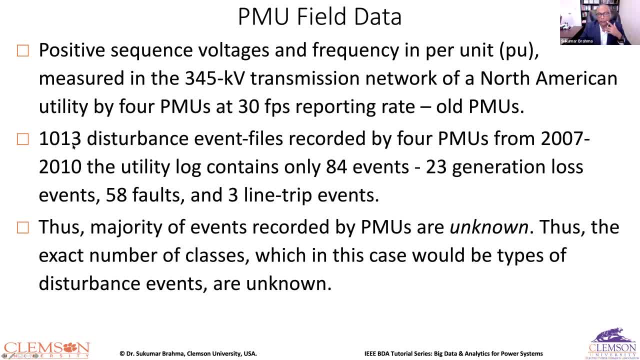 1,013 disturbances. Even files were we got. Okay. Now I said okay, so we have quite a few known events. But well, they were just disturbance files. We didn't know what those disturbances were. So I sent a student to the utility. 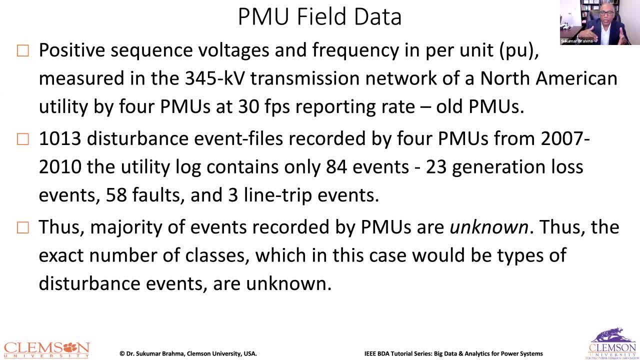 and he just went through the log of the utility And you know how many log entries he found: 84.. Out of 1,013.. So the ground truths that we really want for any application only: 84 events, 23 generation loss. 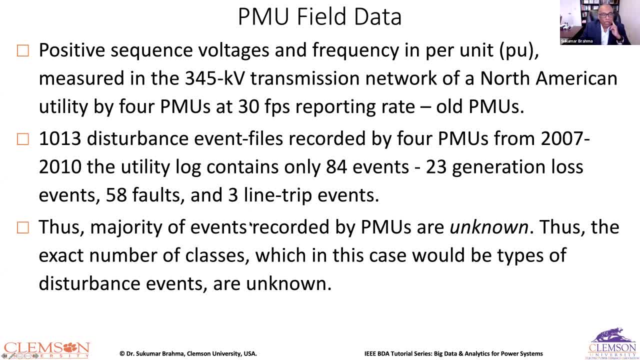 58 faults and three line trips. Okay, So the majority of events, even if you get it, could be unknown, Right, Which is really disappointing. So now the rest of these events. what are those? We don't know. 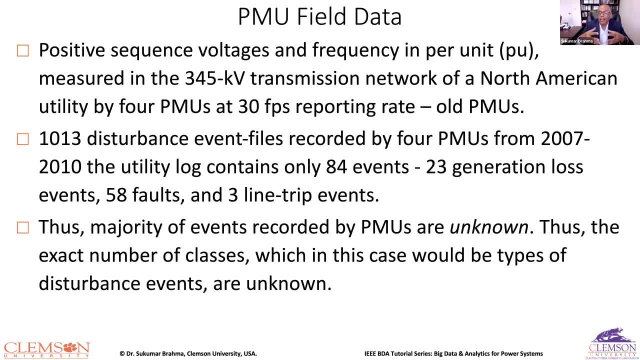 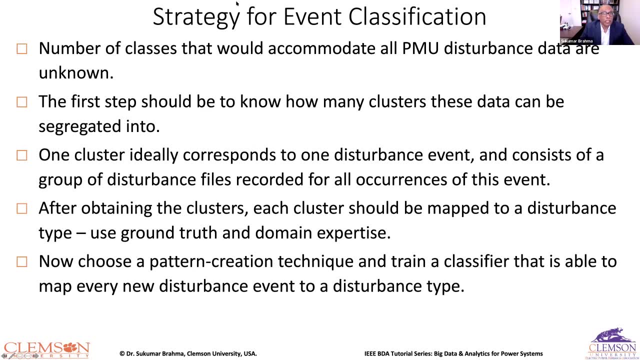 Right. So what are the exact number of classes that are residing in this data set? We don't know. So that's where we started And we said okay. so here is our strategy. First of all, how many? So we need to cluster these data. 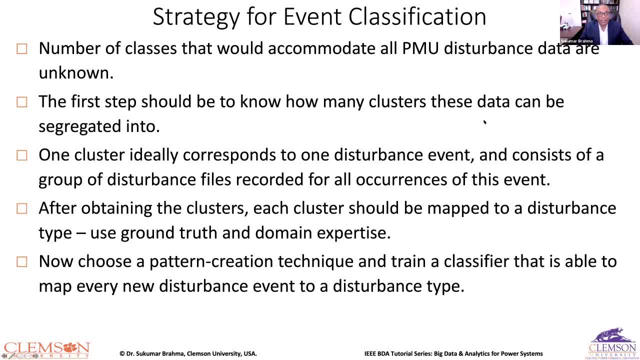 Right And figure out how many clusters these data can be segregated into. Right, And then, hopefully, each cluster will represent one disturbance event. Okay, And then we'll find out how many disturbance events are residing in this data set. Okay, And then, once we know, 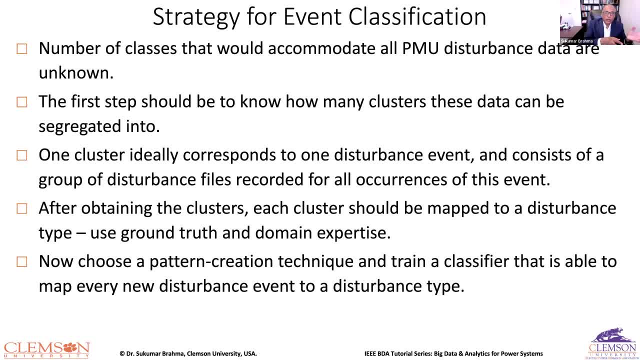 how many classes we have. we use training and testing because now we have how many classes we have, we know. So then you can form your classifier. So this was our strategy And this is where you know working with a data scientist. 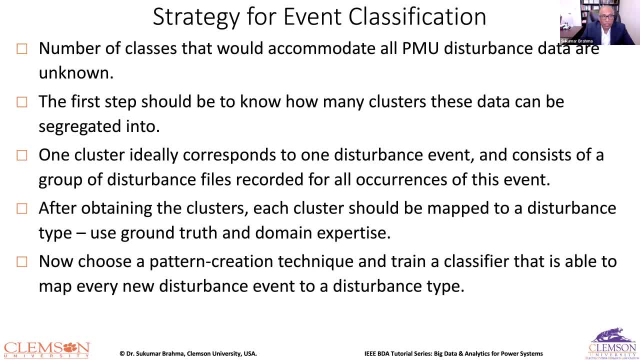 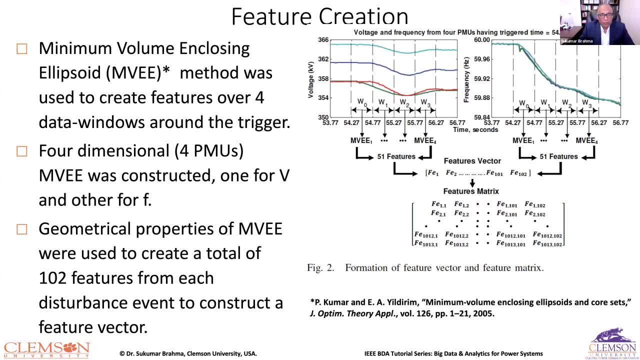 was very helpful to me because she was, you know, she knew what to do For this. the features that we used- and I'm not going to go into too much detail here- Most of you, if you are working in this field, 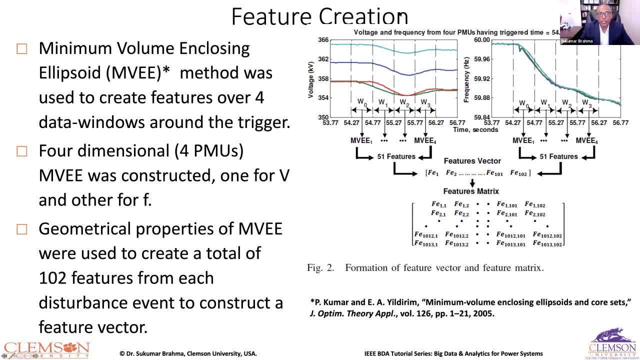 this is a very early work that came out of PNNL, where what they call minimum volume, enclosing ellipsoid M-V-E-E. So they basically create an ellipsoid and the dimension of the ellipsoid equal the number of PMUs And it's. 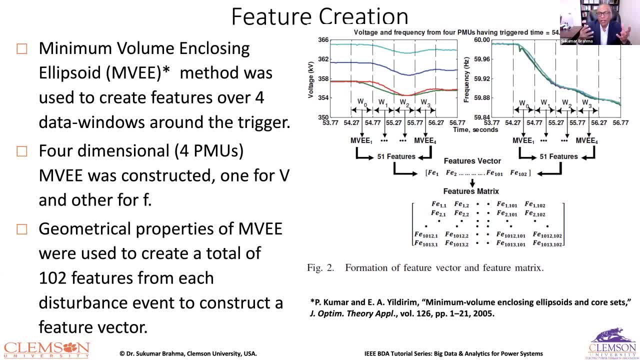 the method looks more or less like a singular value decomposition method, But what we did was, if this was the file, this is where obviously the disturbance is- We took a window before and then three windows during the disturbances, And for each window. so it's essentially 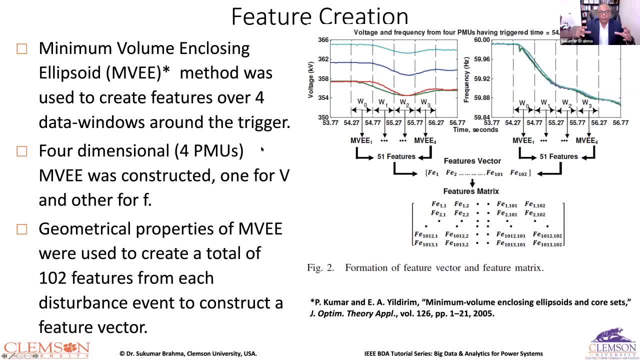 what happens is it forms an ellipsoid And then the shape of the ellipsoid is different, based on different disturbances. So the property, the geometric properties of the ellipsoid will be used as features, And so initially, since this was done already, 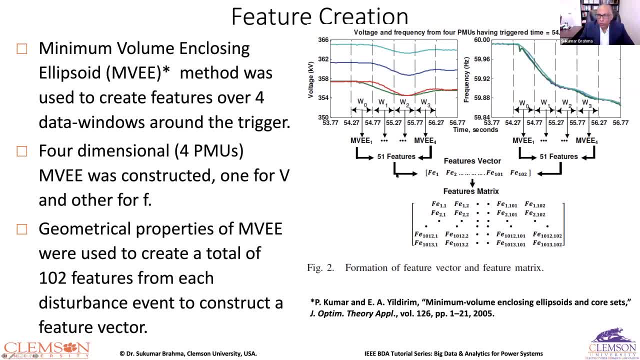 it has shown good results. We used that, So we used that on voltage, We used that on frequency, So we create 102 features And there were obviously 10, 1,013 events, So each event was captured as 102 features. 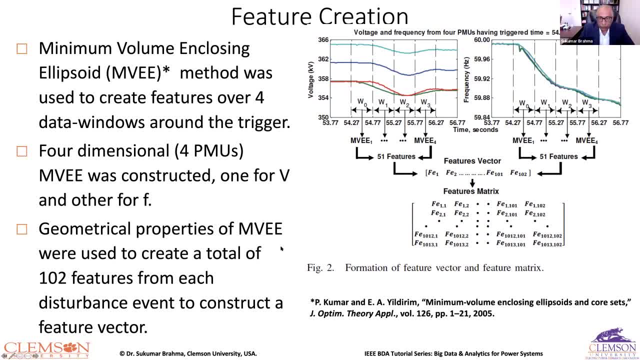 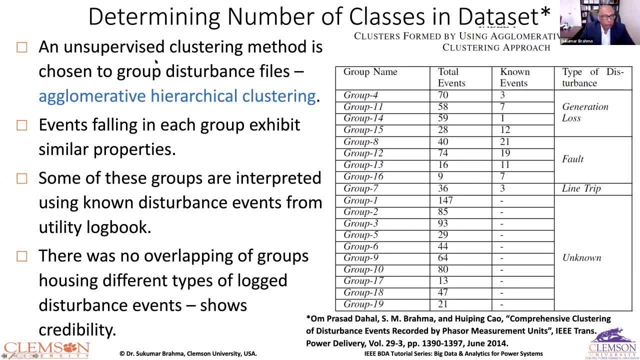 That was our feature matrix, And then we used an unsupervised clustering method, Because this is what you, you know, we do: if we don't know how many classes are there, We used agglomerative hierarchical clustering. And when we did that, 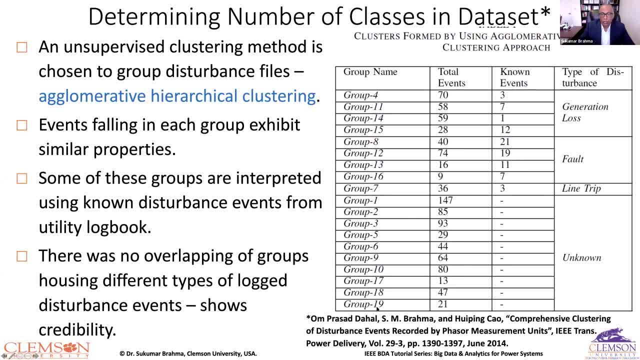 right. we got 19 groups Right And these are the events that fell into each group. These are the total: 1013 events were divided into 19 groups. as you see here Now we looked at the known events and the known events were. 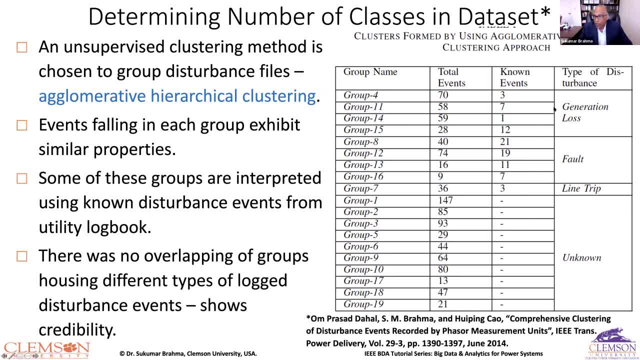 here was: the generation loss was spread across four groups, Fall was spread across four groups And the line trip was just one group of. you know all three events. Why is it spread across four groups Where there could be a smaller generation loss? 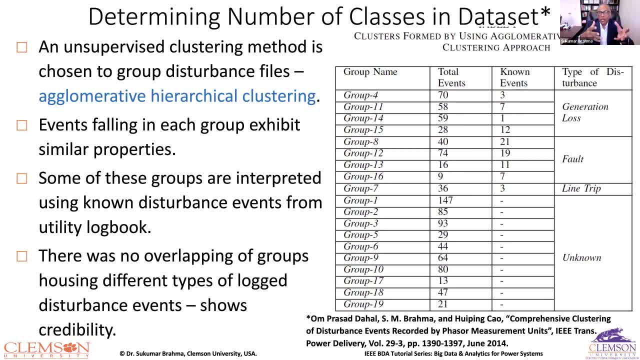 there could be larger generation loss And what this method did was that it actually created different groups for smaller and larger generation loss. But the good thing is there was no misclassification. None of the fault event which was known event fell into the other group. 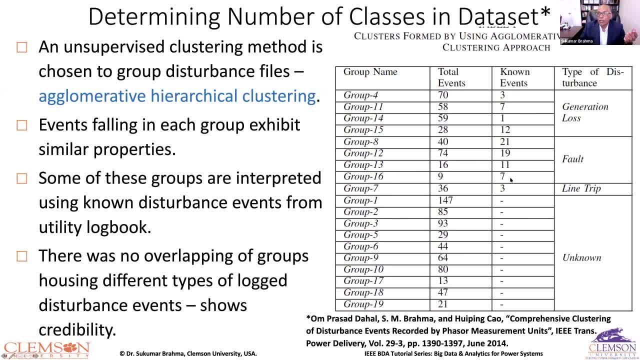 for generation loss and vice versa. That gave us some confidence. Okay, this is working. So all we had to do is, you know, make one single group of all four, one single group of all four, But then these are the ones that 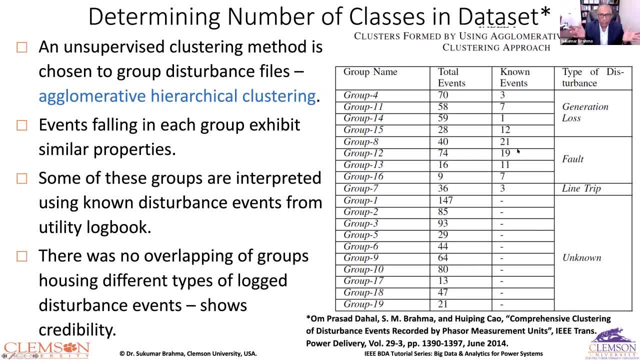 so because of this, we said, okay, this is working, This is doing a good job. However, we don't know what these groups are. These are other events. These are not generation loss, These are not falls, These are not line trips. 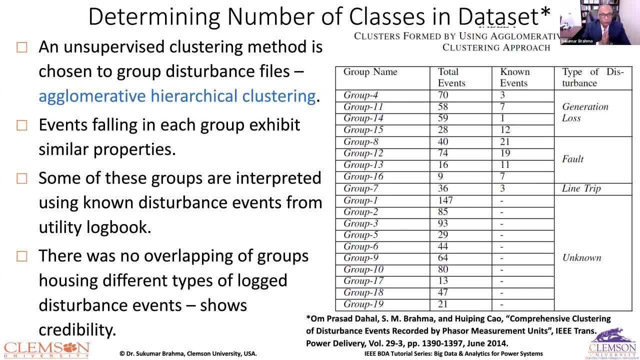 These are something else. So now, what do you do Again? so in this case, we then started look. so here is where the domain expertise comes in very handy, for this is a power system, Our system problem, right? So we started looking at these. 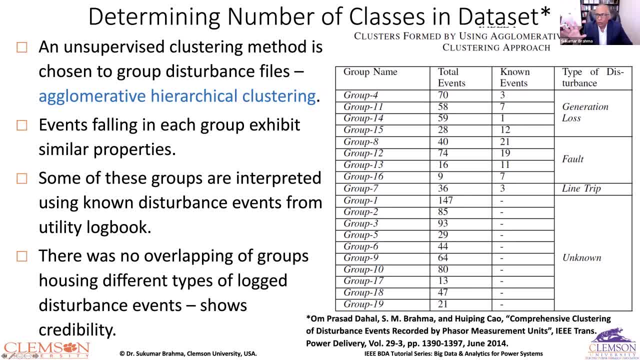 and we said, okay, this looks like a load switching on, load switching off. There were series capacitors in there. So that's what me and my students started looking at and says, this looks like this. Okay, So let's say, if 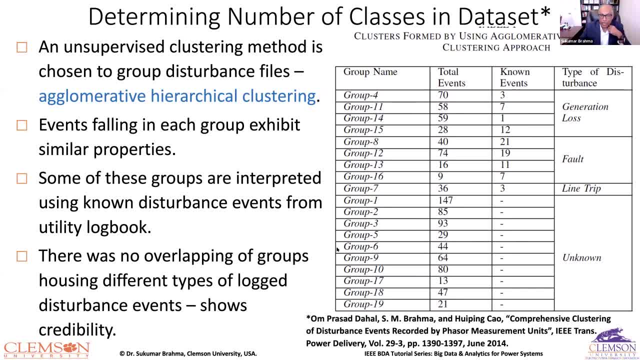 you know. so now, how do we confirm that it is like that? So, fortunately for the system that we were using, the four PMUs was in that Southeastern system and other Southwestern system And that was already modeled on PSLF. 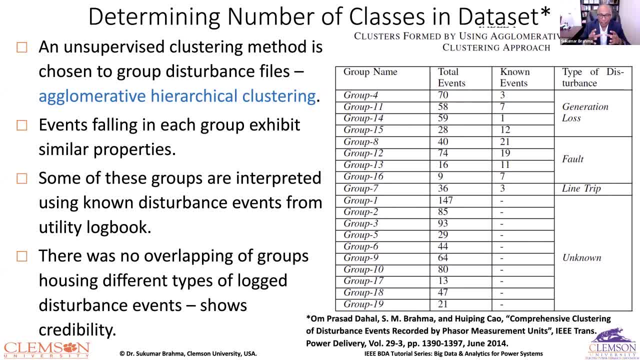 So we had- we actually bought PSLF license and those, those test cases, And we ran these events that we thought you know, load switching, capacitor switching and all that. We ran those as simulation events And then we added those events. 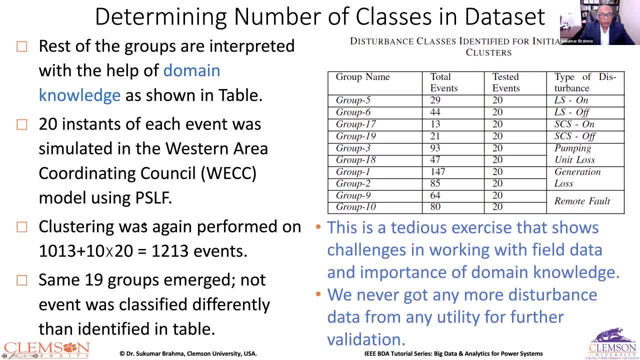 and ran the clustering algorithm again And it actually gave us what we had assumed was correct. So finally, we came down to all the unknowns that you saw: load switching on off, series capacitors switching on off, pumping, unit loss. These were synchronous motors. 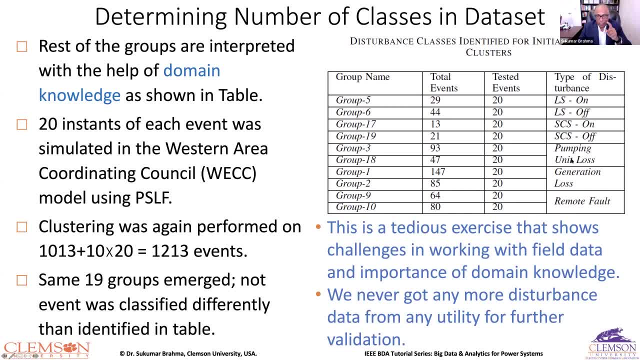 And that was, you know, typical for that system. They got lost And there was a generation loss. There's another two groups which were generation loss And there was one remote fault. Sometimes what happens is fault takes place away from the PMUs. 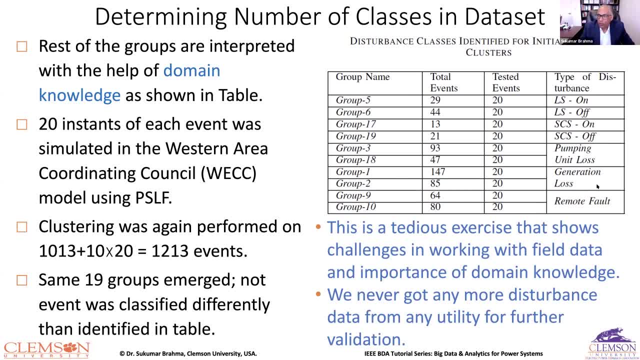 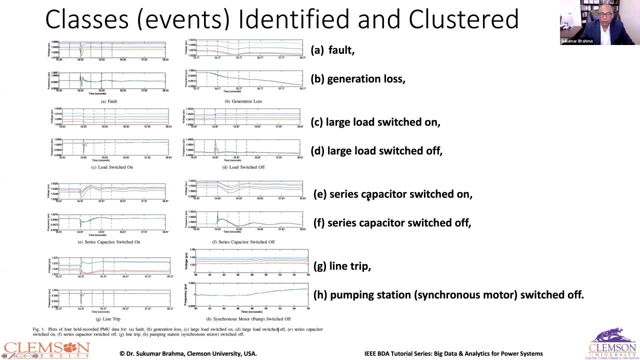 The PMU is still captured right. Same for generation loss. So then now we, if we put all these together right, we have our classes. So fault generation loss. switch on, switch off of load series capacitor. 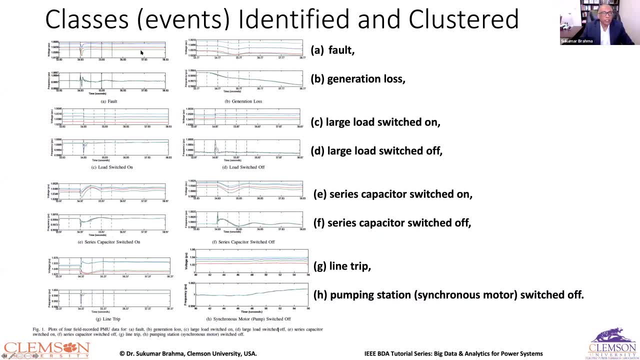 line trip and pumping station. These were, these are the typical signatures And if you look at this, these are faults: the voltage and frequency for fault for generation loss, for load switch on, load switch off. It will, for if you look at from, 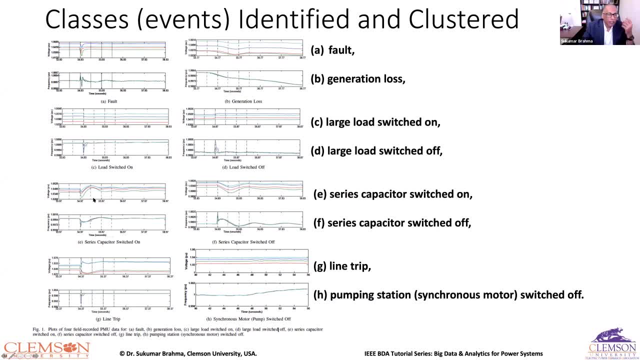 if you put your power system hat on, this is reasonable for for this type of event, You would expect to see these. So that's how we. that was the first step, to find out how many classes. Okay, Now let me show you a little bit of close up here. 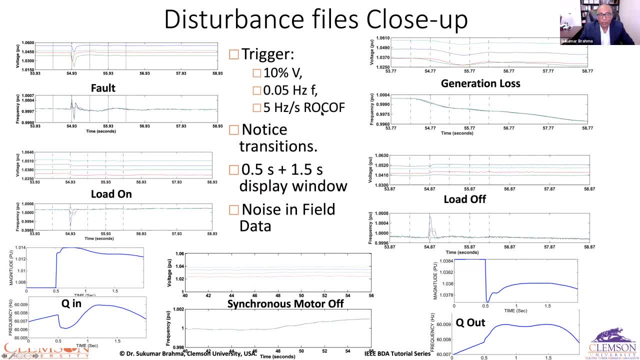 The trigger was set as of, you know, rate of change of frequency, frequency and voltage. So if you see the fault signature here, suddenly the voltage goes down Suddenly, the frequency jumps up and down, Whereas in generation loss it's pretty. 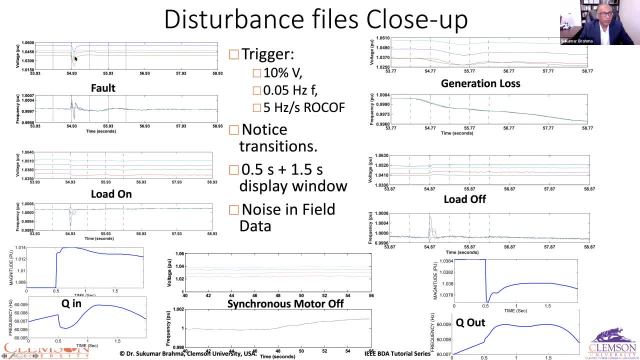 you know classic, It's not doing anything that quick. So these are very clearly separated. Load switch on. Now load switch on. if you look at this, the frequency is doing what you know, a quick jump, but the voltage 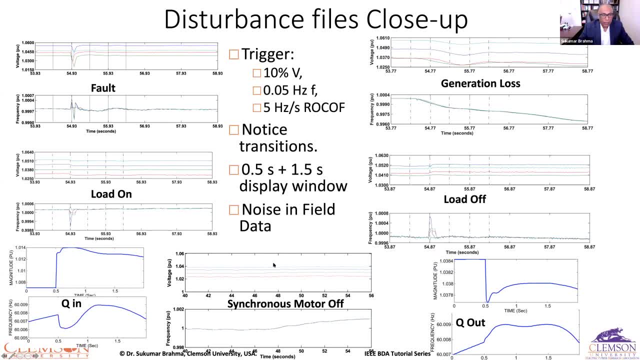 not so much. Same here, right, Synchronous motor, again very different signature, And then the this: we didn't actually have a field data, So we created this data for you know: capacitor in and out. So this tells you that, if you can actually see, 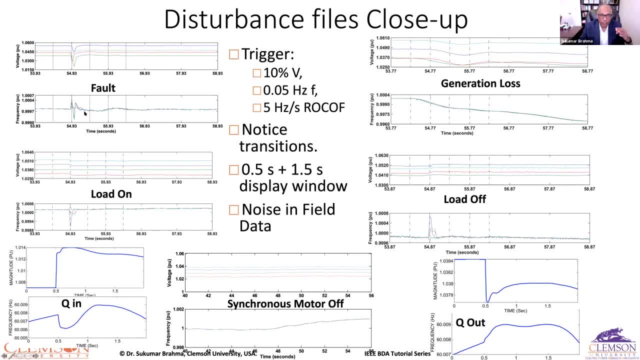 so this is where, again, the domain expertise of my computer science science colleague came in handy. She looked at this and she said: you know what The features are? the raw data has a lot of information here. So instead of using any domain transform, 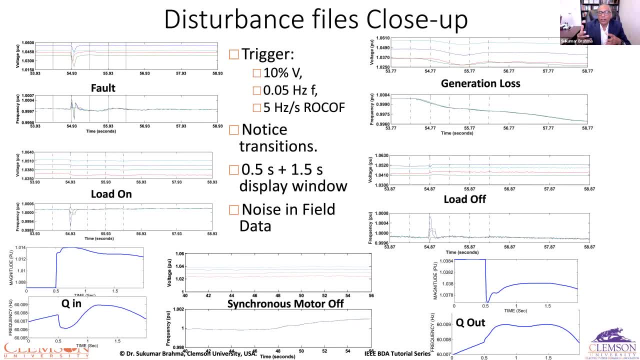 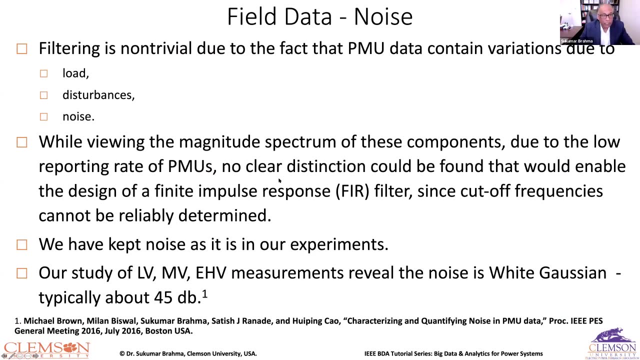 why not we use just the raw data or a method based on raw data, And that should do it. So she was recently. she had started working on shapelets and that's what she did. So in the interest of time there, yeah, 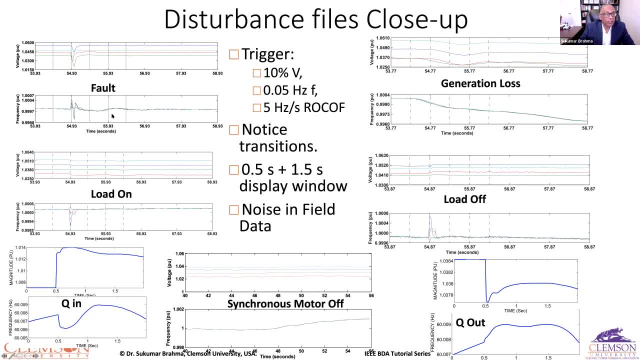 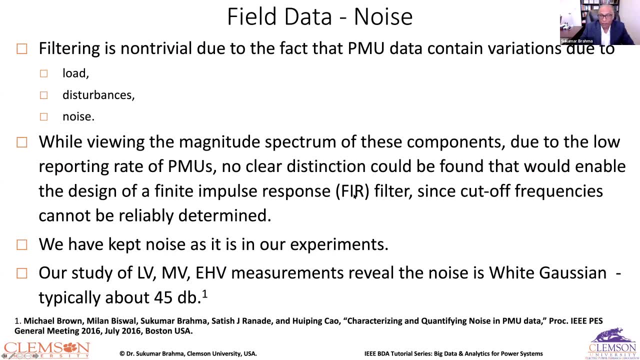 there was noise. So if you look at the data and you know that anybody has used PMU, it always has noise And this noise is not easy to filter. There's you cannot design an FIR filter for this, So we kept the noise as it is. 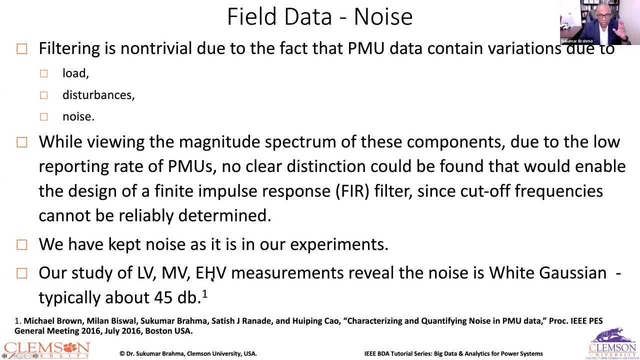 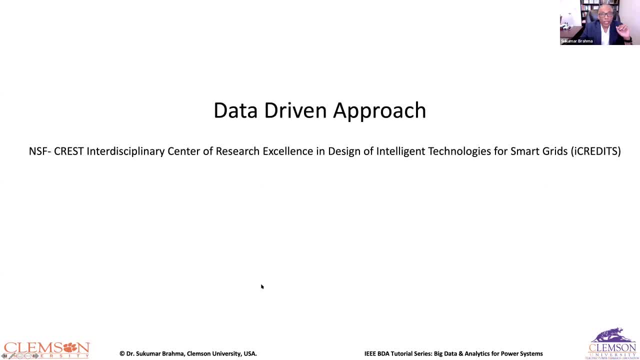 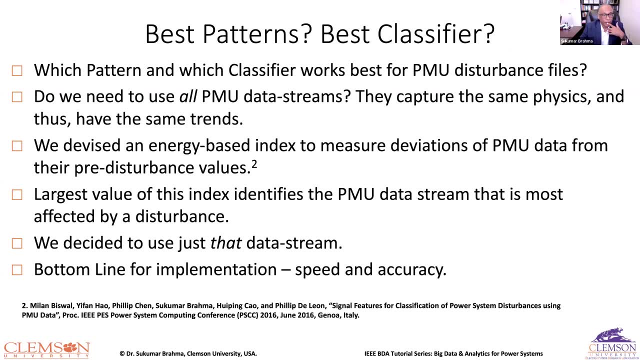 And we also studied the noise in all LV, MV and EHV measurements that we had from other projects, So about 45 dB. Okay, We kept it Data driven approach. So what pattern works the best And then what classifier works the best? 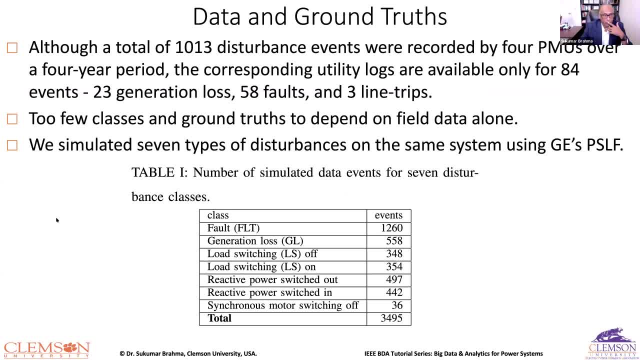 So again, if you wanted to build a classifier, you need ground truths. You had 23 generation loss, 58 volts and three line trips. Those were your ground truths. That is not enough. So now we simulated again the same PSLF model. 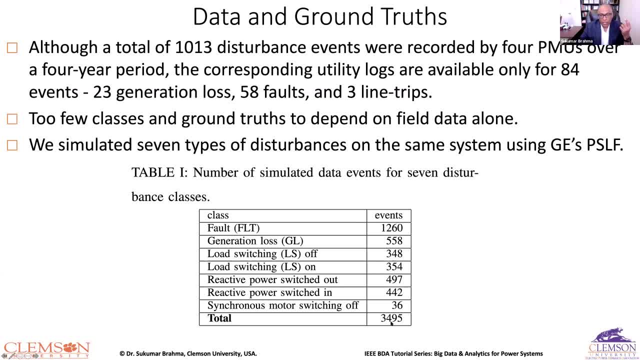 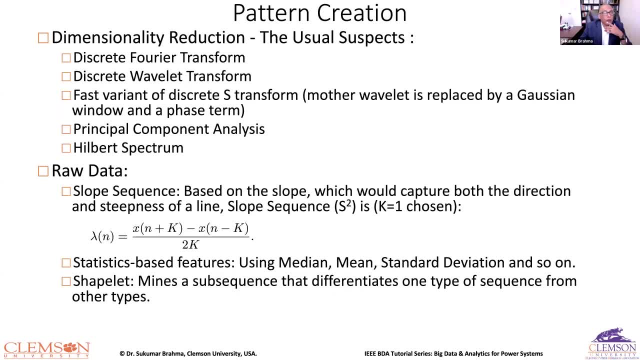 we simulated more faults, more generation loss, So we actually simulated a bunch of disturbances to include Now, since there are multiple people involved there. So we said, okay, let's do domain transform also. Fourier wavelet: There was a postdoc who was very 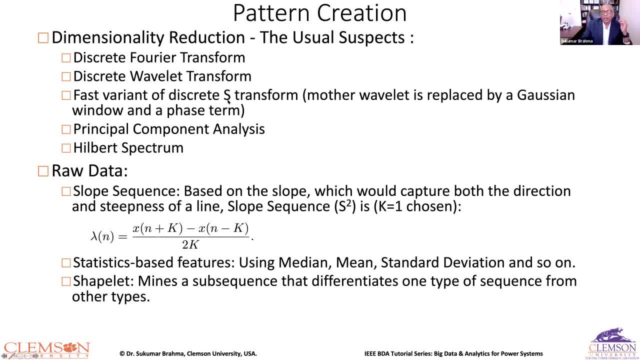 a big fan of S transform, which is basically a, you know a mother wave that is replaced by a Gaussian windows And there's a face down there: PCA, Hilbert, So you name it. like these are all heavyweights. 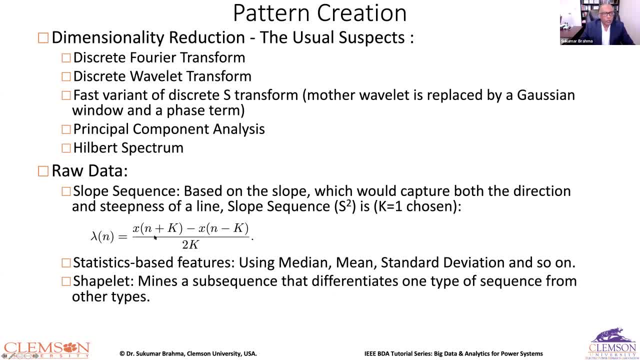 Then we said, okay, raw data, We just do the slope of raw data, statistical based features and then shapelet. So shapelet is basically a subsequence of. so what it does is it creates a subsequence of the time domain data. 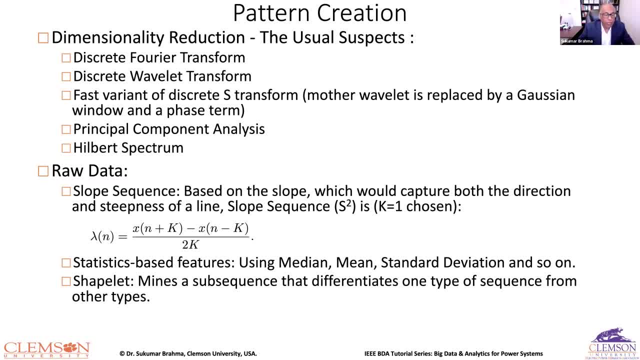 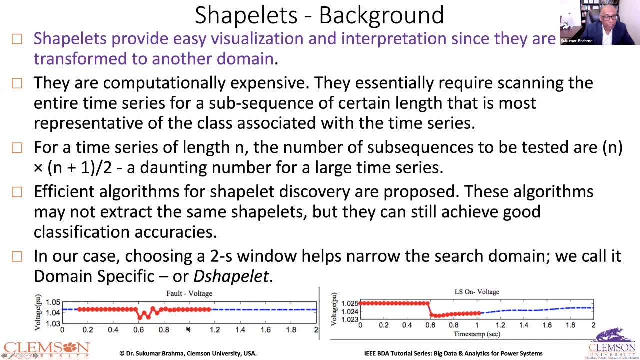 And how it does that. we probably skip that because we kind of getting near the one and a quarter hour mark here. But usually the shapelets are good but they are very computationally expensive because for a time series of length n, the subsequences to be tested are n times n plus one over two. 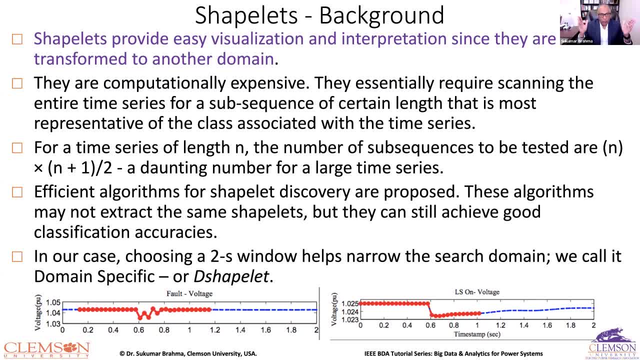 So if we had a three minute window but we shortened it to to a two second window, because that's where the disturbance signature was seen the most prominent. So because of that we called it domain specific shapelets or D shapelet. 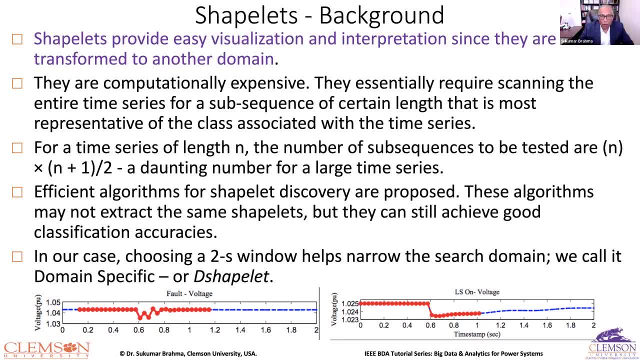 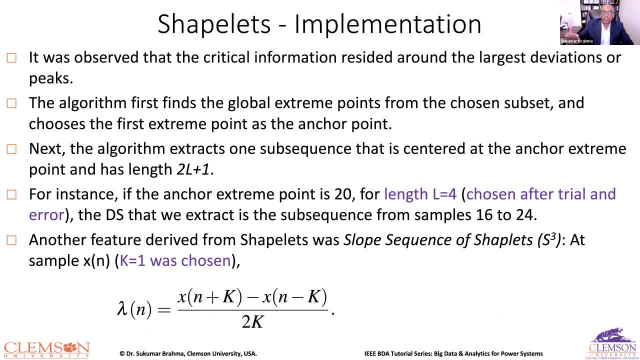 And that works. So that reduced the computation burden a lot. And we also created another feature. that was the slope of slope sequence of shapelets, which basically took a, you know, a slope across every point, Okay, Of the shapelet. 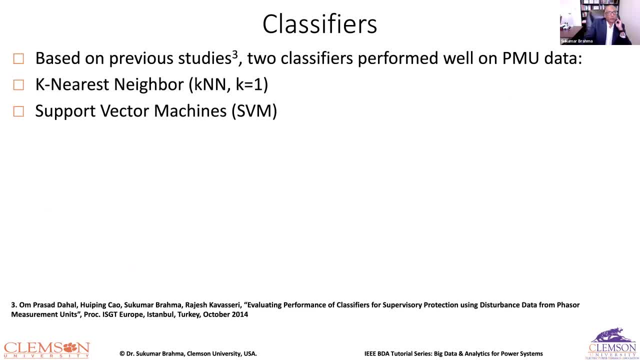 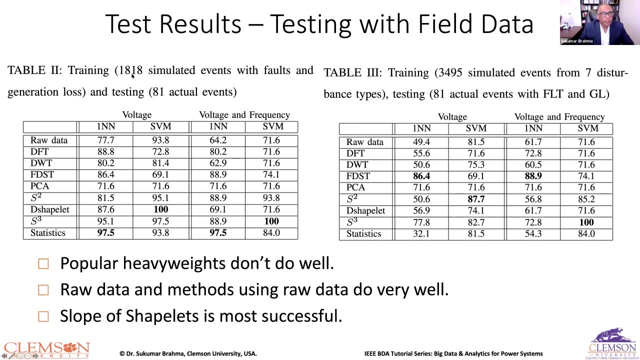 And then we tested. we had done some tests before and the KNN and support vector were were quite promising in that study, which is in this paper. So we did that. Okay, Let's look at the results. So what we did was all simulated faults and generation loss were used for training. 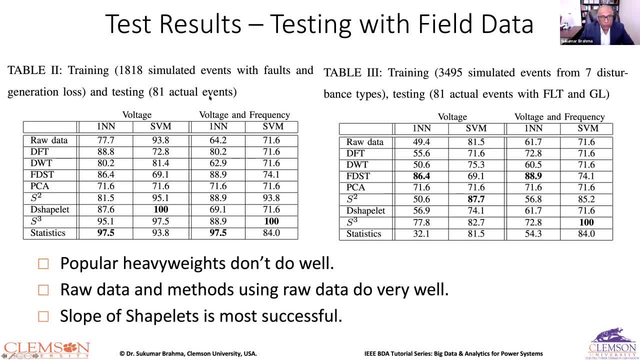 And the field data was test used for testing. Then here all seven disturbances- simulated disturbances were used for training, but for testing was done only for fault and generation loss. Look at how these perform. All these heavyweights are not really doing very well. 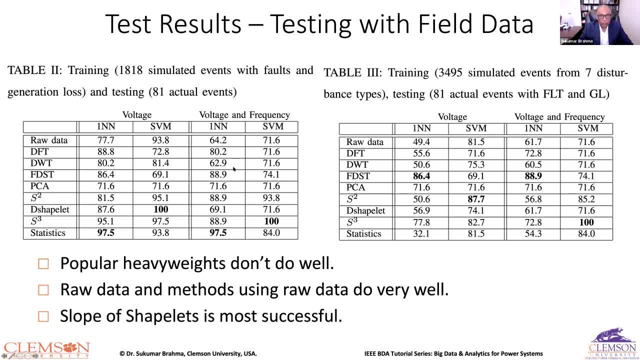 So we took voltage and also voltage and frequency, both Voltage and frequency, both is better. But if you look at raw data, raw data is 93, 95%. It's even better than some of the transforms. but the, the slope of C, the slope of shapelets, 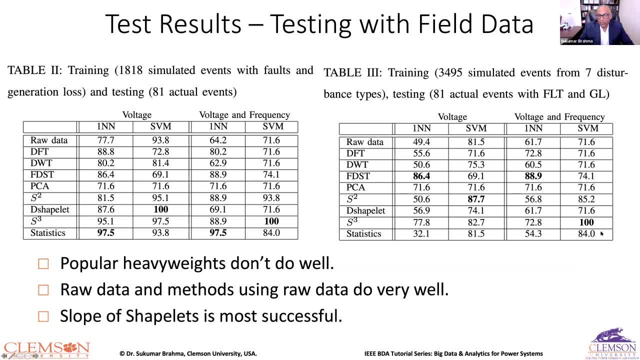 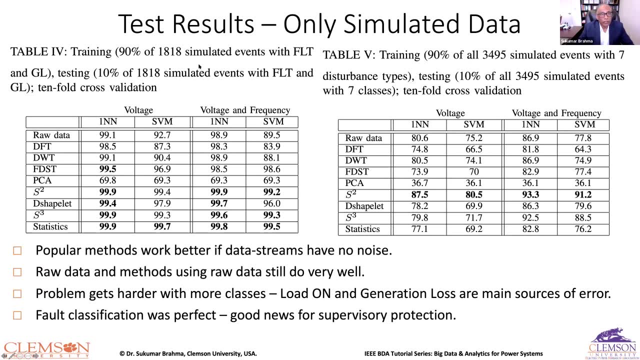 which is SQ, performs the best here. Also it performs the best right. Okay, So this was simulated data for tests, for training, field data for testing Then. then we took all simulated, So 90% of the simulated fault and generation loss. 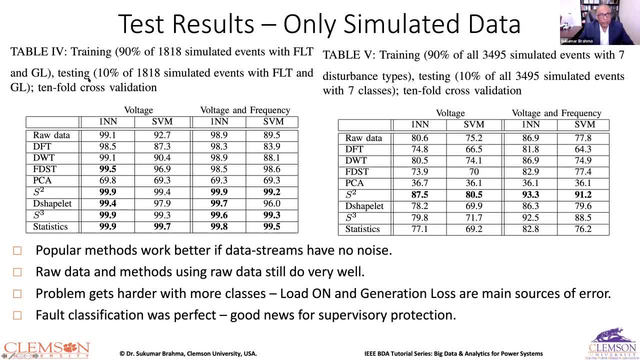 and then 10% were of that was used for testing. We did 10 fold clock cross validation. That means all the data that were used for training once was also used for testing 10 different times. Right, And now you can see that, because this is simulated data and it doesn't have noise- 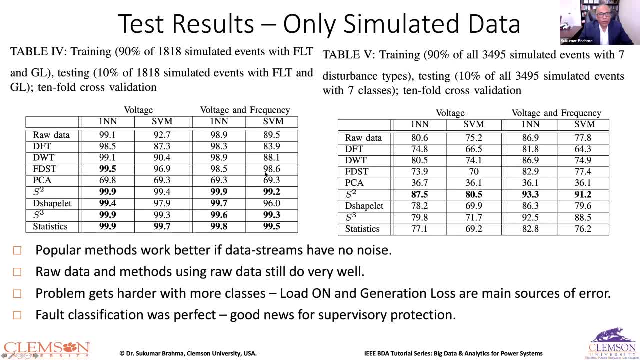 The. these methods start performing much better. These still perform well, but the other ones they perform better than before. here We are doing all simulated seven events And then the. we are testing it for seven classes, not just for fault and generation loss. 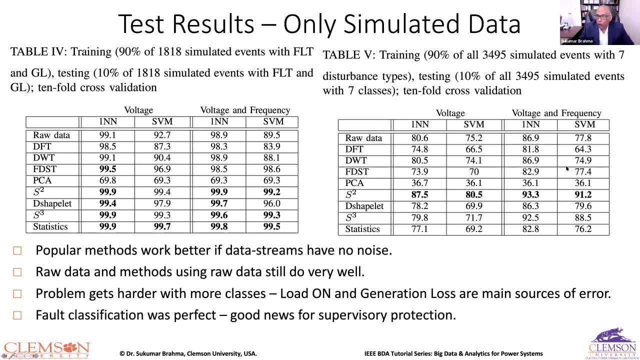 all seven. This is where the performance falls the most. If you can see here the, the methods that are giving almost a hundred percent, 99% of of performance drops to about 88%, And the best is here- 91%. 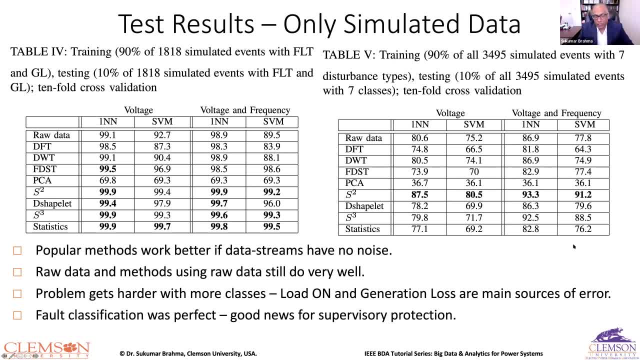 Why is this happening? Well, we looked at this and we saw that all the problems, all the misclassifications were happening in load switching off and generation switching on, or rather generation switching off and load switching on. So if you look at the physics, 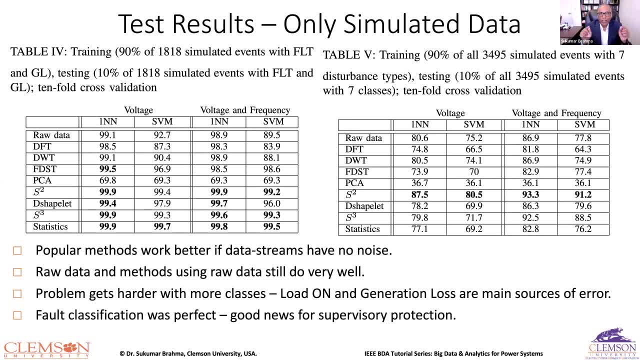 you exactly have the same physics right. A system loses the load or gains The generation is the same effect and vice versa is also the same effect. So load on and generation loss were the main sources of error, And that is why that's. 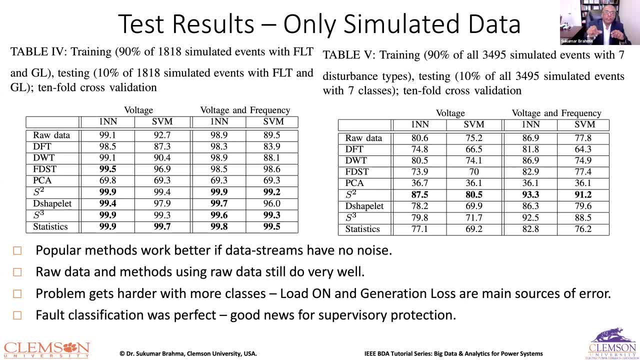 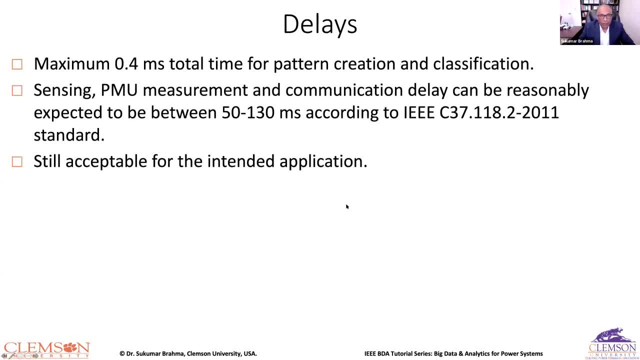 this is why it shows that you know now, if you use some physics based approach to this to help this out, this can get better, And that's what we did. I'll give you like two or three or four minutes. 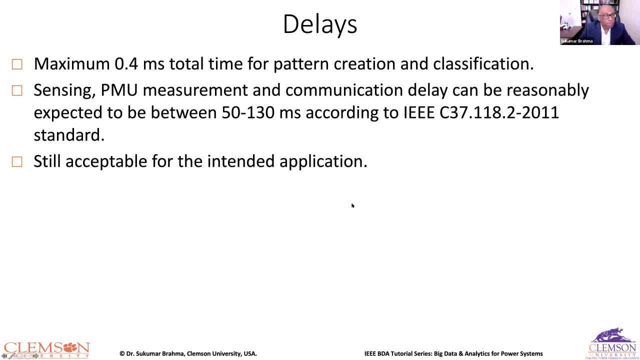 Uh, so it took about 0.4 milliseconds, of course, for for all this to to happen, which is fine, Uh, for, uh, you know misoperations, you have more time, Uh, and the fault classification was perfect. 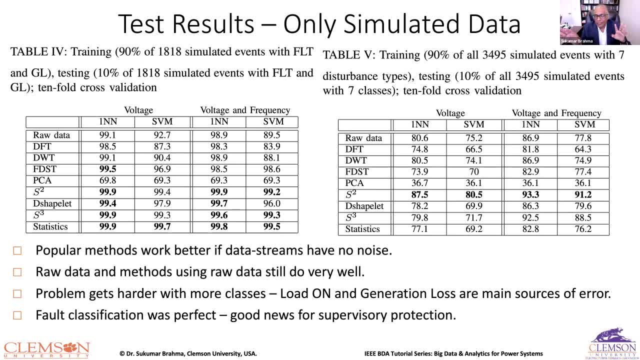 Okay, Even with uh, for any of these cases the fault classification was perfect. That's what we want for misoperations. So that is a good news for for what we call supervisory protection. Uh, and then we another. 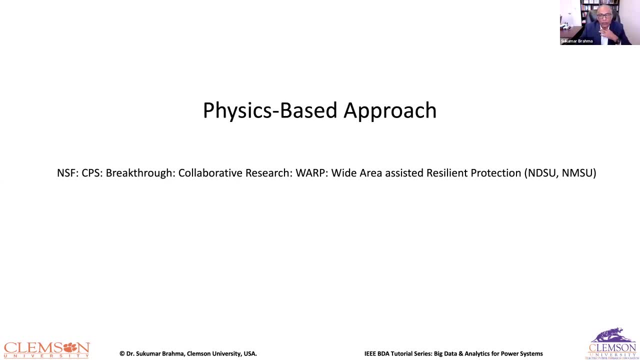 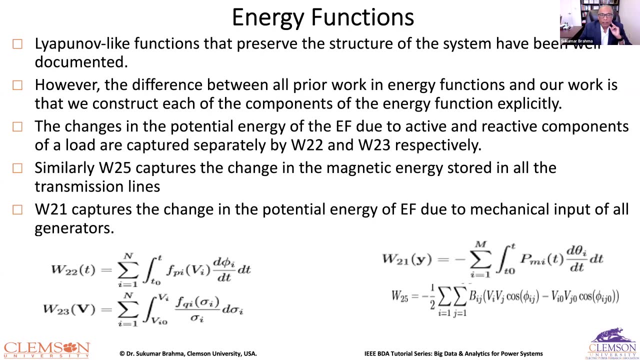 uh, uh. CPS, the NSF grant that we got was essentially using a physics based approach. We used energy functions. Uh, now, energy function, typically they, they've been used for a long time. Okay, You see papers on on energy functions. 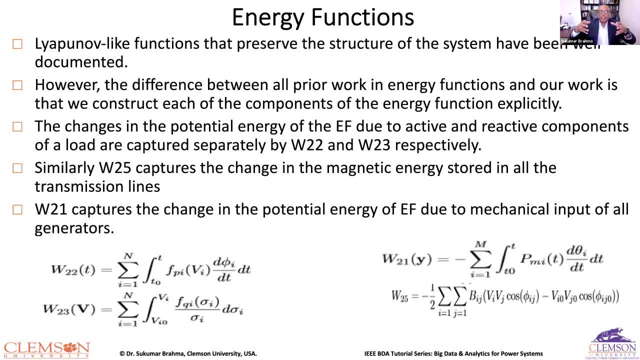 the seventies. but it is a big, humongous function. It captures all the energies of a power system. What we did was so that energy comes from generation, comes from load, comes from line. So this is what you know. this comes from gen. 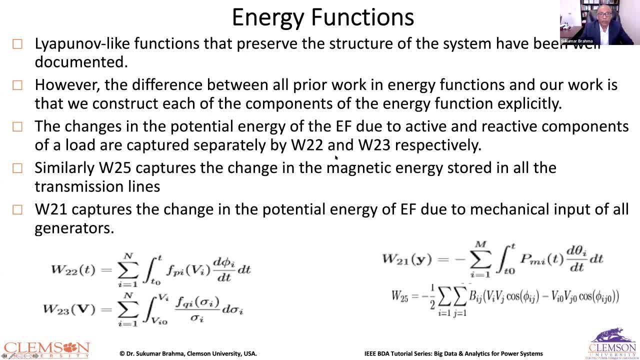 uh uh, these two uh w uh. two, two and two, three are uh uh representing loads to. five represents the line. energy to one represents the potential energy in the in the generator. These are the components. 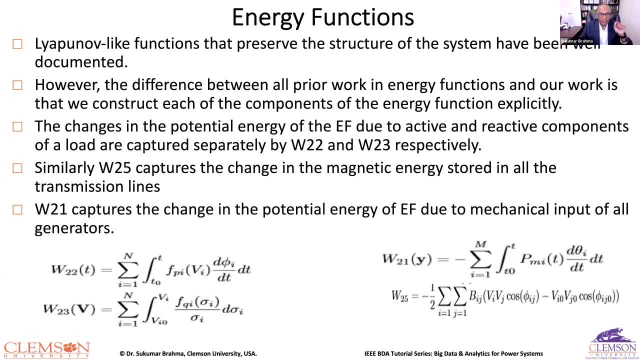 Of energy functions. So we said that if there is a fault, I would say the line from line energy function would be impacted the most. If the load changes, this is going to be impacted. If the generation changes, this is going to be impacted. 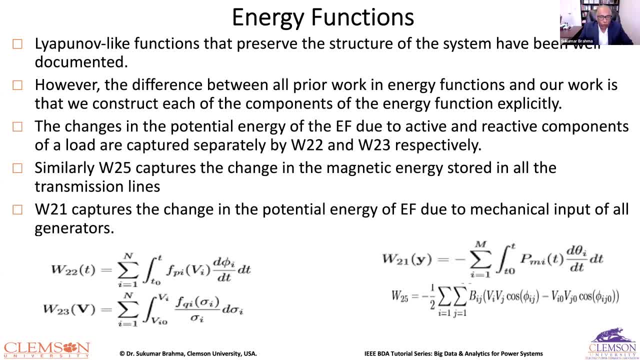 So the the problem we had between generation and the load, we resolved by using components of energy function, And we were our assumption was correct. If you look at this, the generation mechanical input changes the, the, the, the. 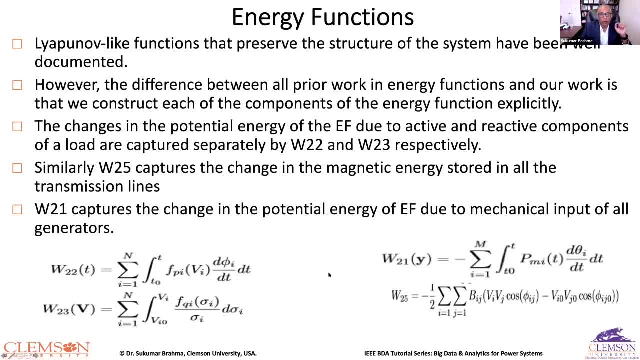 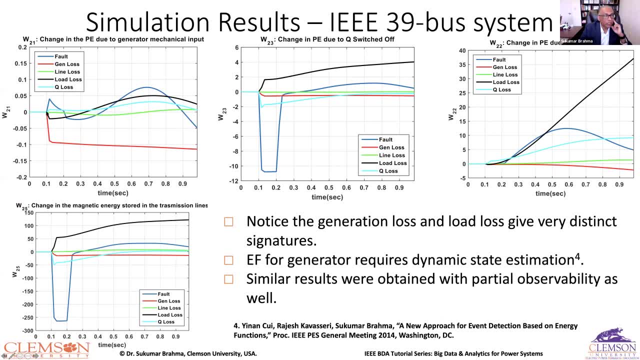 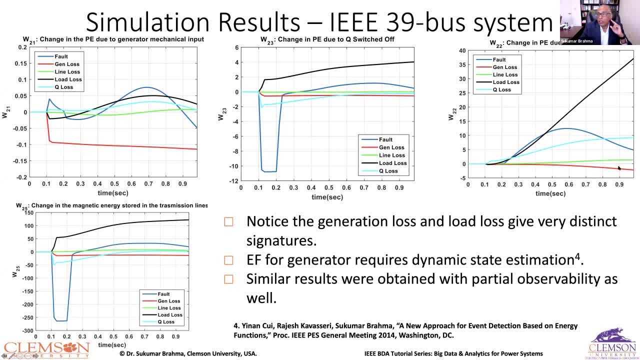 So this one changes the most for generation. But if you look at change in the load you hardly see that changing the load component, The load energy function, is changing perceptible here. So that problem between the generation loss and low generation and load. 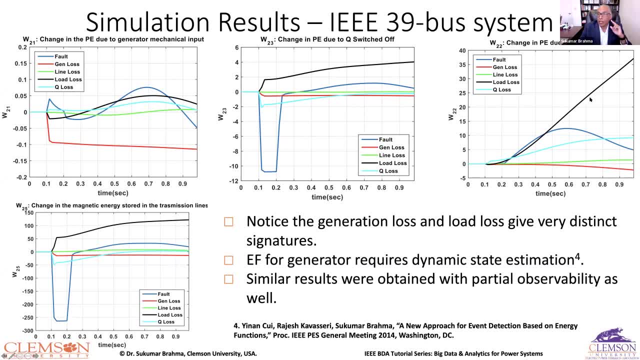 uh, uh events Boss is resolved Using physical attributes: The system. So so, uh, thehy the, uh, the, the, the the system. So I guess, in the interest of time- I think I'm probably- it's all that I needed to say. 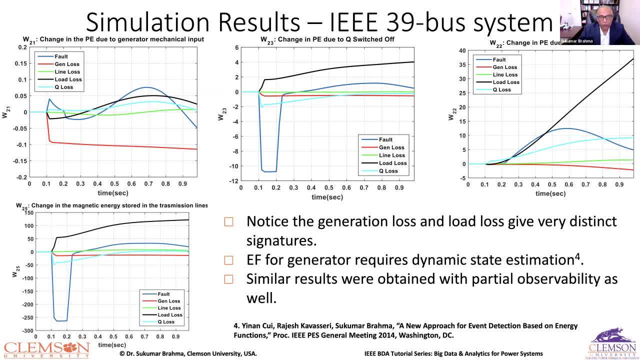 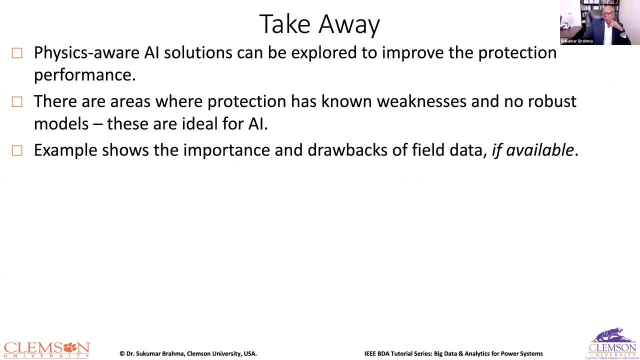 We could have gone into a little bit of detail of this, but that's okay, You got all the papers there in case you're interested. So then you know physics, aware AI solutions. So make you know AI and physics. if they are friends with each other, we can go a long way. And 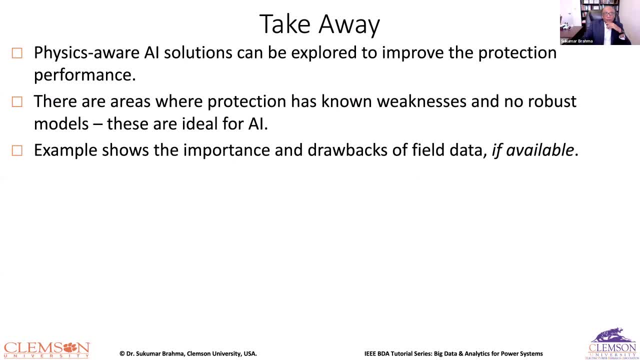 there are some problems that the protection engineers have not been able to deal with efficiently. where AI can be helpful, right, And then the example essentially showed how much of a. you know how difficult it is to first get the data disturbance data. 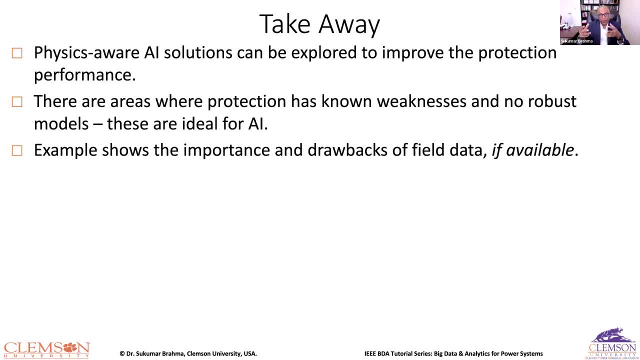 If you get using it is it takes. it's challenging right Now. we wanted to take these results and validate it with another set of data from another set of PMUs. Nobody gave us that data. Okay, All my friends at different utilities, different ISOs, they were all okay with it. But when it got to,